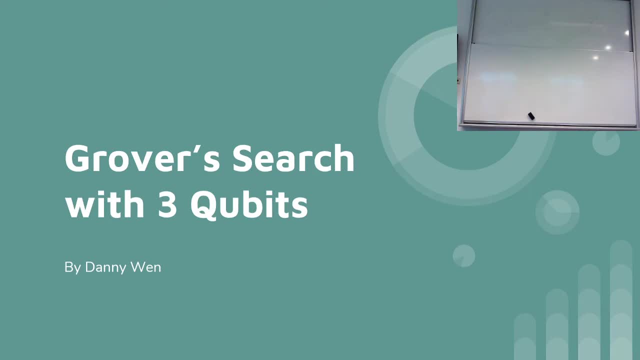 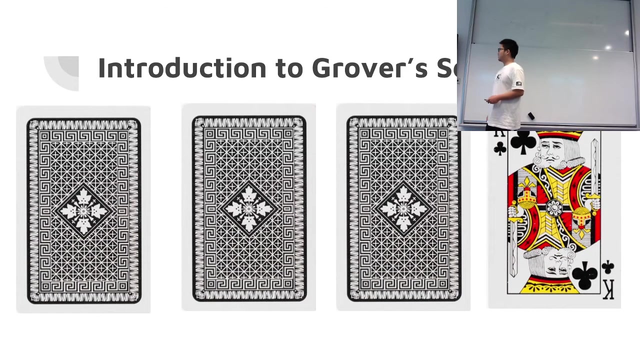 Do I need to push this? No, The other way All right. All right, yes, So I need to open this? No, no, no, This just needs to be in the foreground. Okay, thank you. So first let me ask you a question. 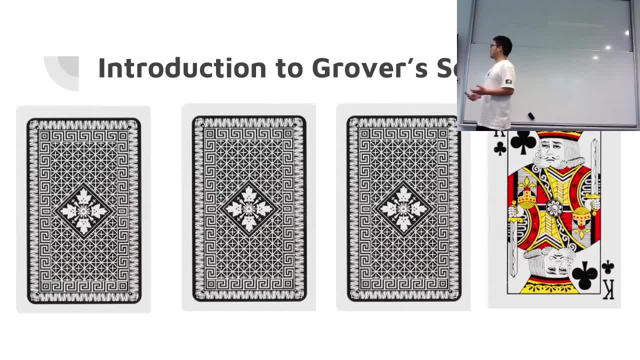 If you want to find one card inside four cards and you only have one chance, what are the odds of locating that card? Can you give an answer? What does that mean? I think it would be quite easy to open it. You need to find the K in between the four cards. 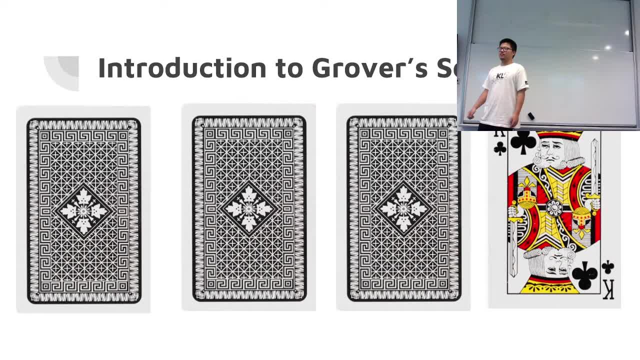 Yes, I would have one card which is the king. I would be hiding four cards. and then what are the odds of finding this card with my first try? I can't think of a method. There would be only one king in these four cards, and then you want to find it. 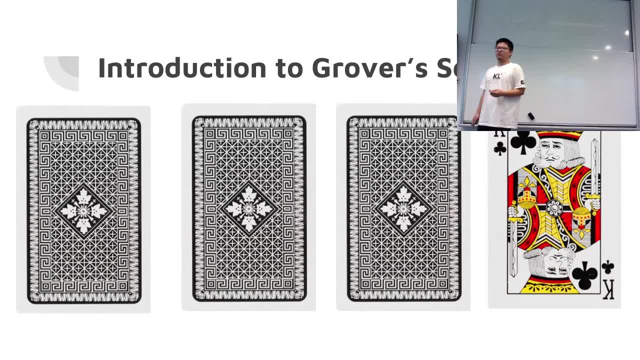 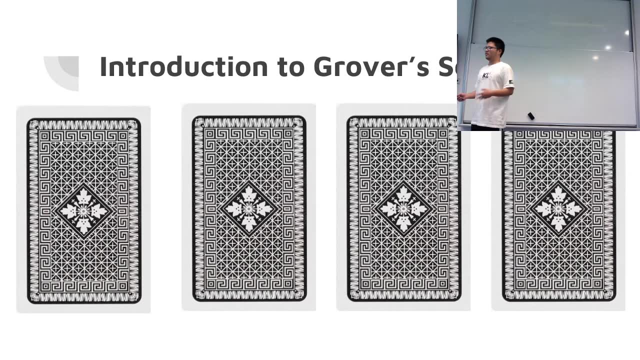 And it's like drawing a random card from four. Yeah, but it only has like 25%- Yes, 25%- chance of finding this king within the four cards. So what if I told you if I were to hit these cards and I were to find the king? 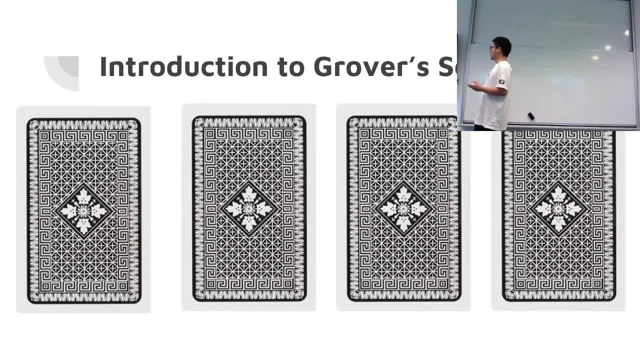 I would only use one chance and then I would get the king 100% at a time. That sounds a little bit amazing, right, Yeah, Okay, so that's basically what our Google search does. It's a little bit complicated than just drawing a card. 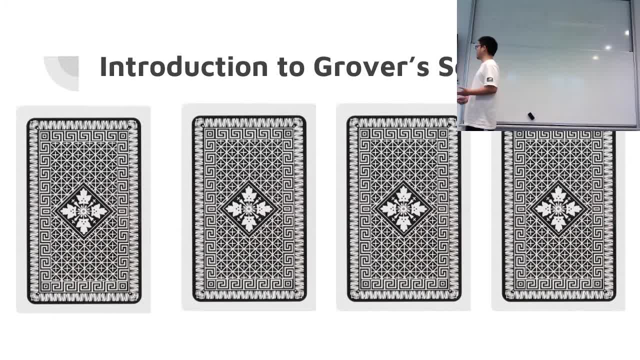 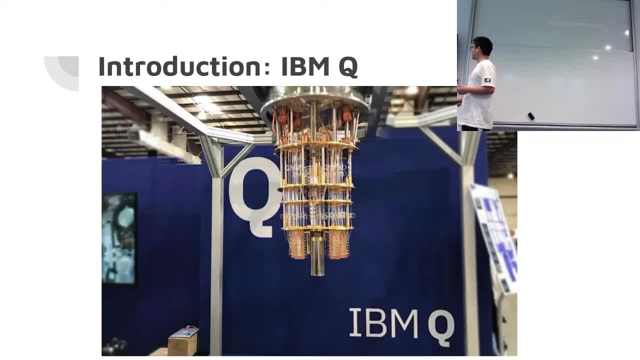 It involves some calculation in a way, but the basic idea is kind of like that. Okay, so the platform I'm using is IBM Q, which Professor introduced this platform to us, And it's like an online quantum computer which allows users from all over the world to use a real quantum computer through the Internet. 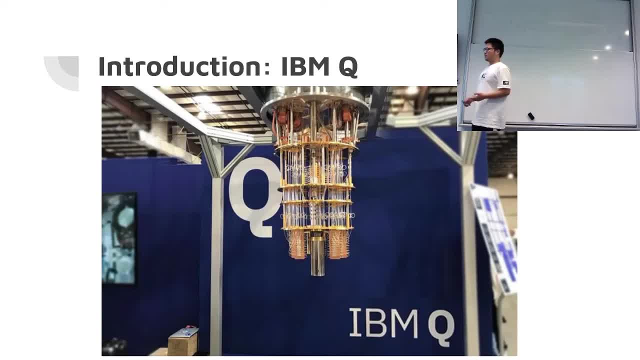 And actually some of the like. some data this platform provides is actually not like real-time operation on a quantum computer. It's kind of like if your circuit is already built, they will give you the data that was stored in their database, But the data is actually run through by a quantum computer. 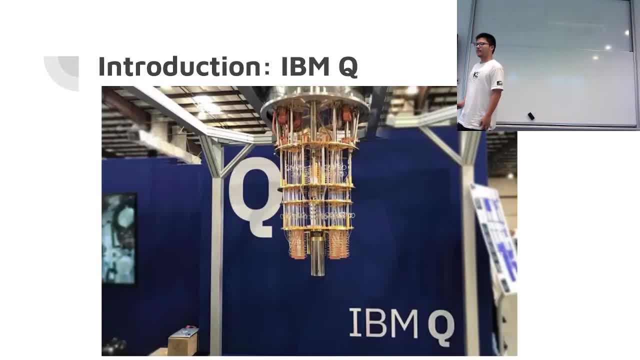 So if there's an algorithm that's single, it just gives you the data for that? Yeah, to my understanding, it's Yeah, because it's always like the same result and there's no fluctuation. so I Oh, okay. 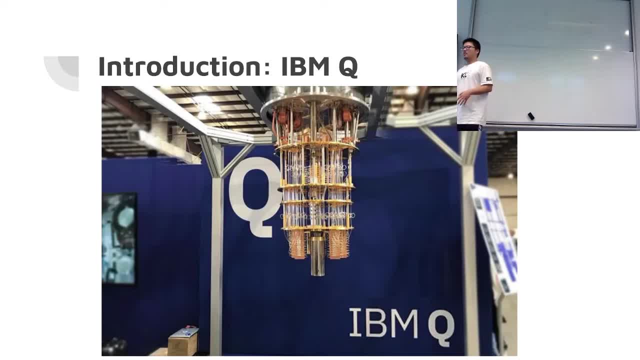 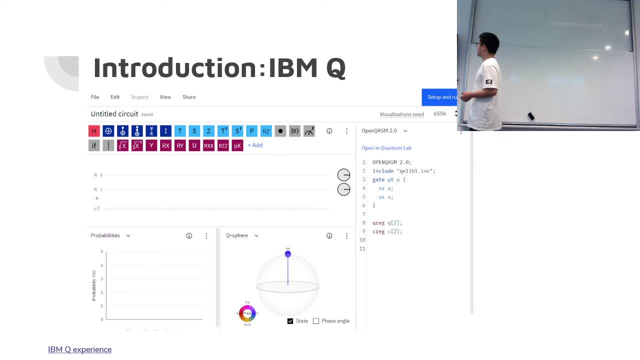 So only if you give it a brand new algorithm will it actually go and calculate. Yeah, it's like. So. this is basically the interface of IBM Q. Here you get some. Oh, this is a composter. I usually use a composter. 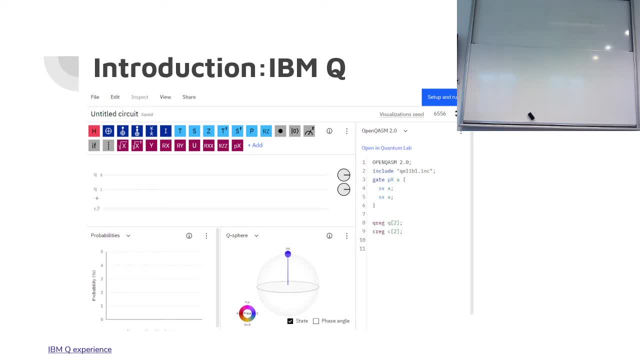 This is some quantum base that you can use to build your circuit. And here is these qubits that you can add and delete. I think you can add up to eight qubits, but I never use, Or more, or even more, but I never use that much. 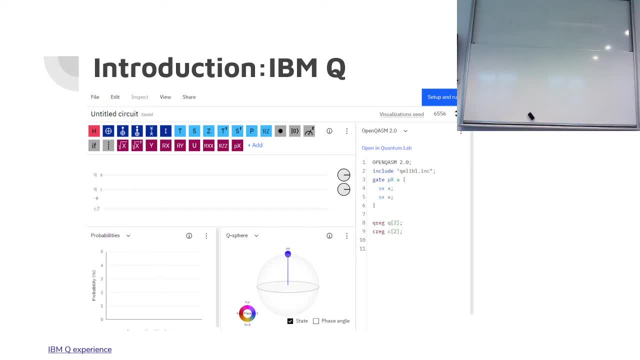 And here under this bar is, I think, which is what is the most important part of this quantum computer. It shows the results in very clear shape. One is the probability, The other is the block sphere state, And over here is the. 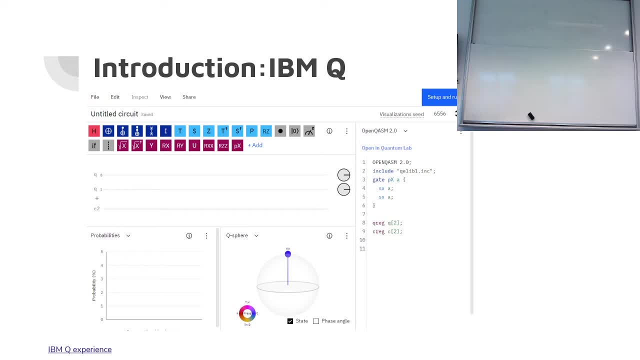 I think it's the coding part. I never used this part in my coding because this is the same as dragging gates and putting your circuit together with these quantum gates And in order to code, you need to understand like what is the code for each gate. 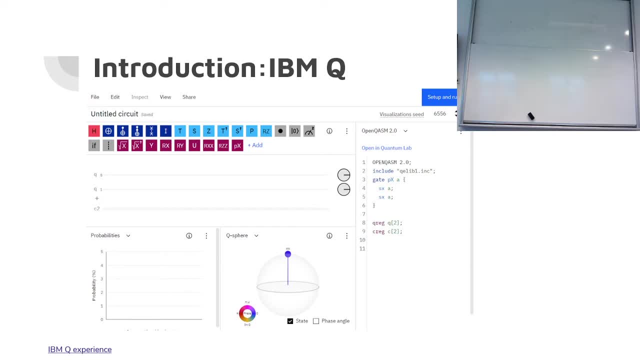 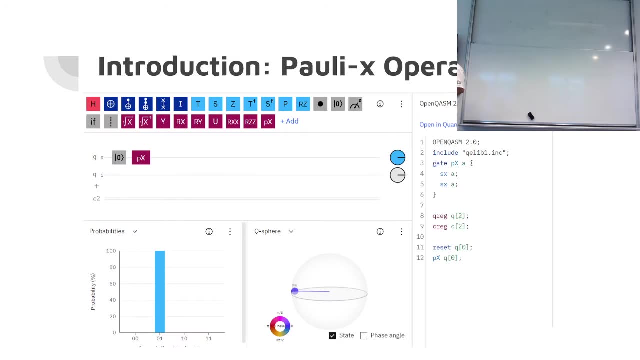 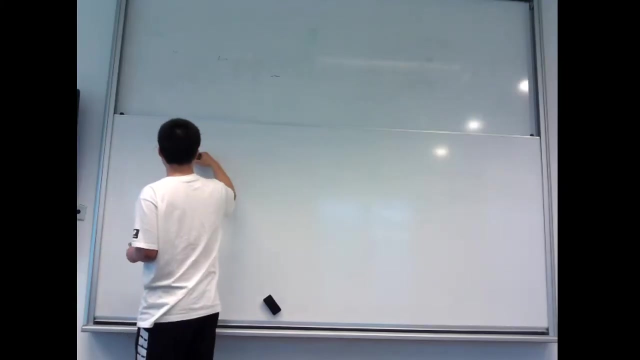 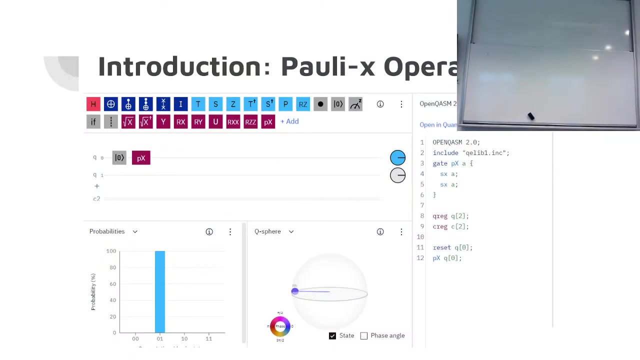 So to me it's more simpler using, like dragging, those gates. So in my quantum circuit I use a polyX operator which is simply this matrix- I think it's actually equal to the Not matrix here- which is this: 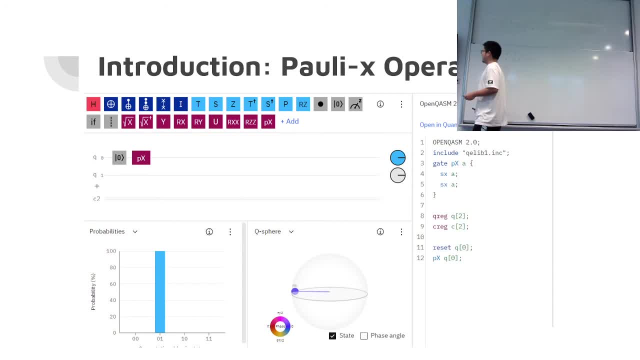 But at the time I did it I wasn't. I didn't fully comprehend this quantum gate. so I ended up grouping two, grouping two squared X together to make a polyX operator and use them in my circuit. So you defined that yourself. 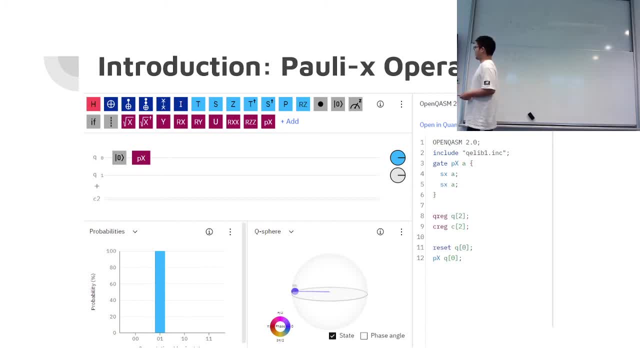 Yes, I grouped them together and defined it myself. Yeah, And from here we can see that, starting with the qubit at the zero state, after the polyX operator we get a qubit in the zero-one state And for that Q sphere. 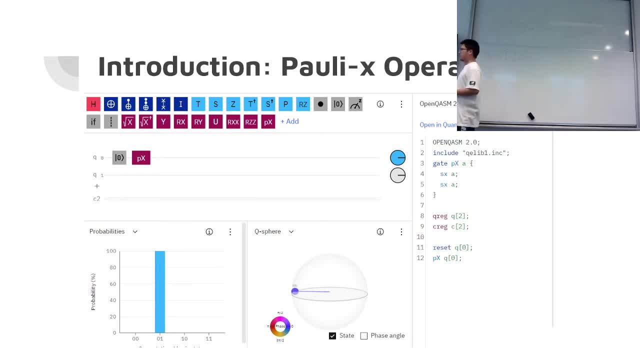 which I guess is the block sphere. how do you change which qubit you are looking at? Um, How do you do that? Yeah, I think you can drag it around and Because, like that one, I guess, is for the first qubit, right. 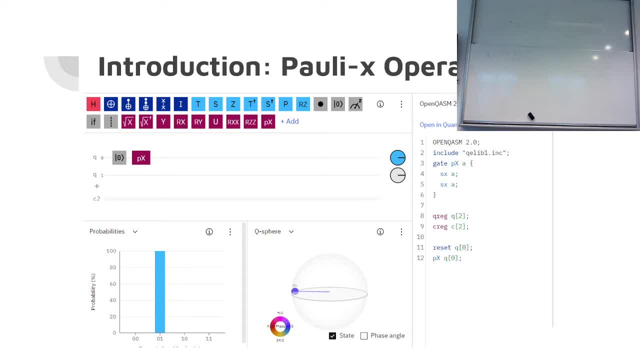 And this is: you've got two qubits, and the other one is always in zero right, In zero position. this is the zero-one position. Oh, oh, so that's the whole. Oh, okay, okay, so they must. 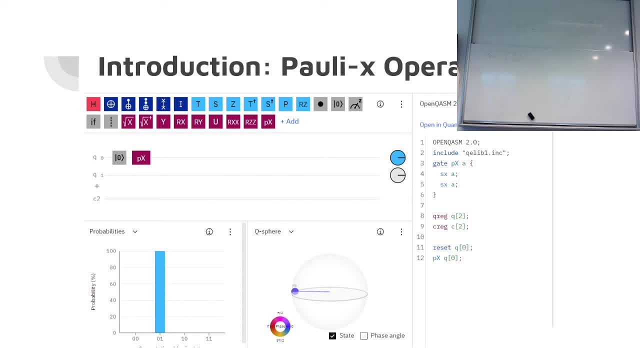 I guess they're using a more generalized block sphere, right? Because, Yeah, when we did the block sphere, You know our block sphere, Just for one qubit, Just for one qubit. yeah, This is actually for more than one qubit. 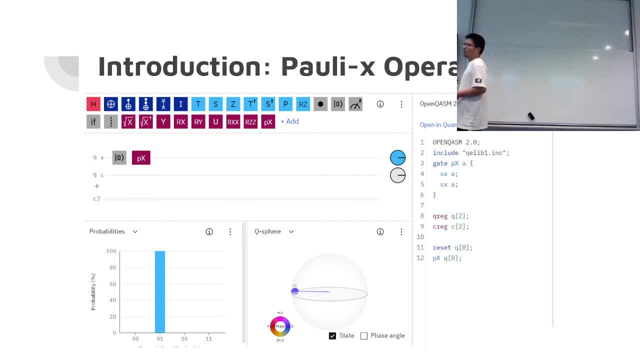 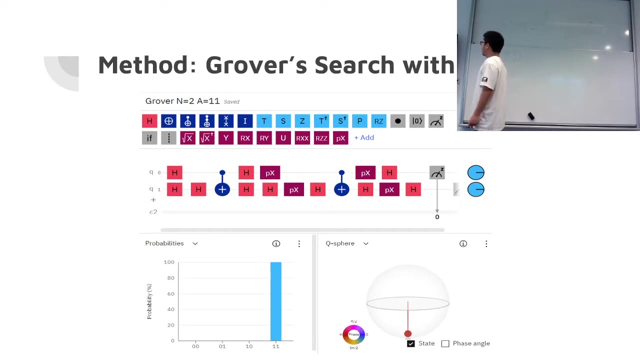 Yeah, I think they even have a block, This sphere, for three qubits or four qubits or even more, And they have different, like different, positions on this sphere. I see As an indicator. So, So Like, my goal is first to break down the 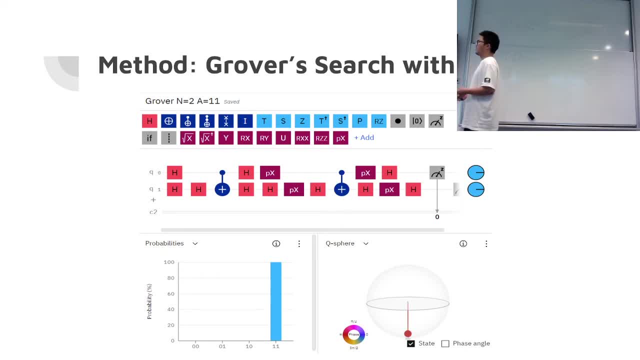 This goes. Their goal is to search with two qubit and like apply their similar methods to a three qubit case. So this is actually a circuit for the two qubit case And this is not what like the. This is not what the 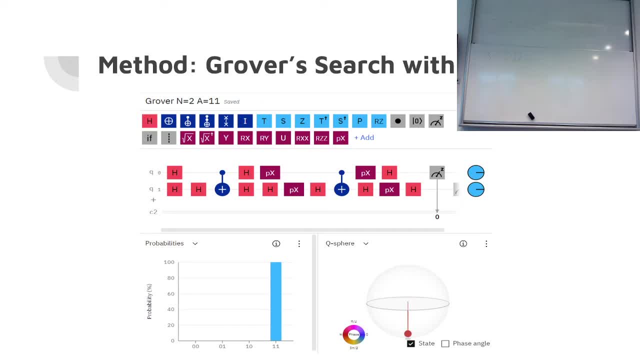 My Q instruction, provided I use my own operator, functions just like the Hottkey, and I will explain the circuit and how it's built, and so we can apply this method for the three qubit case. So here we are trying. 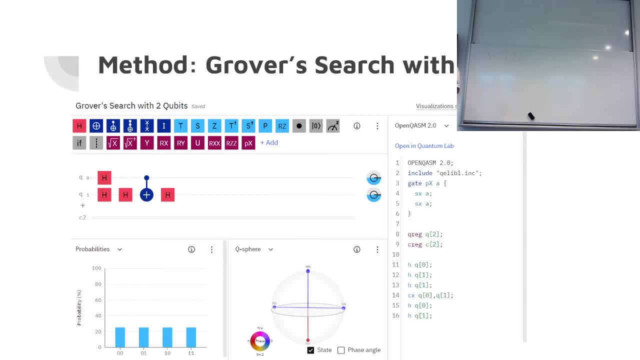 What we are trying to do is basically like putting the king into these four cards, So we first need to put some information into this circuit, and then we can try to use our global search to locate this piece of information. So what I'm doing here is creating a superposition using the Hadamard gate. 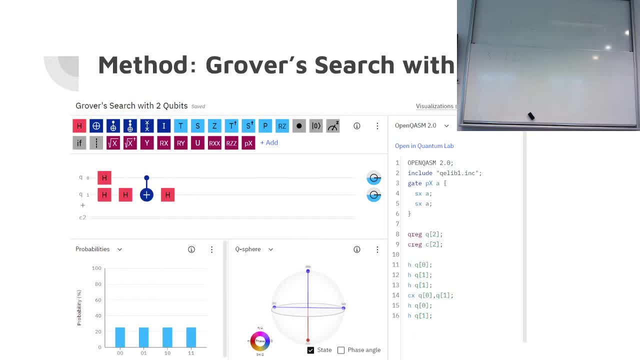 and then I'm using another Hadamard gate and the CNOT gate and another Hadamard gate to encode this message into these two qubits. So you can see from the end result the probability of them is actually the same. 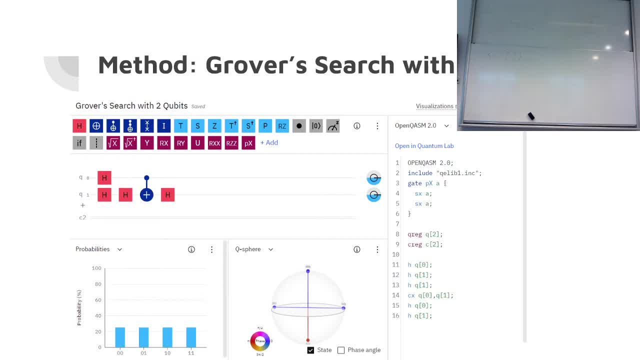 but what this operator does is that it has its information embedded in the last qubit. So that's the oracle, right? Yeah, that's the oracle. Hadamard, control node Hadamard: all that together is the oracle. 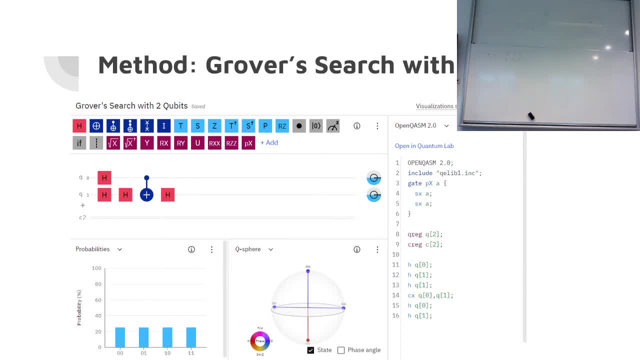 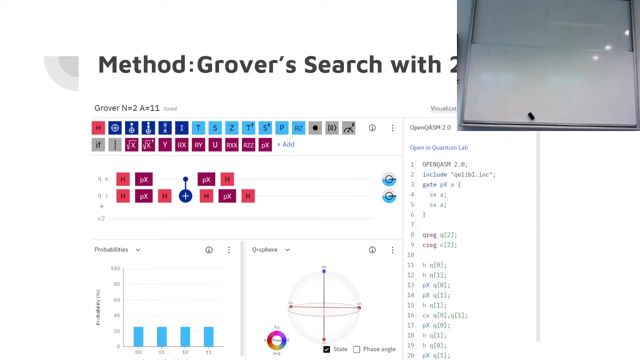 Yeah, so this part is the oracle. The superposition is just making it into the starting point And after, But after the oracle, I think this circuit is actually. I think this circuit is actually not the correct case, because we shouldn't have these polyX operators here. 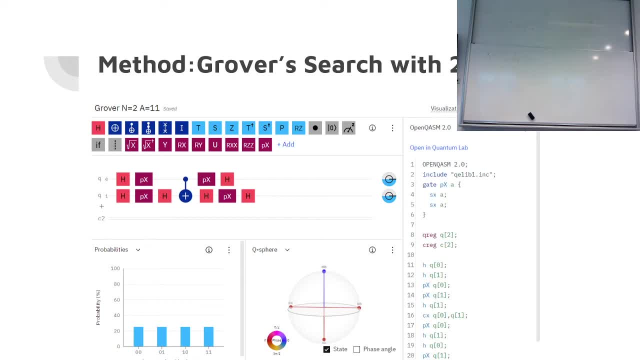 and the polyX operator should be over here. Yeah, those Xs will actually do nothing because, Yeah, The Hadamard gate is Yeah, Yeah, It's the eigenstate, so it'll just add a phase. so actually they'll do nothing here. 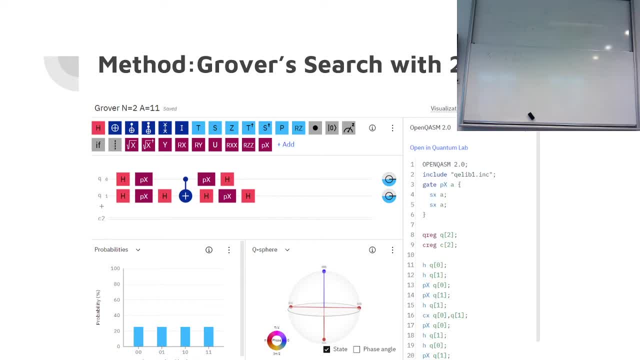 Oh yeah, so Is it safe? Yeah, it could be deleted. It's better to delete it. And so here we are, actually using these two operators to find the state, And what this polyX operator and Hadamard gate does is. 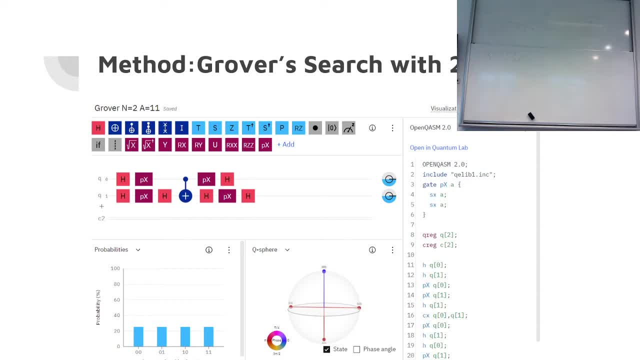 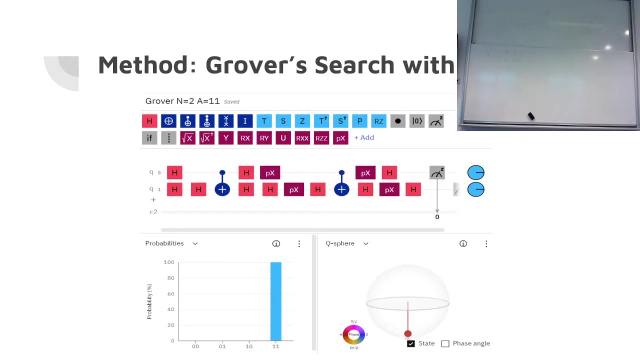 I guess it first changes, flips, the two states of the Q0 qubit, and then applying a superposition, And after that with some, And after that with another Hadamard gate and a CNOT gate. so this is: 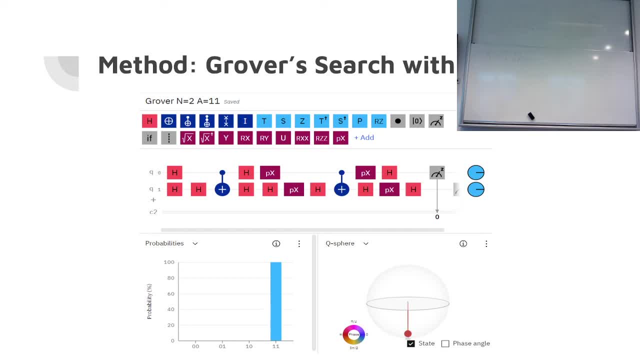 You can consider this as a hole. So this part is actually the Grover search algorithm And So the second stuff, all that stuff, is the thing that flips the sign on the 00, on the plus-plus state, that other operator. 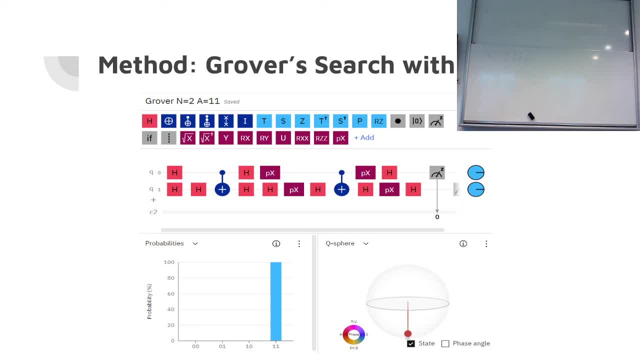 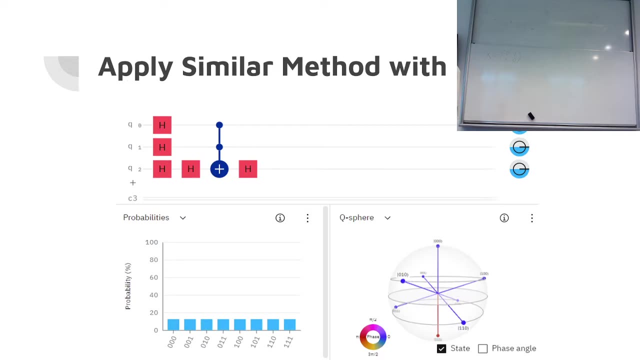 Yes, Yeah, Yeah. so that's actually the only function part here which does the work with this part, So we try to apply a similar method to the three-qubit states and Hold on. So did it work? The two-qubit? 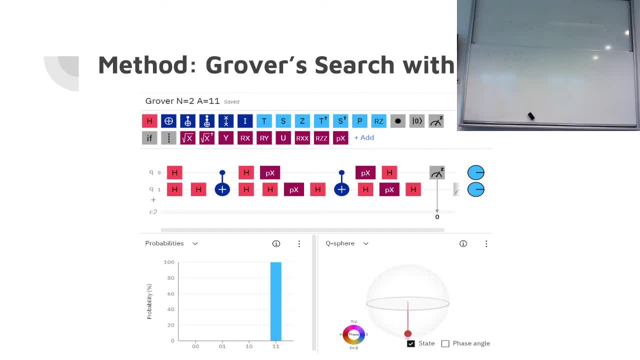 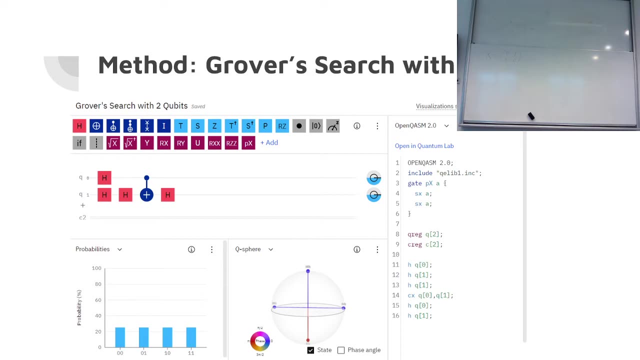 Yeah, Yes. the two-qubit state here is: Oh, I'm sorry, I skipped the result part. So here we can see we've hidden the information into one of these states and from this operator we know it's the 11 state. 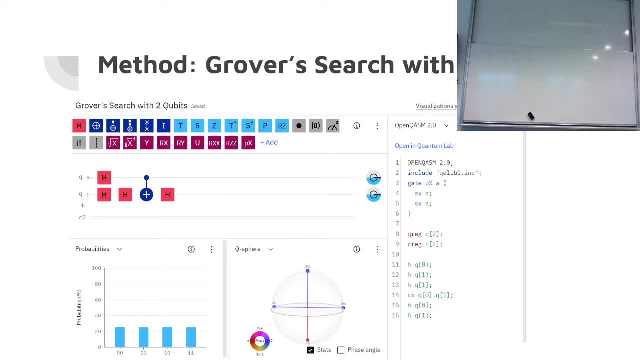 You can actually hide it in either state. For example, if you change this, If you change this to, I think, a NOT state here and a control state here, it will be hidden in the 00 state. So from the Grover search, 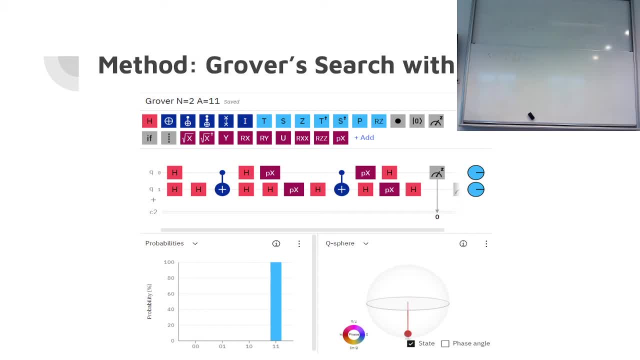 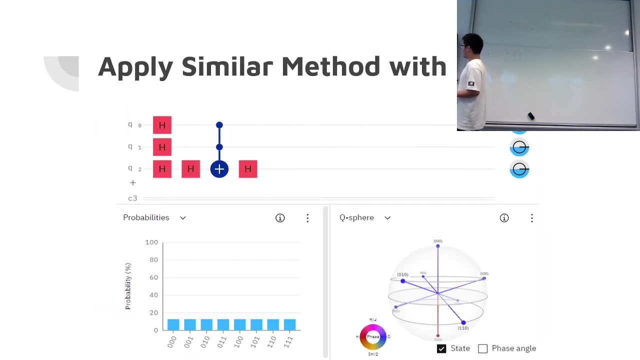 we can find the probability, which is The probability is one in the 11 state, So the information is hidden in the 11 state here. So in the case of three-qubits, we are again creating a superposition with the Hanmer gate. 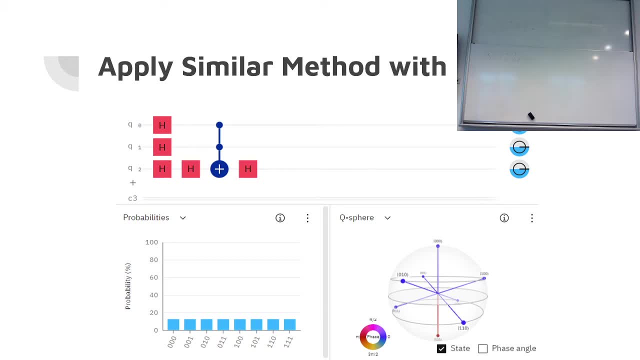 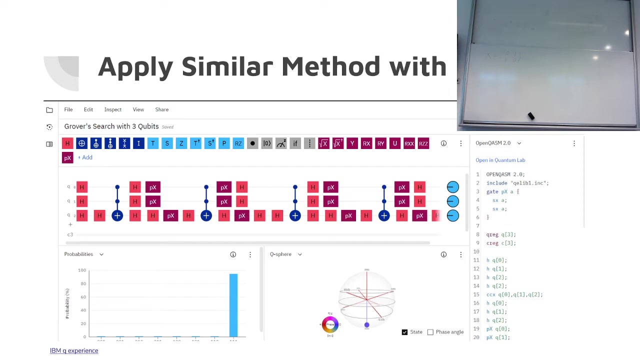 and then hiding the, hiding the information on the 111 state with a Hanmer gate and a Toffoli- I think it's pronounced Toffoli gate, And then another Hanmer gate And this is the. This is the full circuit for Grover search in the three-qubit case. 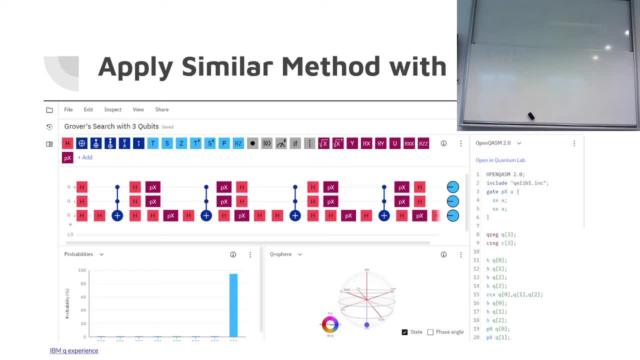 And this is the oracle here which hides the information. And this part here- the remaining part is the- is the circuit which does the actual search And it's very similar to the two-qubit case And we use We use the Hanmer gate and the PolyX operator. 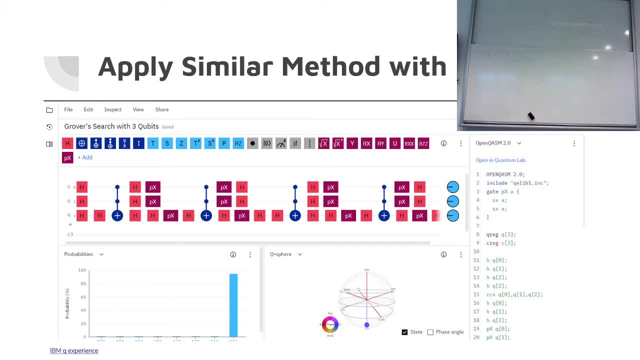 to first to create a superposition to. I think in I hear it's actually reducing the superposition and then changing the and then slinking the two states within each qubit, And then we use the, the Hanmer gate and the. 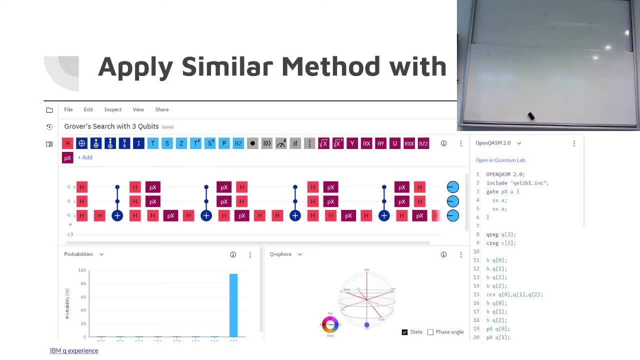 Hanmer gate and the Toffoli gate to, to pass the information to the to the last qubit And after these steps we can. we can get the result that the- the probability is- is actually all in the 111 state. 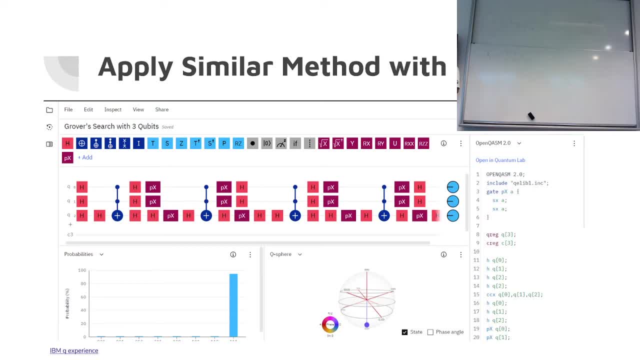 Yeah, so it looks actually like the Hadamard. and then three Xs. This looks like the thing which. This is the thing that puts the phase on the zero state. So remember, like from when I was: Oh, we haven't done the lecture yet. 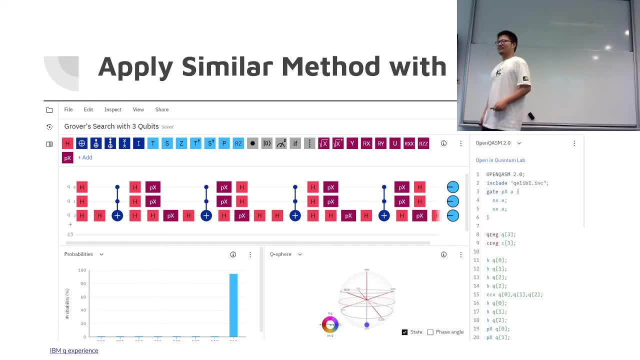 Okay, But the Like in Grover's algorithm there's, like You do Oracle and then you do the other thing which puts the phase on the zero, zero, zero state, And then you keep on repeating those two And then so it looks like the H. 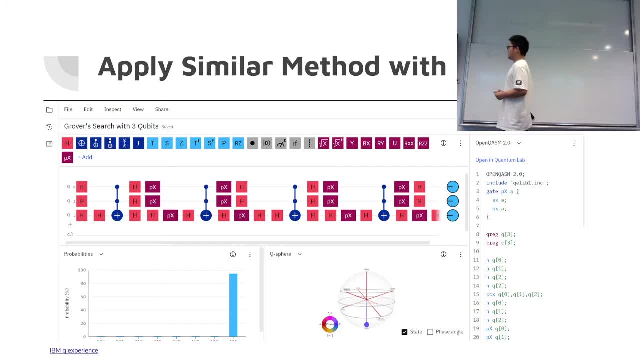 Three Hs and the three Xs is the is the other gate. Is that? Yeah, yeah, That's. That's, That's what I, That's what the circuit is about there, But like the way, The way, this. 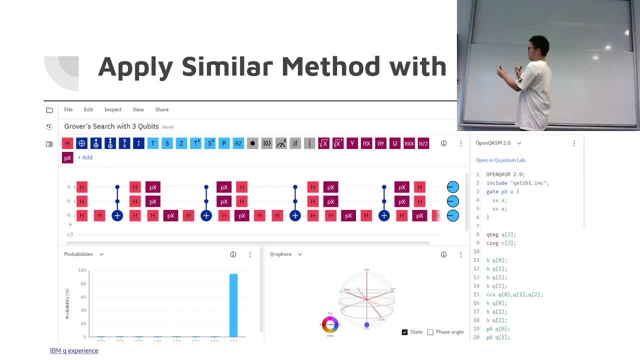 I mean Q is constructed. I couldn't like separate these two, These two, The Oracle and the state, clearly. So the What actually does the search is, is this part, Like the, The three, Three Hadamard gate, and then the poly X operator. 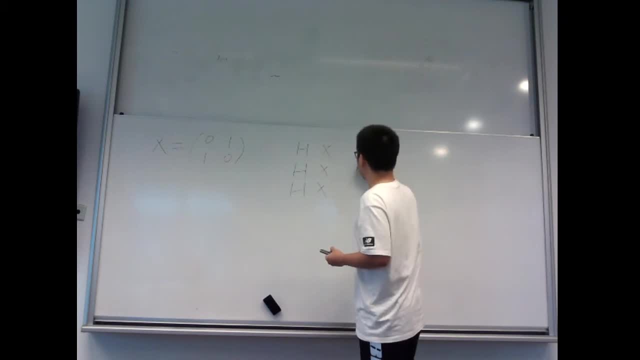 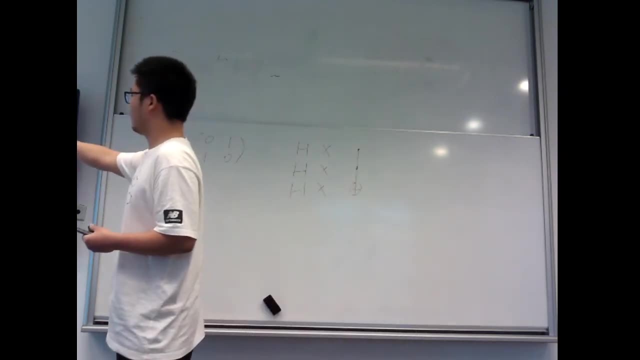 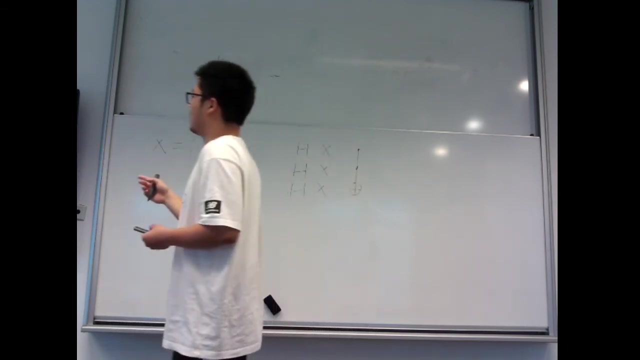 And then this This gate here. So, So that would That would be much more clearer if, like the, I separate the Oracle and the, The part that actually does the search. So it's actually very Because here it's, It's all. 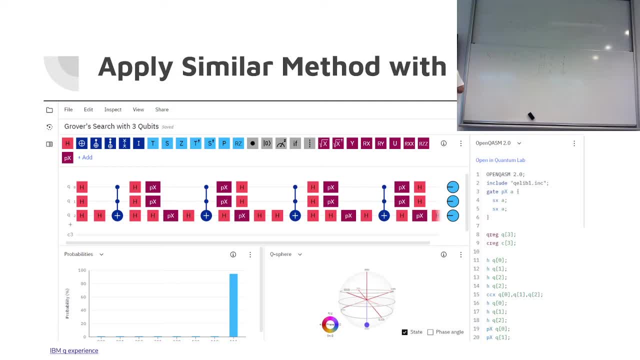 It's: Yeah. Yeah, I can see, I understand that. Yeah, But actually I I thought that the other operator also needs something like a Toffoli gate or So, So it's actually quite interesting that this works. So it's actually not what I would have expected. 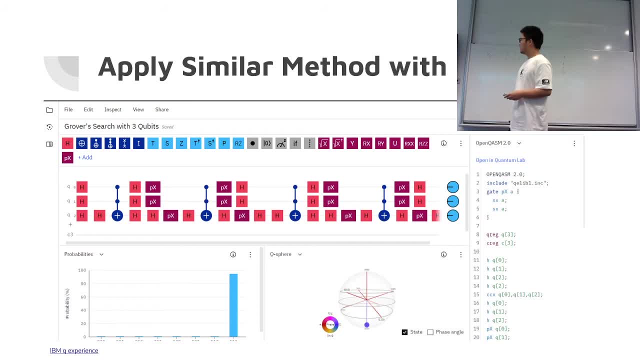 Like for the other operator, The, The Toffoli and the Hadamard. I totally agree with you there. But then the three H's and the X's is Is not what I would have thought Would work, But actually. 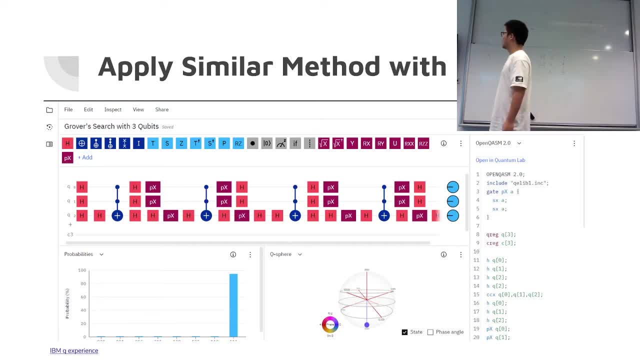 Apparently it works So. So you might have actually found a Slightly different way of doing it, So it's kind of different than our. Like the Yes, It's actually. It's actually a bit different, I'd say Yeah. 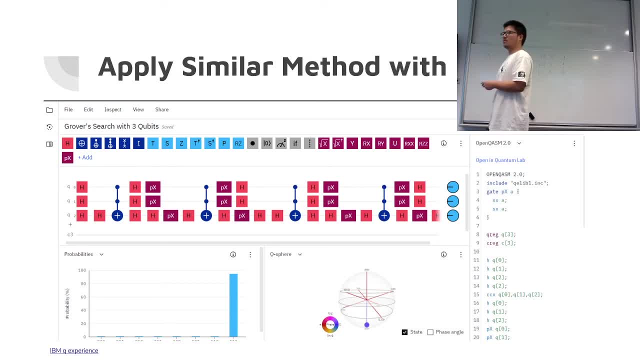 I'll have to, I'll. Well, that's, That's cool. It's, You know, Unexpected near results. So Cool It. I mean it still works. right, It, totally Absolutely. Yeah, Yeah, Yeah. 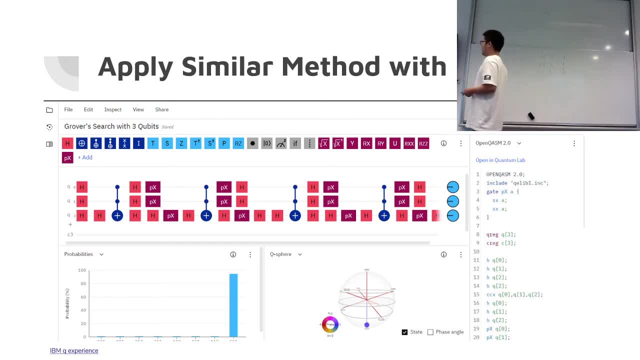 Yeah, It works, It works very well. Yeah, All the qubits are, Like all the probabilities, Mm And So So further, like Further on the result. This is actually The, The- All the probabilities combine. 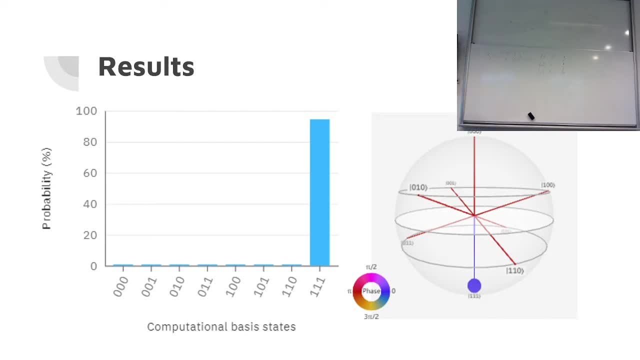 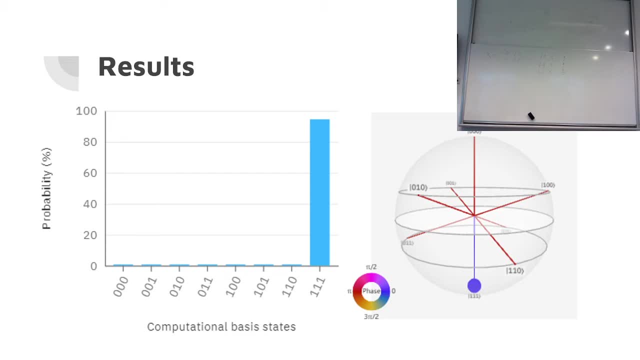 It's, It's, It's, It's 0.. There's actually some probabilities on the other qubit case as well. This is actually kind of confusing for me, because in the 2 qubit case, if you can check it out here- 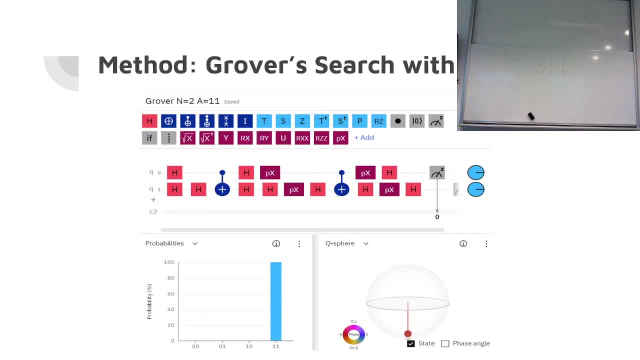 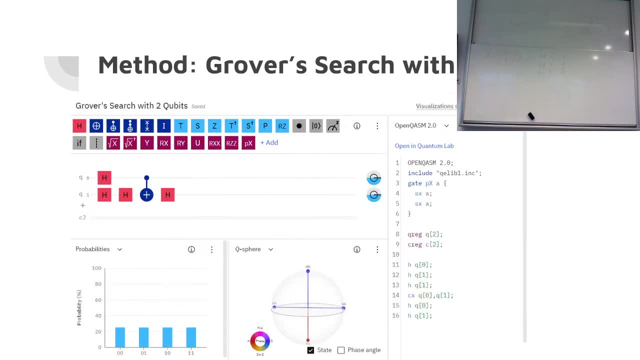 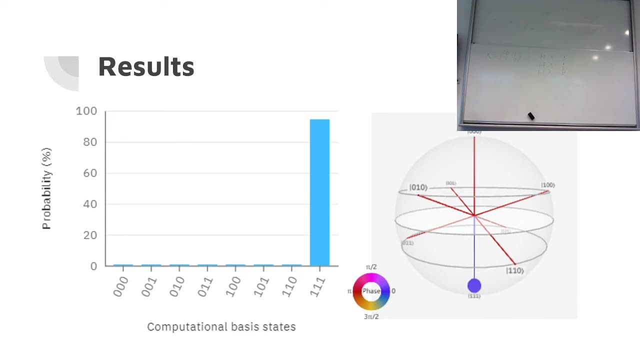 there's actually like this: probability is actually 0 and the test results show that they are 100% on the 1 and 1 qubit, But at the 3 qubit case we are actually seeing some probabilities on our other qubit as well, And for the sphere, for the Q-sphere. I couldn't. 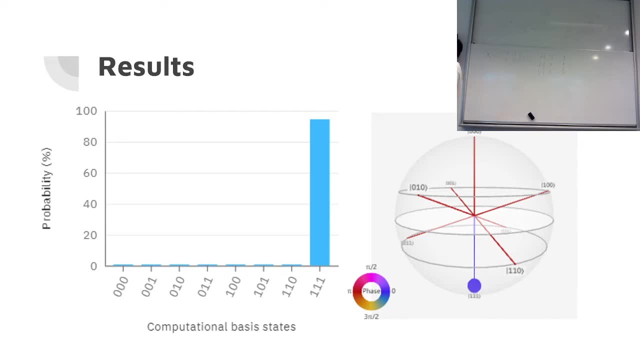 really understand what is going on, because it has many, like it has too many states and that's a bit confusing for me. Yeah, actually I also don't understand it because actually this block sphere representation is like I think it's generally not so easy to extend it to larger spaces. 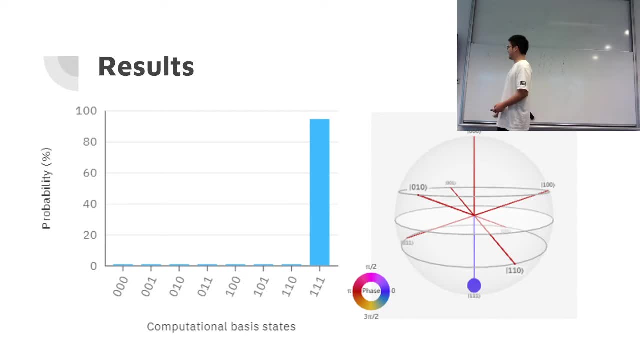 It works for 1 qubit, but then for other things. it's not really an exact. I don't know. I don't know how to really do it. Maybe they just sort of made a, you know, they just equally distributed all the orthogonal states on the sphere. 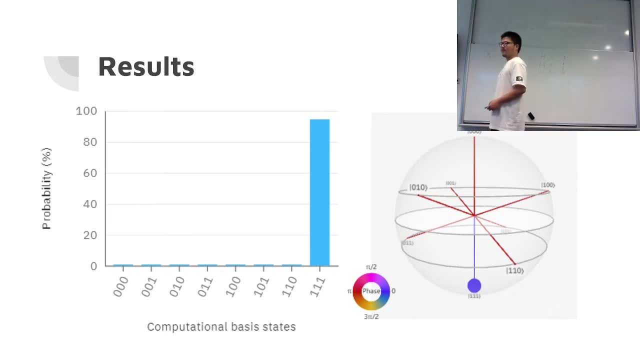 Is it like a projection from a 4-dimensional space? No, No, That would be even harder to understand. That would be smart, but I don't know how they would do that. So yeah, But maybe it's nothing, Maybe they just made it up. 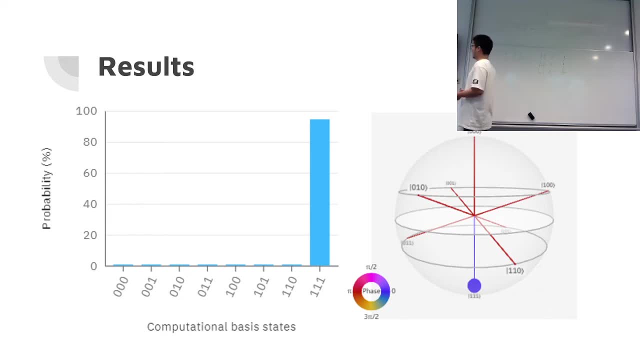 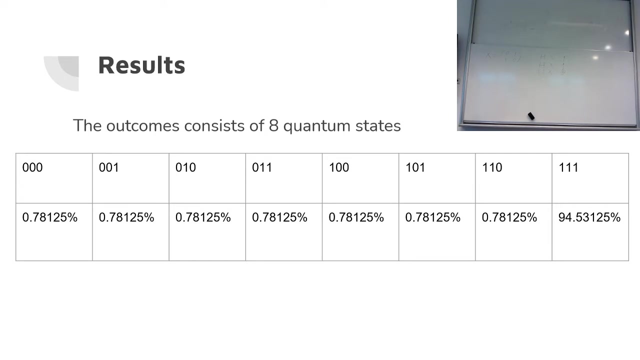 Yeah, but I think the probability cases could illustrate the results pretty straightforward enough for me. So I always kind of just look at the probabilities: Yeah, Yeah, And this result here actually In the test case, the actual result in numbers is actually here. So for all the other states, 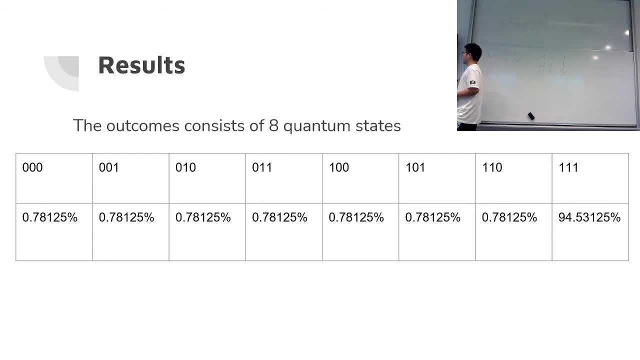 except the one-on-one case, the probability are all 0.78125 kind of percent. This I found I found quite interesting as well, because I originally thought that these were all the other states were just like computational errors that are generated from like computer. 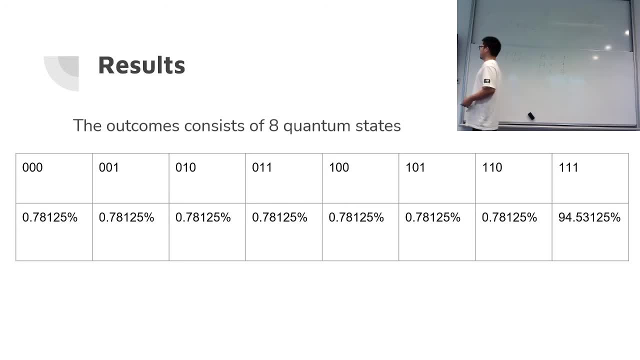 tests, because I guess 3-qubit they should like it's much more complicated than 2, and they would actually have some test errors, But the probability is actually, you know, all the same. So it got more confusing from that. But aside from those errors, which 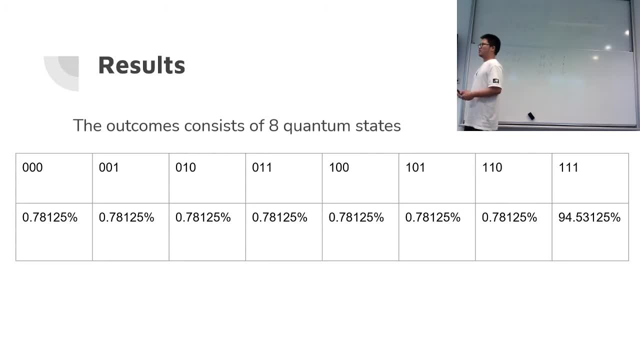 to this point, I'm still not very, I still don't really understand how they, how they occurred and like, how much, like how did they end up being the same one? The test results is actually: Yeah, about 94% case. about 94% cases are in the one-on-one case, which is really good. 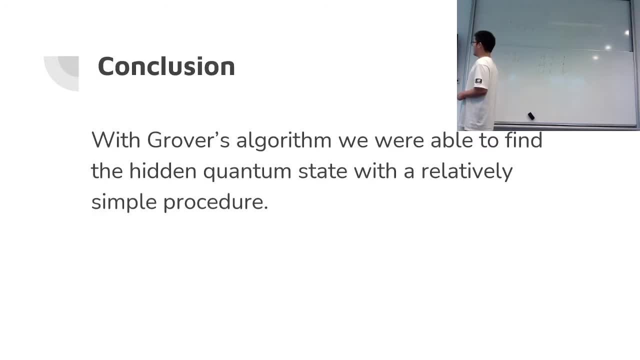 So we arrived at our conclusion that with the Gorbas algorithm, we were able to find the hidden quantum state with relatively simple procedure and like, just basically, you can just find one one thing, like with your- Yeah, with your first, like do some correlation with your like first shot, and which is: 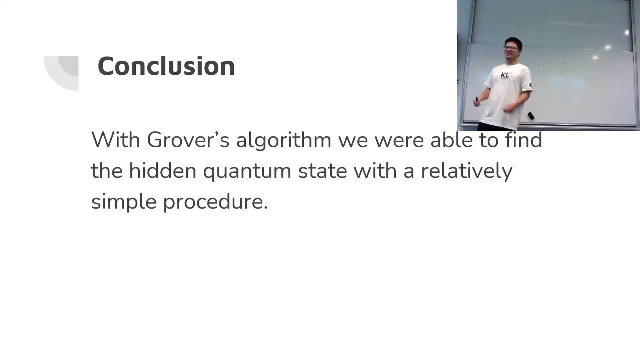 really amazing to me. Imagine, like, if you play poker with that and you just randomly draw one card and say, yeah, I found my card. Yeah, So this is my assignment and my presentation, Thank you. Thank you for listening. 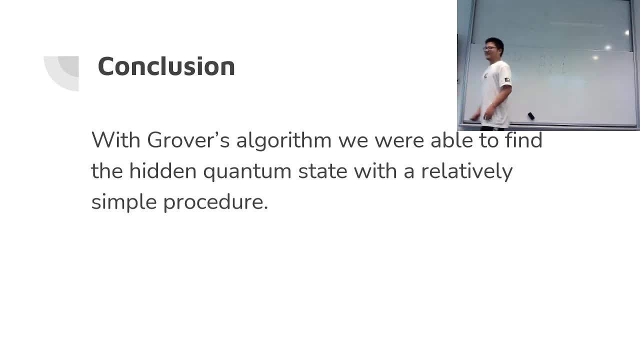 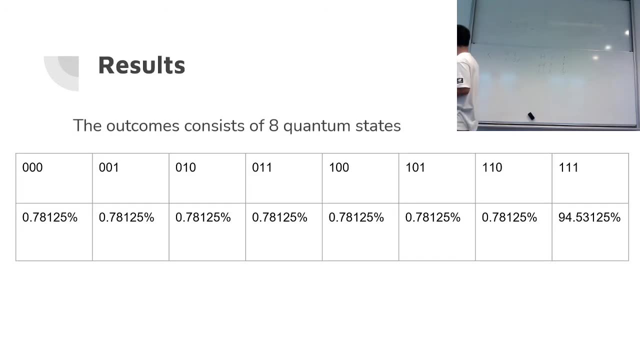 Great, Yeah, yeah, Very nice. So, yeah, I mean regarding the percentages. yeah, that one, Yeah, So it could be because? So actually, in Grover, you have to repeat this, block this oracle, and then the other thing, And then you repeat that several times And then 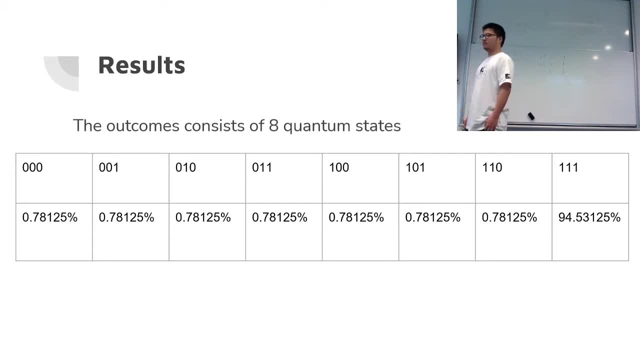 what it does is like it gradually changes the initial state, which is a superposition state, into the final state. right, But it does it in kind of discrete angles. I'll talk about it in the lecture And then. 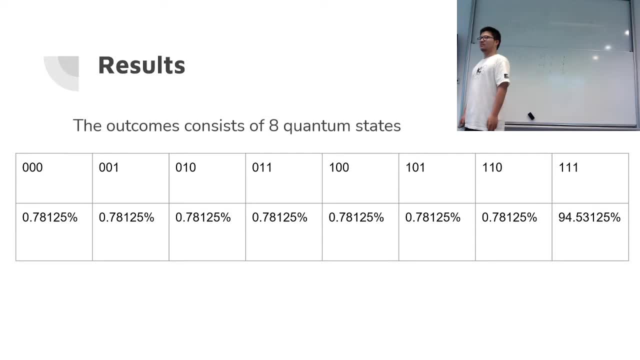 so maybe it just kind of just it doesn't quite get the top of the probability, maybe because it's kind of discrete, It just kind of misses it. So it might be because of that. So it's kind of like separating to each steps and 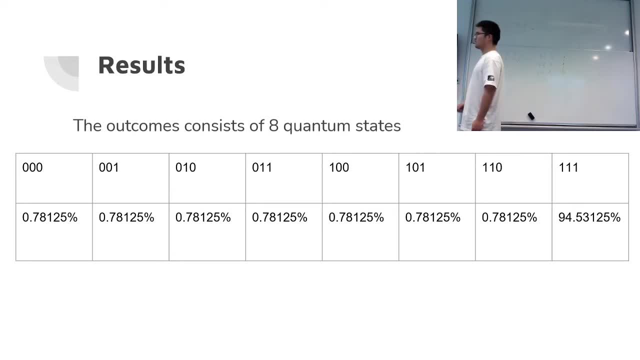 Yeah, Yeah. But basically because with each Yeah. pair of operations that you do, it gets some angle closer to the real result. Oh so, But then if that angle isn't like exact, like multiple of five or something, then 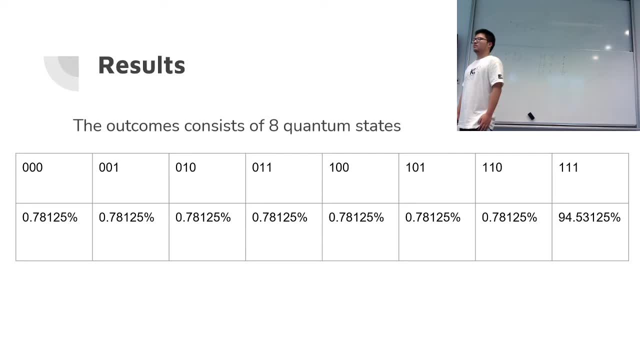 it might just kind of miss it right. Maybe for the two qubits doing two exactly gets it like: Yes, because when I like, when I add more, like add the more, Yeah, When I add more of the similar operation, like repeating those steps, the probability. 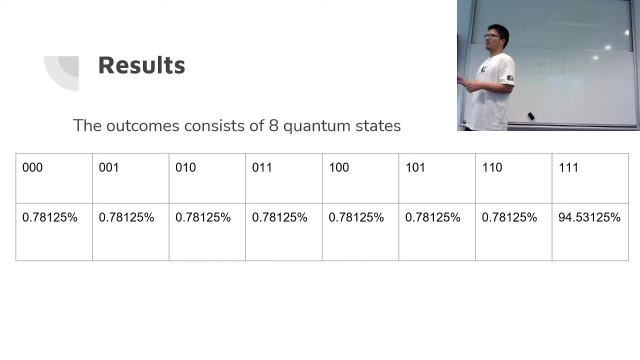 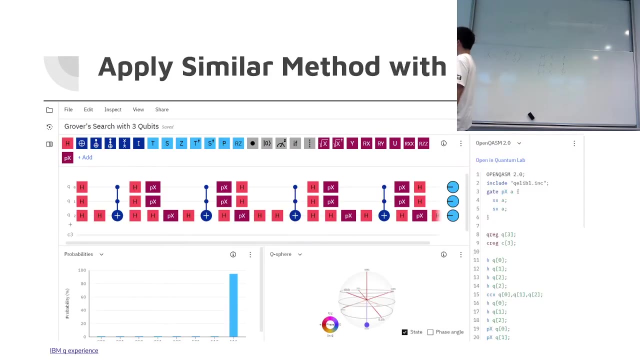 actually kind of fluctuates around, like sometimes it increases, sometimes it decreases, and Oh really, Yeah, Oh. so sometimes it's not exactly this number, or Yeah, When I had a like, So this circuit, This circuit is a really good, It's a really 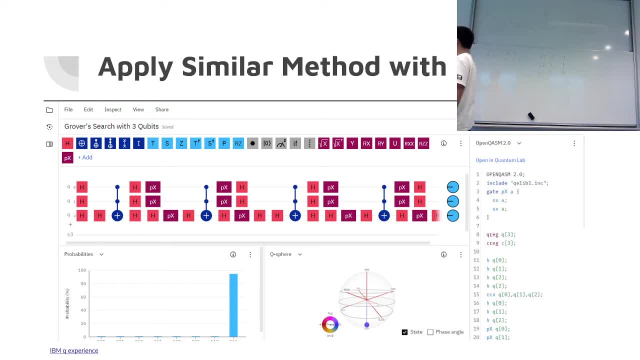 good case. so Because, like the one-on-one person, the pretty much you know one-on-one person- the percentage is really high. so I choose this as the presentation case. but I actually like skip some circuit here and when I try to like compute that percentage. 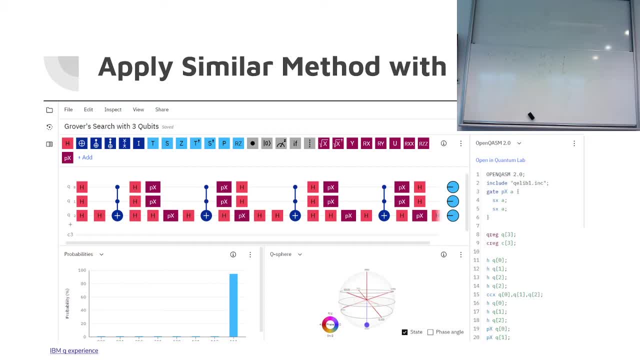 it. So the Each of the others, they have a relatively higher percentage than this case. Mm, I see, Yeah, right, right, right. So, yeah, I think that's consistent with what I'm just saying. 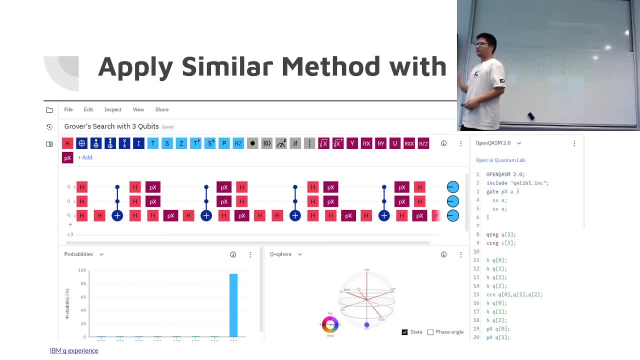 Mm-hmm. So if you're doing a certain number of these ones, you need to get the certain number right, Yeah, And if it's too few, it will, yeah, not be. That's good at the maximum, yeah, And if you do too many, by the way, it'll also overshoot. 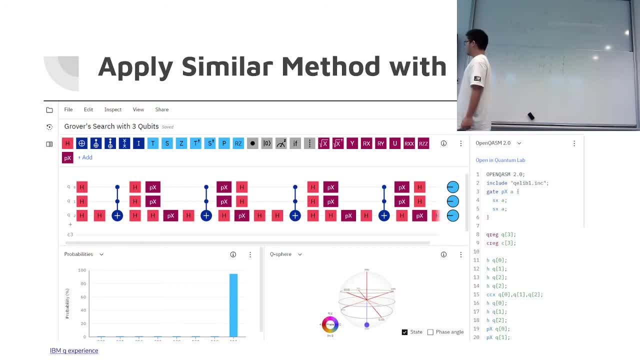 Yeah, And you'll actually get worse results. yeah, Mm. So, but just the fact that these numbers are so exactly the same, maybe, Yeah, Is this maybe the simulator of the quantum computer, or is it the actual quantum computer? 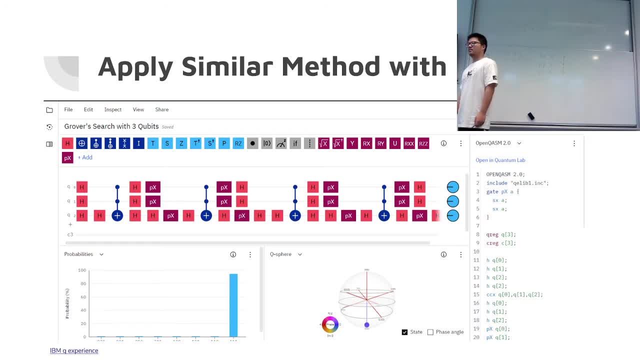 Because I think I know that there's a simulator and then there's also the thing that you actually can run. I wouldn't be surprised if it's the simulator, because they're all like so, even like evenly distributed, Yeah, yeah. 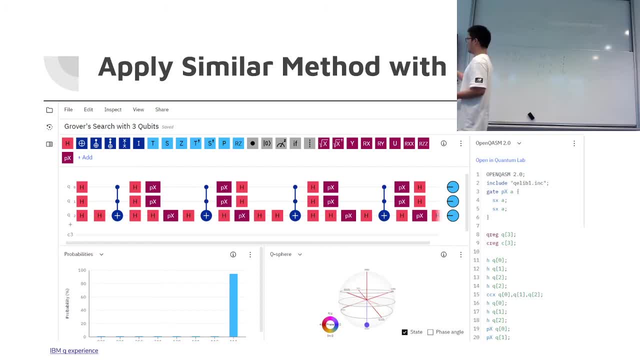 So I imagine the real computer you can, You might get some like like I don't know, Maybe one case will be higher, another will be fewer. Yeah, There's kind of distribution Exactly on the probability there. 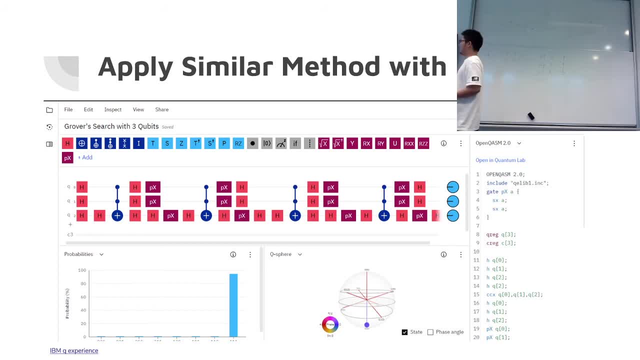 Yeah, But they're so even so. Yeah, that's also kind of confusing. So maybe- I don't know, I've never personally used it, but maybe you need to- I don't know- apply for a different. 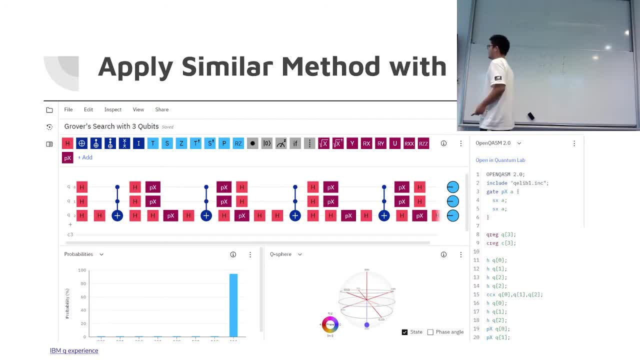 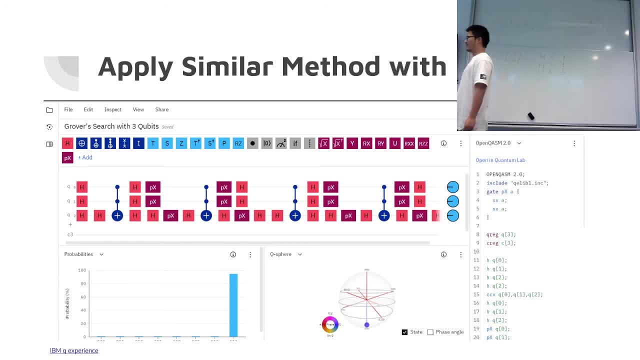 But I think, Yeah, I'm quite interested in this new gate, This other gate which is, I think, not the usual one. You mean this: Those 3 H's and the X's, Oh, this, Yeah, Yeah. 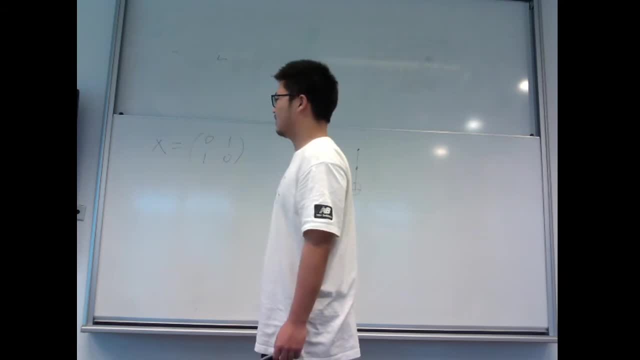 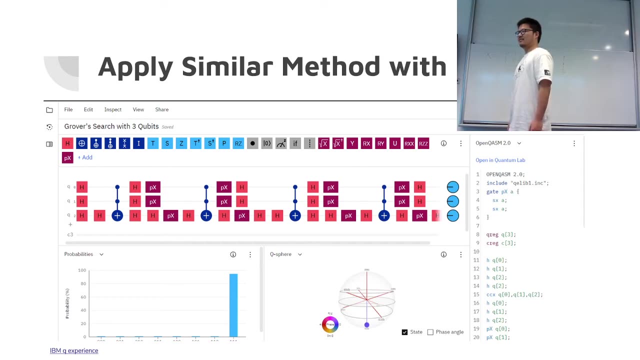 All of this gate? Yeah, So that that thing, Yeah, I would be interested to know why that actually works, because it's actually not the one which I would have thought. Yeah, If we have time, maybe we can look into it. 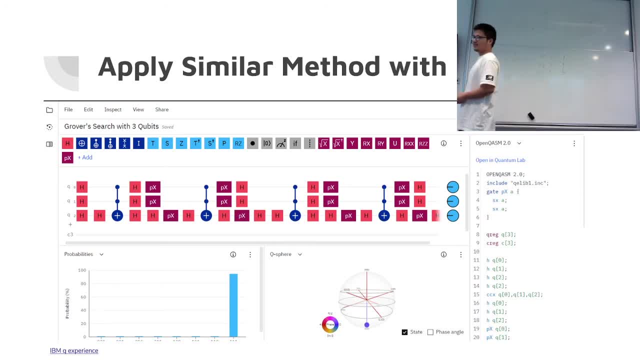 Very good. Any questions, Elaine? I'm also wondering how the 3H gates can perform this search. Is there a computational proof of that? I did some computation in the matrix when I was figuring those gates out, But I kind of just understand them as the first changes. 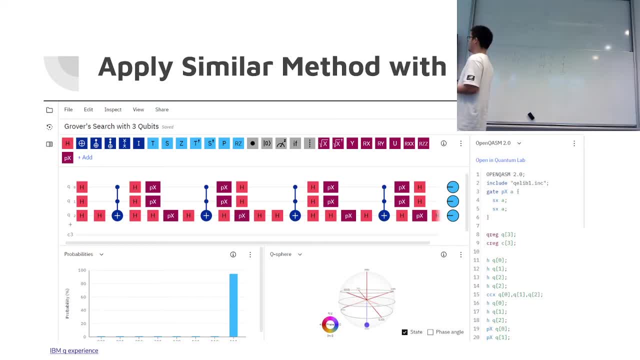 in the matrix And then they kind of flip each state And if the state has information it gets flipped around And with each state flipped the information in terms ends up at the last state there. I guess I could look into it. 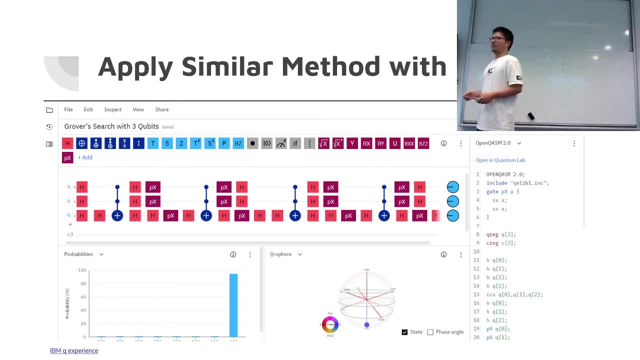 So you're looking into the computational proof of why the search actually works. Yeah, I mean probably the way that I would do it is just that I think I'd figure out what the eigenstates of that combination is, this H and X thing. 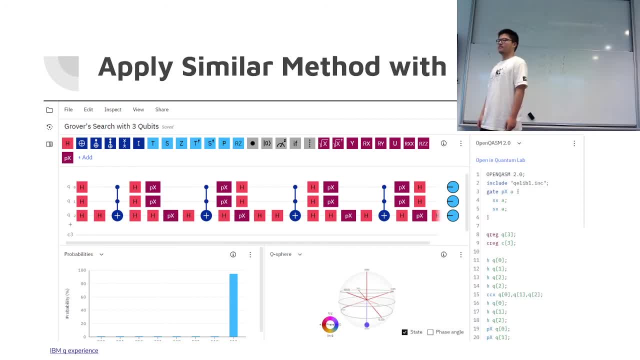 And because they're individual qubits, it's actually just a one qubit calculation And then maybe we can work out something from the eigenstates, Because there's kind of a couple of ways of looking at this Grover's algorithm And there's another way which of course I'm not telling you in the course. 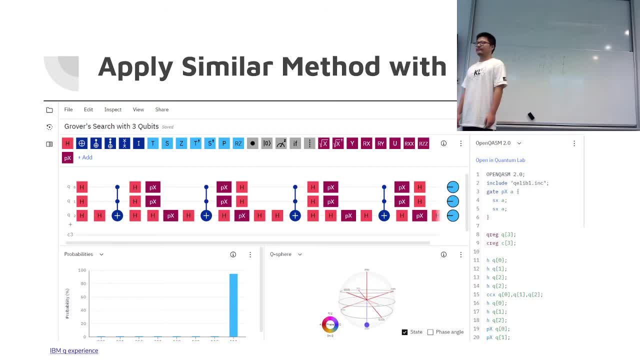 is sort of beyond. But another way is to think of it actually like an energy transition. So actually almost no way gives this interpretation. I wrote a paper on it last year. Can we see that? Yeah, But basically it's like if you think, remember these unitary gates originally are some Hamiltonian. 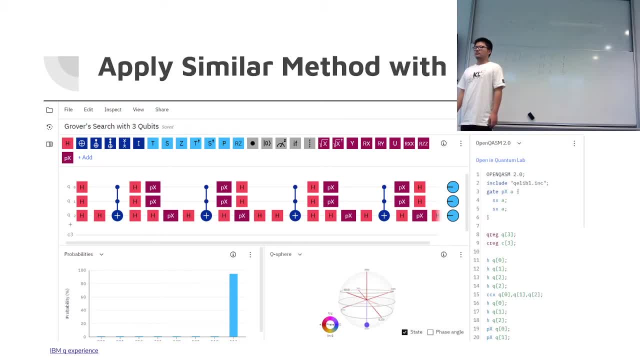 Right. And then the Hamiltonian is something that tells you something about the energy Right And basically what this Grover does is to you can think of it also as some energy transition between this initial state. So what this second gate, your triple X, triple H one is supposed to do is to make a state. 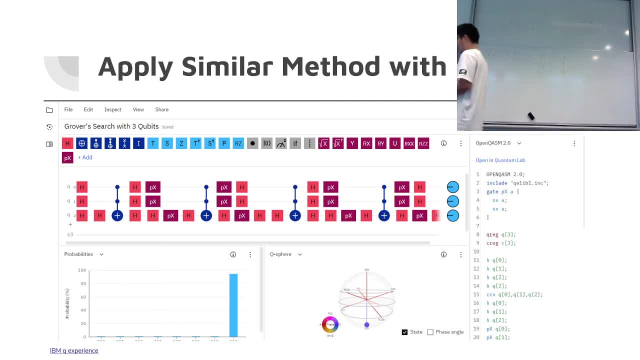 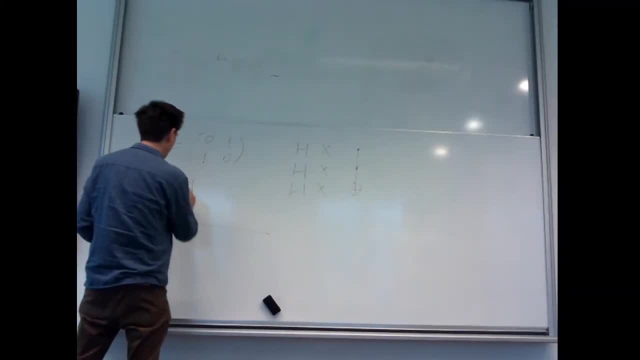 which maybe I'll throw up. Yeah, So another way to view this is for your three qubit case. in energy space, You have basically all these states which are at zero energy, So it's like zero, zero, zero, zero, zero one. 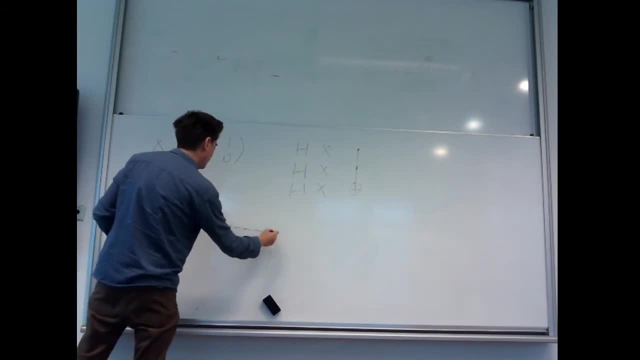 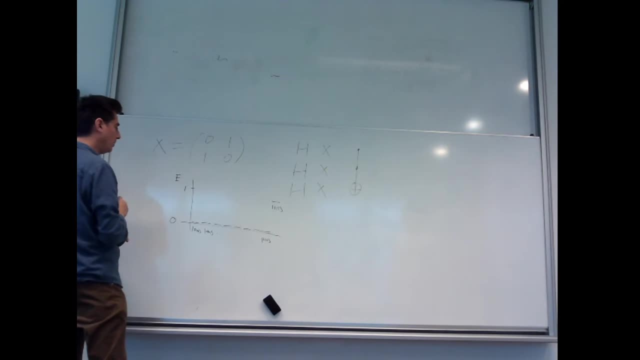 And then the last one, one one, zero. And then there's this state, one one one, which is your target state, And that's at energy one. And then, okay, this is not really proper, not quite proper, but just to give you an. 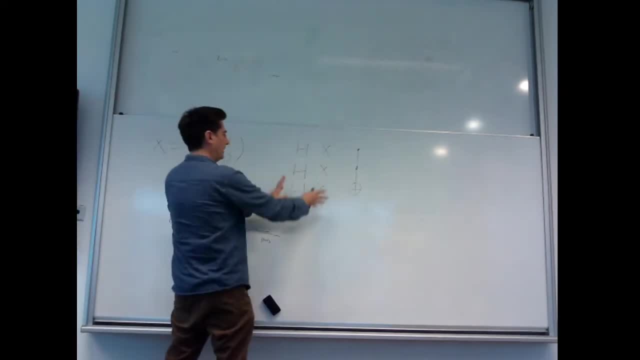 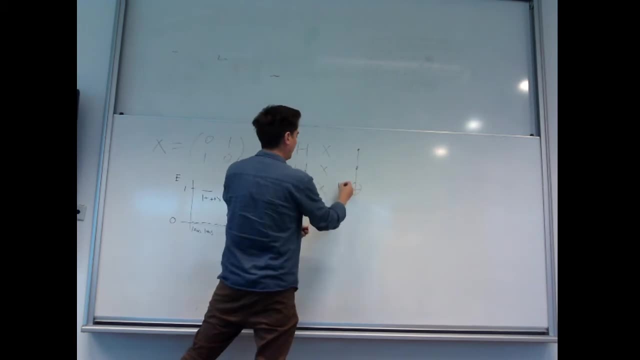 idea, And then this: so your triple HX thing is supposed to make this energy one, And then this other thing, actually with the. So this is your first one. Sorry, that's your first one. That's your second one. 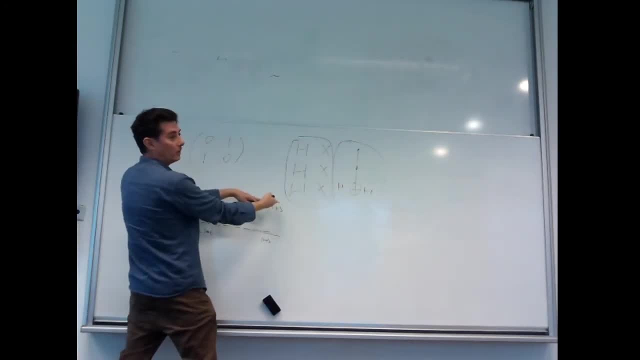 Right, That thing is supposed to make this energy one, one, one. And then what's supposed to happen is that this is because it's at the same energy. this one gradually turns into this one, And all these other ones haven't got the right energy. 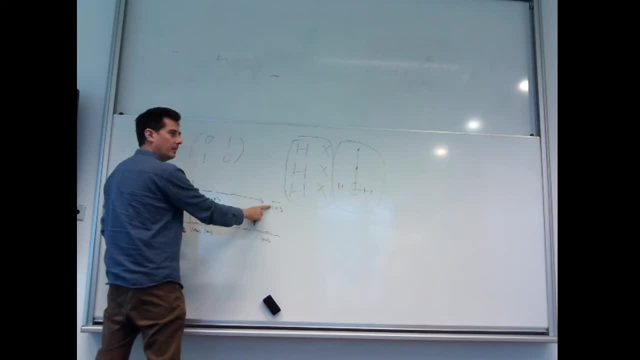 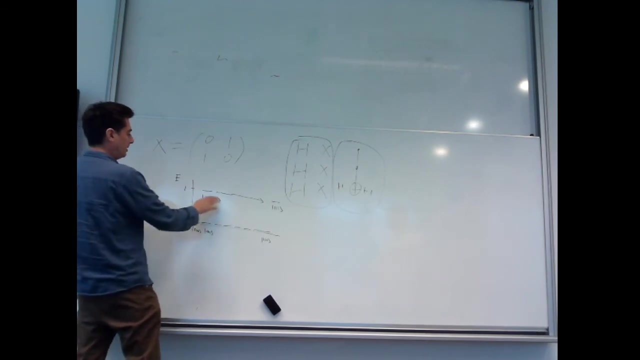 So that's why this one wants to turn into that one and not any of these other ones. This is sort of another way of viewing Grover right, And so I think what might be happening is that this thing is probably something that makes this state with energy one. 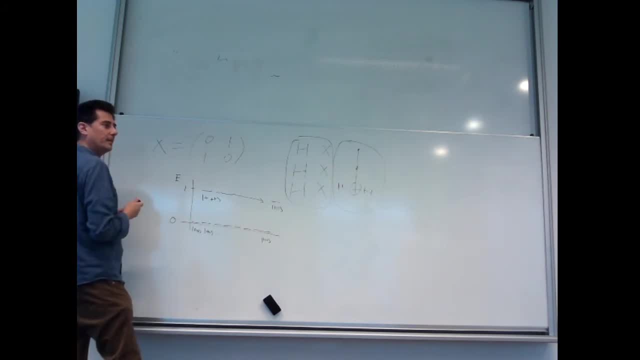 even though it's not the usual one. that's in the textbook. So it reduces the energy from all the other cases and then just leaves behind the Yeah. So somehow you know, maybe your energy landscape might not look exactly like this, but then it might effectively just do the same thing anyway. 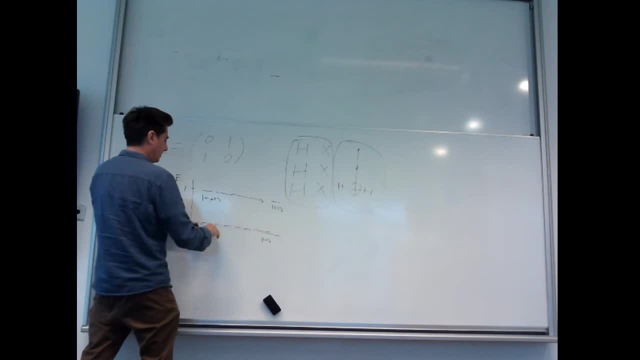 Like, maybe your energy landscape looks a little bit more like some of these other states and zero and whatever. But maybe it doesn't matter somehow in the end, because so long that your initial state, this one, is an energy one and this one, that one for sure, does this right. 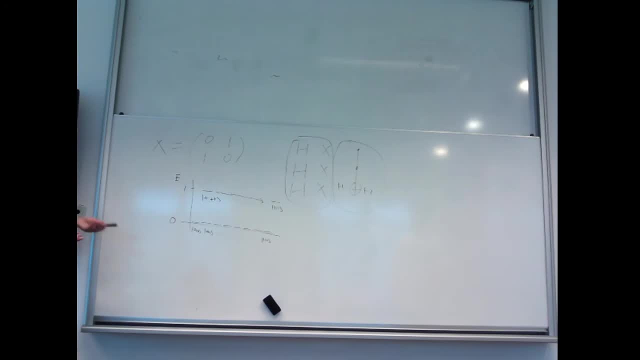 And then so it does the transition anyway. So, even though it's not the same thing, it still works. So that might be the way. Yeah, we'll look at it, But anyway, yeah, that's great. Any other questions? 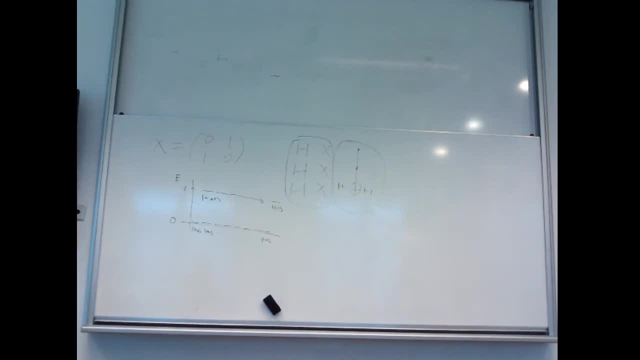 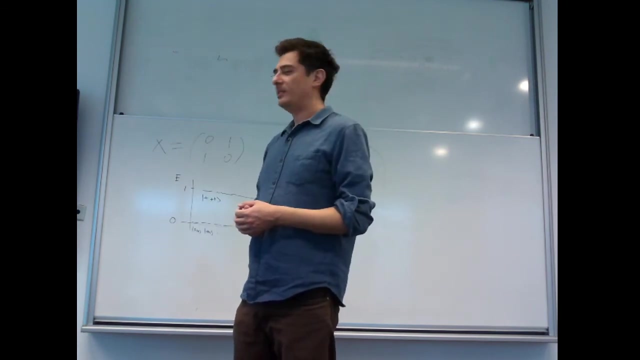 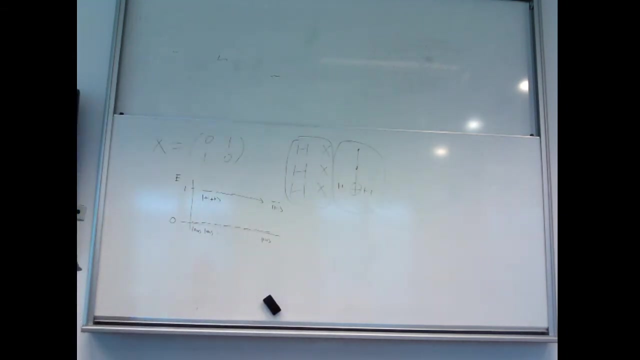 No, Okay, Great, Thank you, Okay, Yeah. so I don't know. I think it's quite nice actually to have these assignments, you know, because it's not just me talking at you all the time And you can sort of find something a bit new sometimes too. 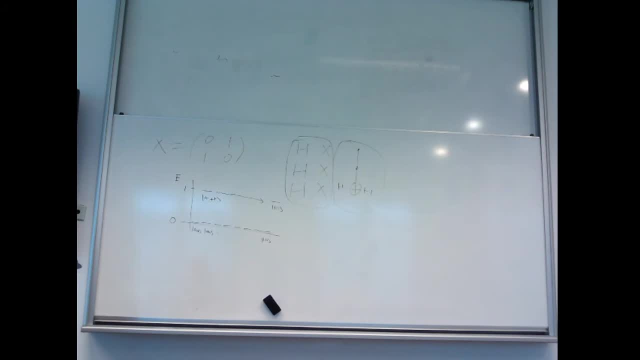 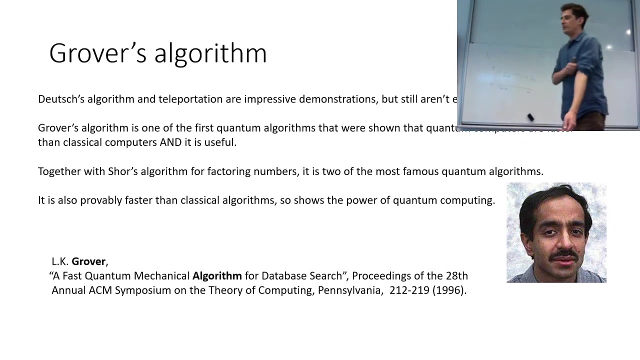 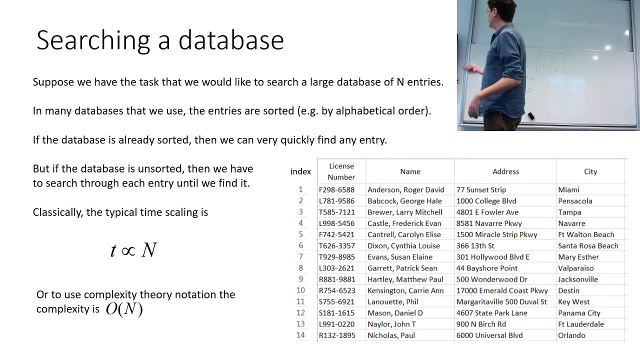 Okay, Having said that, let's go back to the lectures. Okay, So it's been a little while, so let's recap where we're up to. So, okay, we all know what we're over in Searching a database. 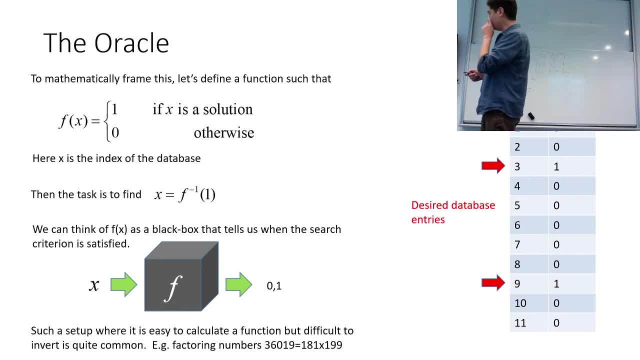 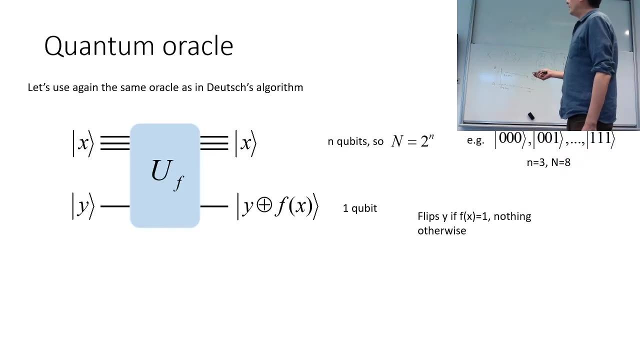 That's right, We were talking about the Oracle, And so we have a function that is finding these desired elements. So a king, as Daniel was saying, And we're going to use the same kind of construction as in Deutsch's algorithm. And yeah, and in a way, actually, you know. 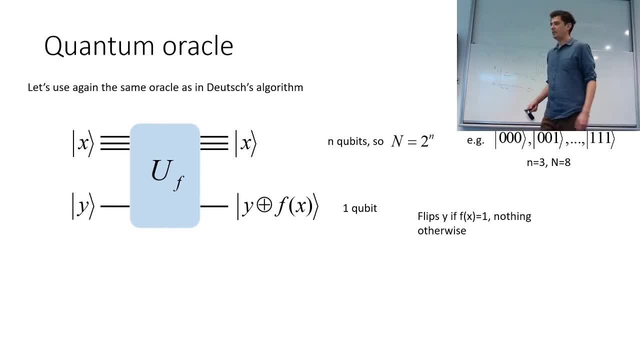 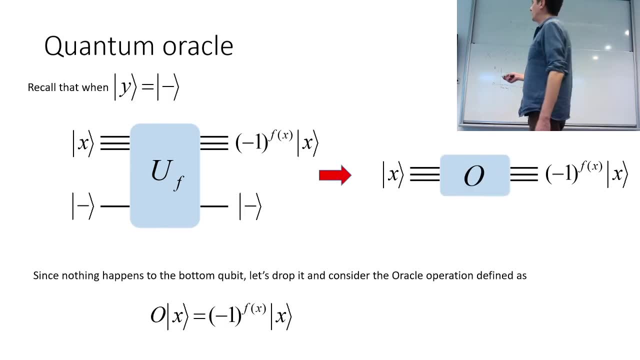 you don't really need to do this construction because essentially what you want at the end is some operator that kind of gives this kind of relation, So this, if you have the solutions to the problem, so this X. these are all the states. 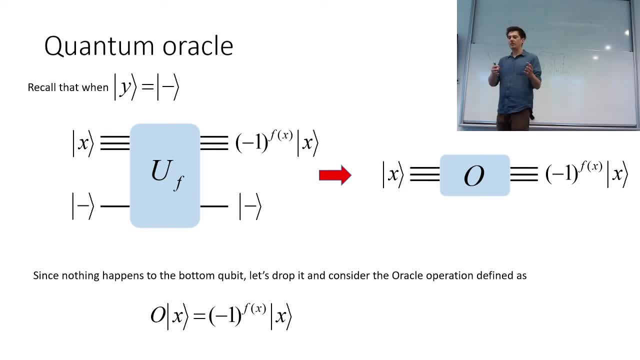 And this is a multi-qubit state that goes from 0,, say 000, to 111.. That was the case that we were just talking about, And one of these ones, which was the case in Danny's assignment, requires a minus one phase right. 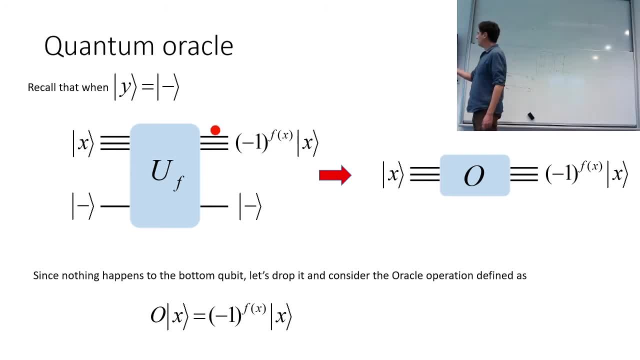 So, essentially, this whole construction is there just to create this effect, And you know, so we could have equally just started with actually this one, because the reason, if you remember the reason why we were talking about this, is we kind of made this thing to ensure that it's like a unitary, reversible gate right. 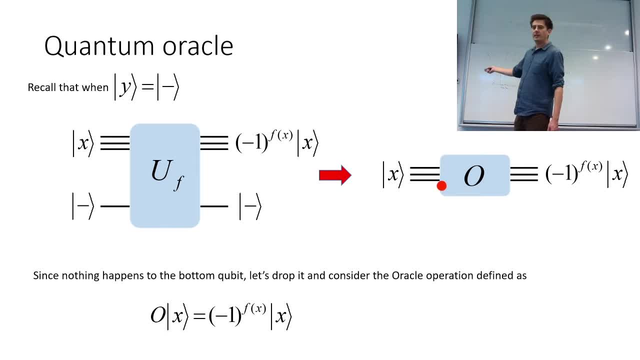 But actually this is a perfectly reversible unitary gate anyway, And in Danny's example, in fact, we didn't even use this extra qubit to achieve it. You can just use some kind of gate to make that minus sign. So I don't know. 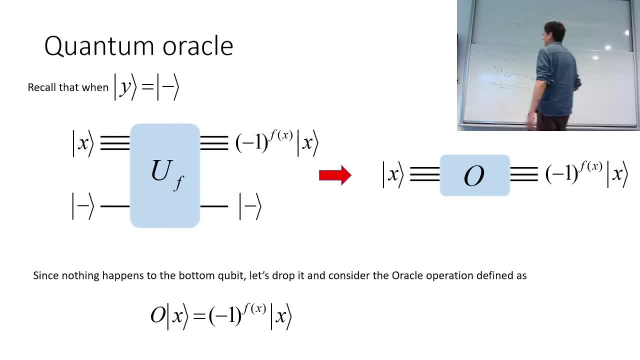 You could say it's sort of a historical artifact, or you know why do I bother talking about this? It's probably because when it was first conceived, discussed, you know, it appeared in this form, But I think, strictly speaking, it's not completely necessary. 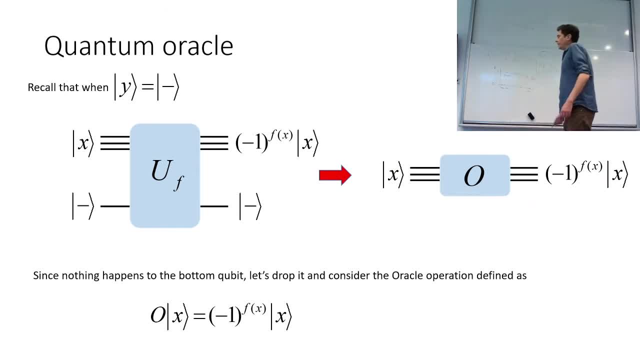 You could just start with this, Okay. So basically, henceforth, we're going to forget about this ancilla qubit, because we just want that minus one sign, And so we're going to find the oracle, just some operator that puts a minus sign on the state that we're looking for. 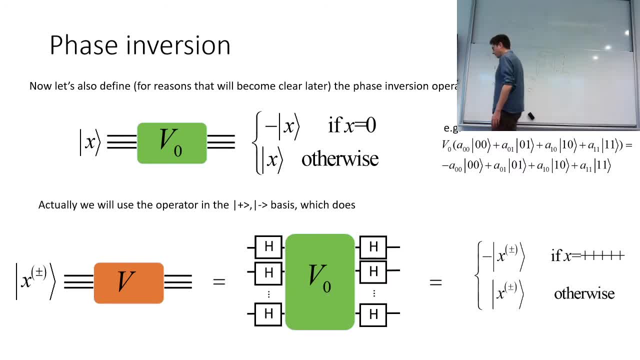 Right, Okay, So this is where we got up to last time, So that was one of the parts that we need for Grover's algorithm. There's another operator, which I'm calling the phase inversion operator, And this one is a lot like the oracle. 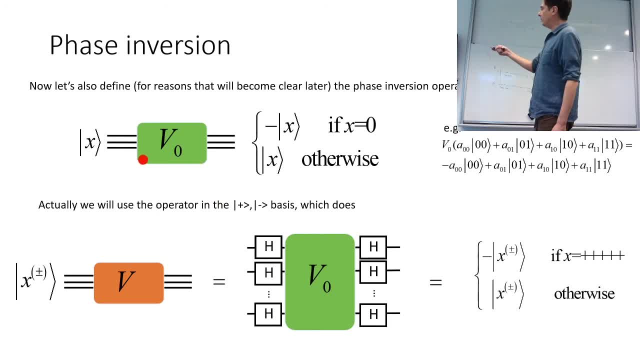 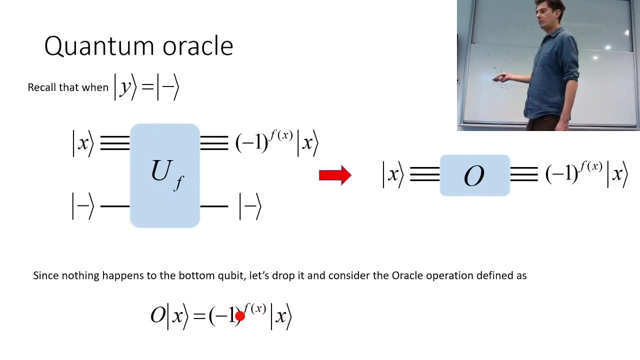 except that it always just adds a phase on the zero state. So just the zero state And the oracle. you know, this is dependent on the function or the problem that we are solving. So you know, depending on f of x. 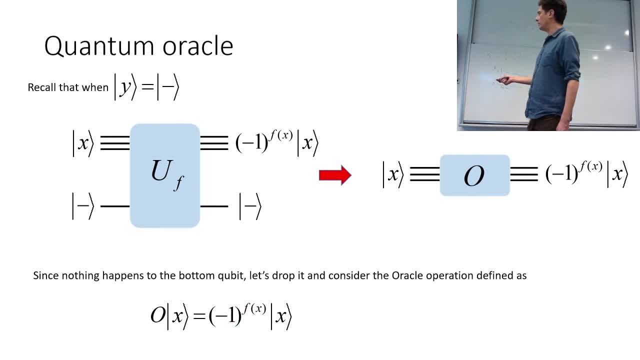 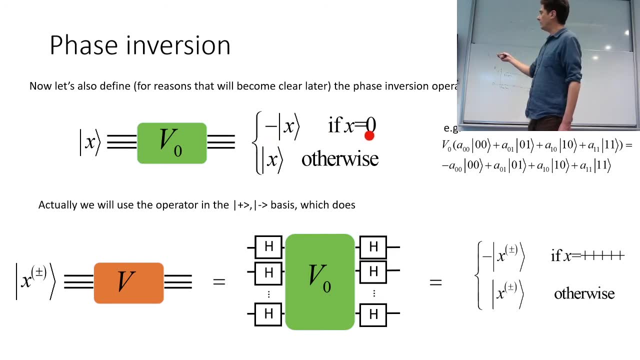 you'll have a different distribution of minus signs, But this one is always just this one And it's always just on the one minus. sorry, always on the one state where x is zero. And, by the way, when I write, x is zero. 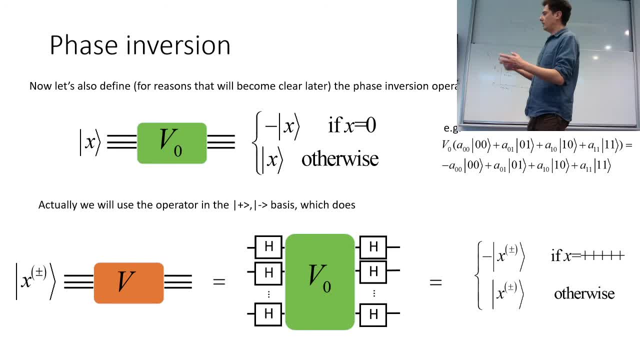 I mean this qubit is like zero, zero, zero, zero, like this state. So, for example, if I have this two qubit example here, if I start with some initial state there that's the arbitrary initial state, then what that does is to add a minus sign there. 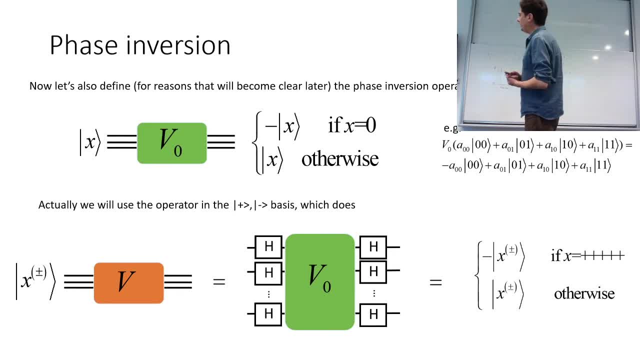 Okay, so that's the v zero phase inversion operator. But what actually we normally do is we surround this thing by Hadamard gates And basically what this does is to change the basis of this whole operator. So over here we're just working in this zero one basis. 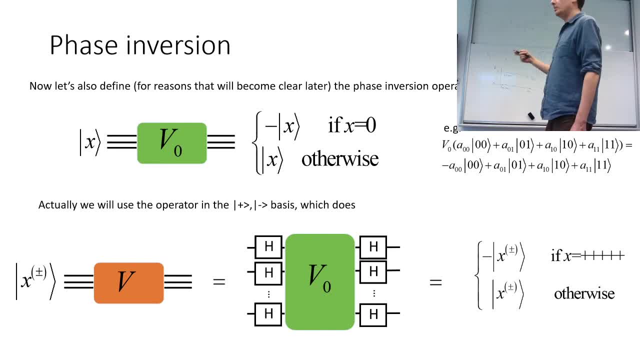 This is usually called the computational basis, because zero one is like the digital kind of basis. So if we put Hadamards before and after this operator, what basically that does is to change the basis of this so that it's not the computational basis that we're dealing with, the zero, zero, zero. 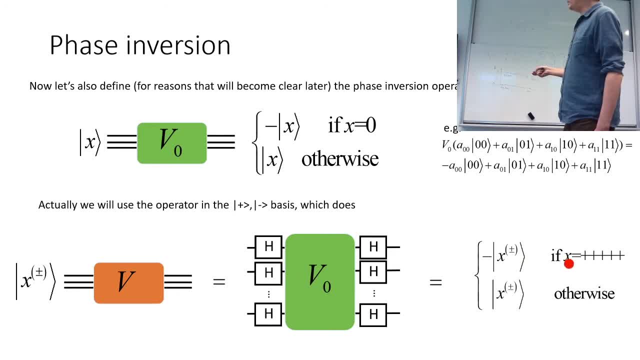 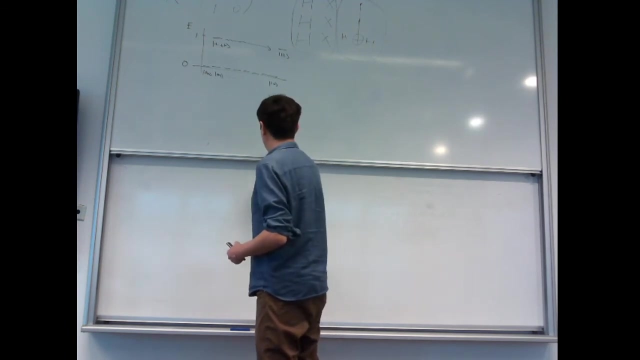 It's actually. we actually rotate the whole thing to this plus minus basis. So instead of writing, the basic difference is we're just going to write this one, So the v operator. so, if I have my input, that states x. I'll just do a two-qubit example. 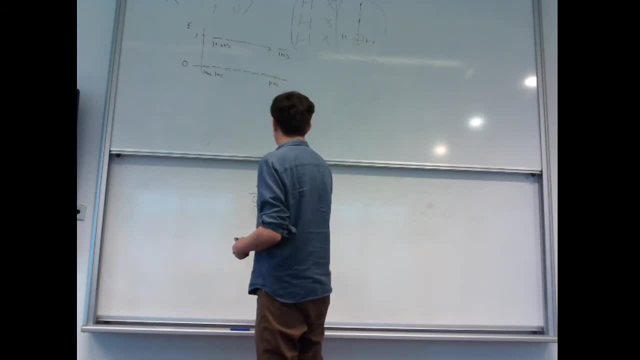 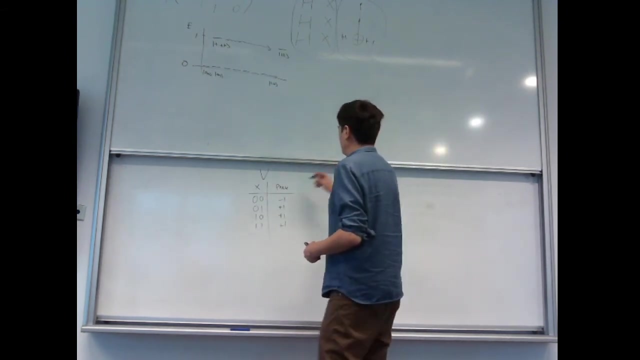 So basically the phase that we can have is: oops, so the phase will be like this: Oh, sorry, that was v zero, right v zero, The rotated thing. essentially, we're working in the plus minus basis. Maybe I should do that for consistency. 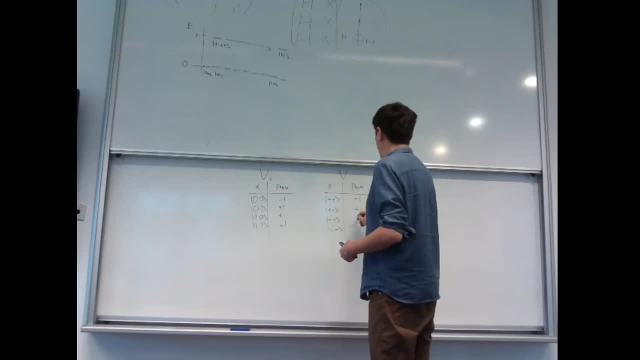 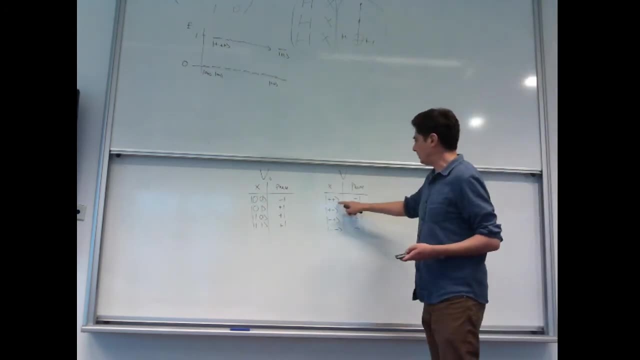 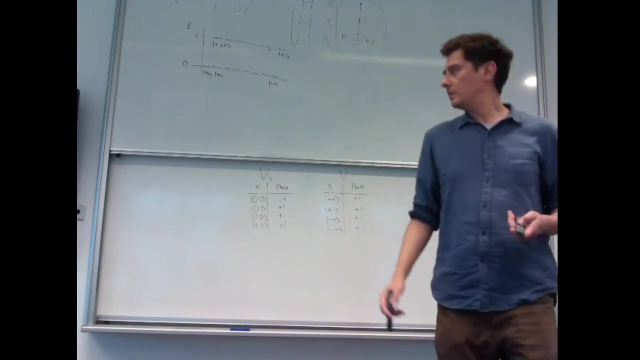 And it's. it's exactly the same thing, right? So it's just only that plus, plus, plus state that gets a minus sign and everything else has a has a just a regular plus sign. The first one has a minus sign. 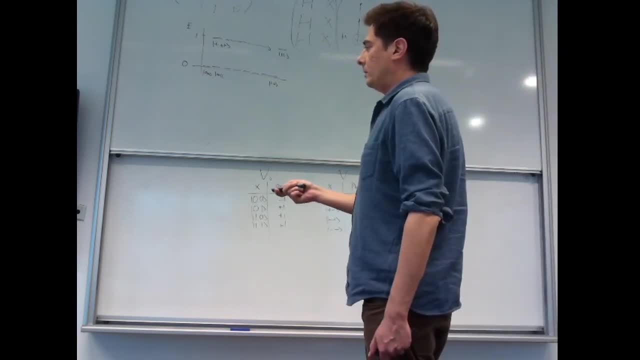 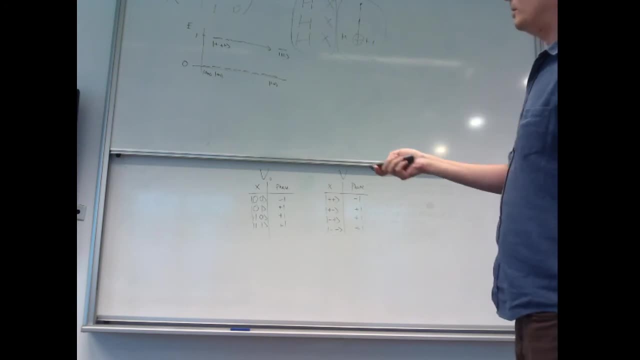 Okay, so that's sort of the second thing that we're using And this is the thing that we were just talking about with Danny's here. So this v- what Danny had as v is- was basically this thing here. I believe that. 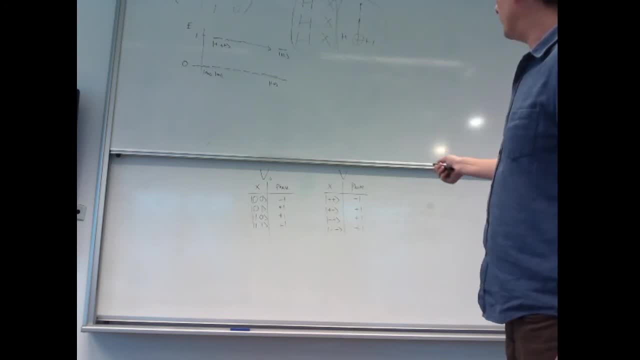 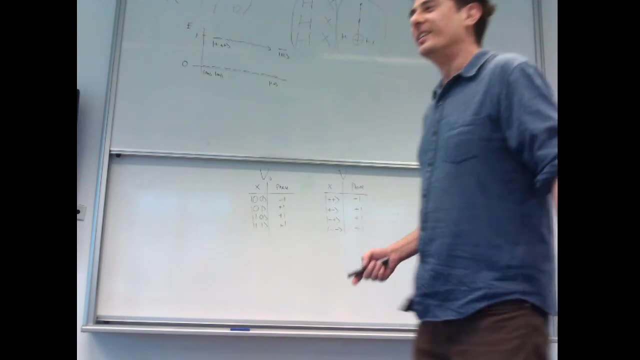 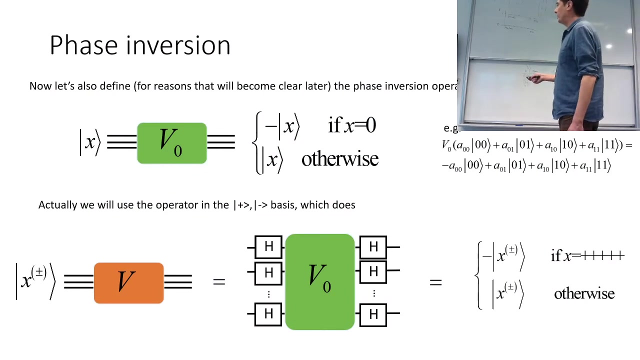 yeah, so I I think that that's that doesn't actually do do this, but but it must do something kind of like that because it still works, So yeah. so that'll be interesting to figure out In what sense it's similar. 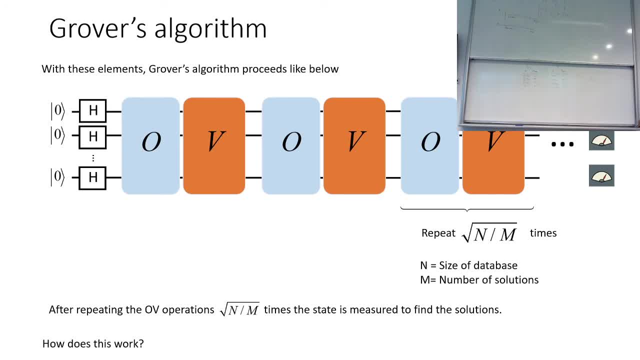 Okay, So then Grover's algorithm goes like this: So we have those two operators. Well, okay, So we start with making full superposition state here. So if we apply zero Hadamards everywhere, then initial state Hadamards everywhere. 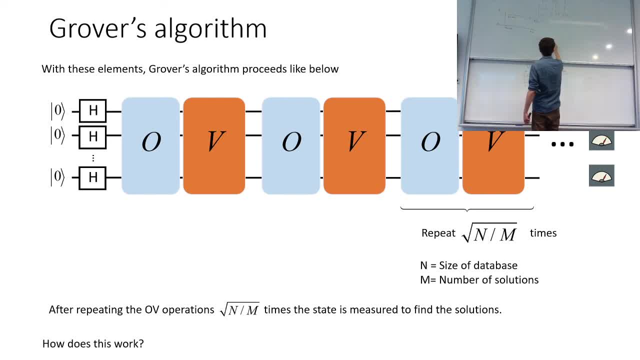 basically this point, this point in the circuit: the state is plus plus, plus, And plus plus plus is, of course, well okay. eight, zero, zero, one, all the way to one, one, one. 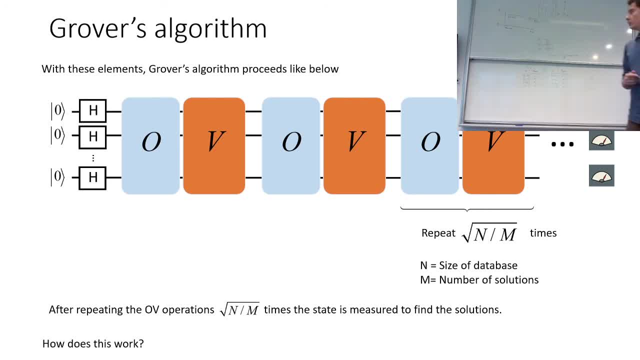 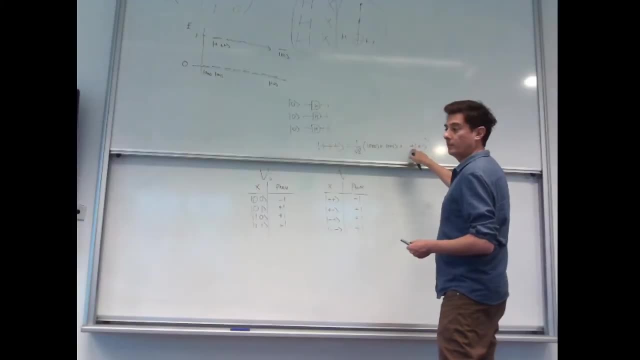 So it's a superposition of every possible state. And then we apply this oracle and that will change the sign of the target state. So in Danny's example we'll change the sign of that one, one, one one, And then V. 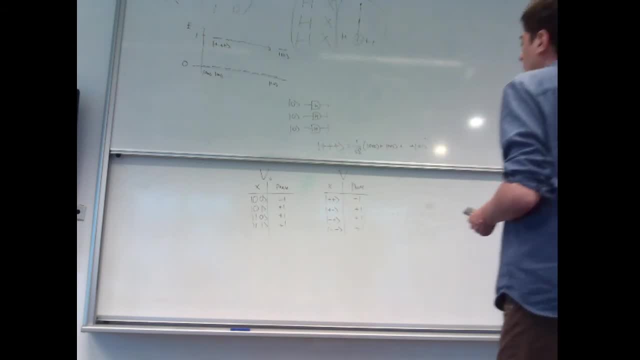 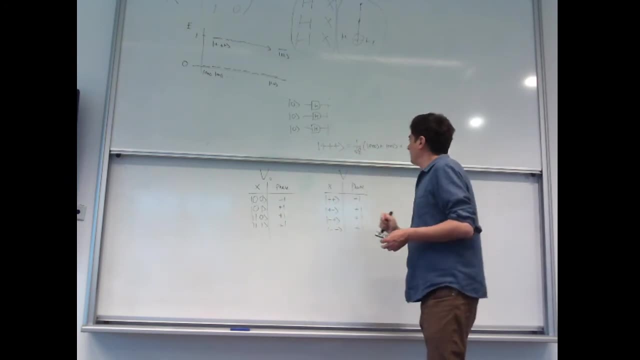 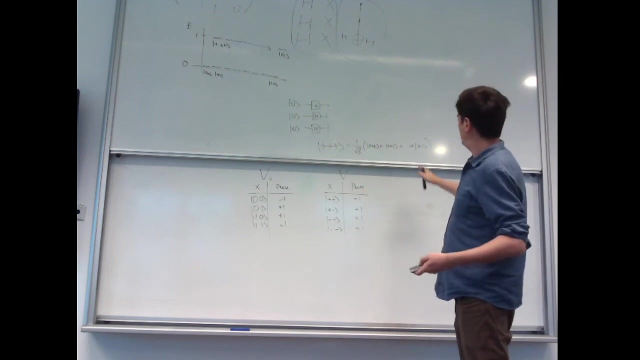 for V, it will flip the sign of plus plus plus, plus plus plus state. So because you know, after the first oracle this state is actually no longer plus right? So we actually have to work out what this does. 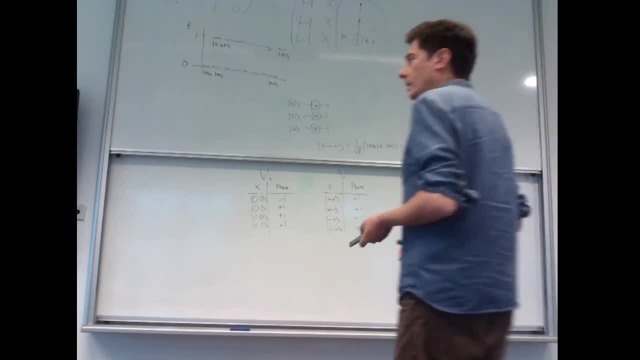 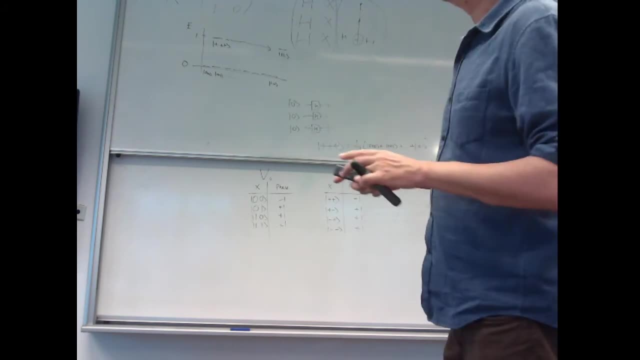 So it's not obvious just by looking at the circuit. what is going to happen to this In fact requires a little bit of a proof. So I'm not telling you on this slide, but I'm just telling you what the whole scheme is. 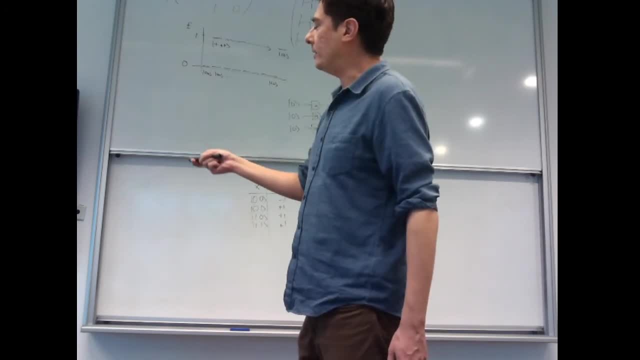 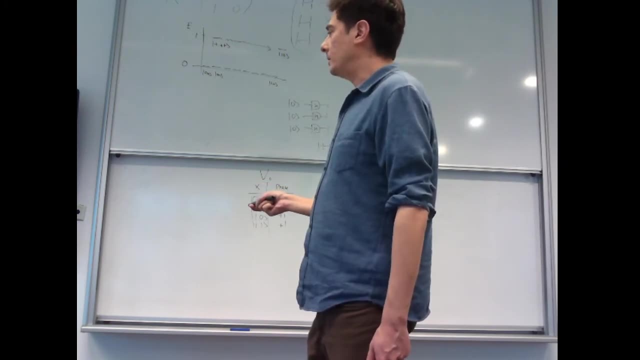 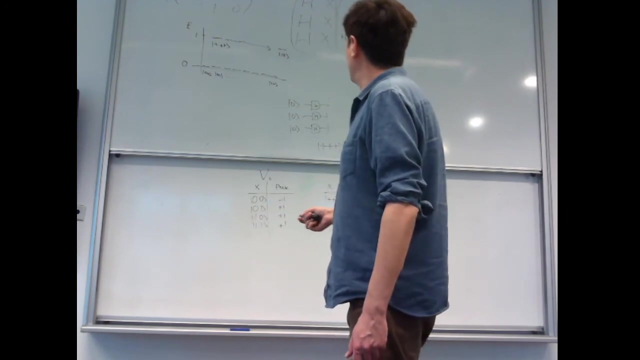 And if you repeat this O V combination some number of times and this some number, is the square root of N. This is the size of the database. So in this three-qubit example that would be eight, which is a power of three. 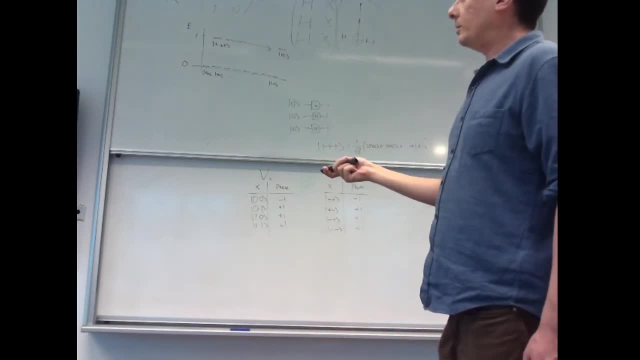 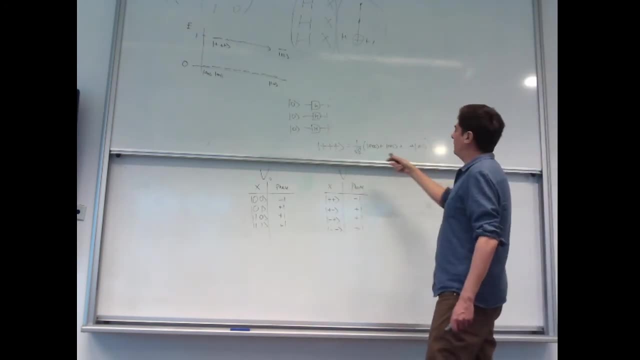 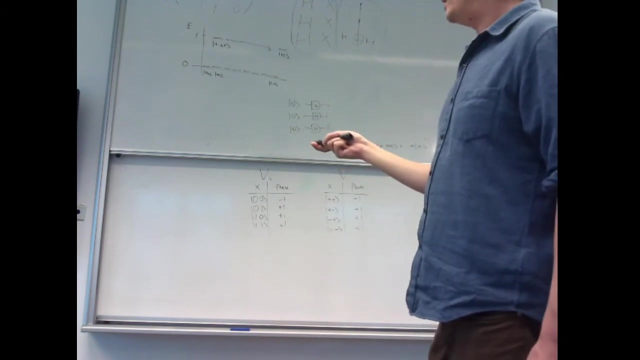 And N is the number of solutions that we're looking for. So if we're only looking for the one, one, one state, like we were for this example, then that would be one. So in other words, for the three-qubit example, 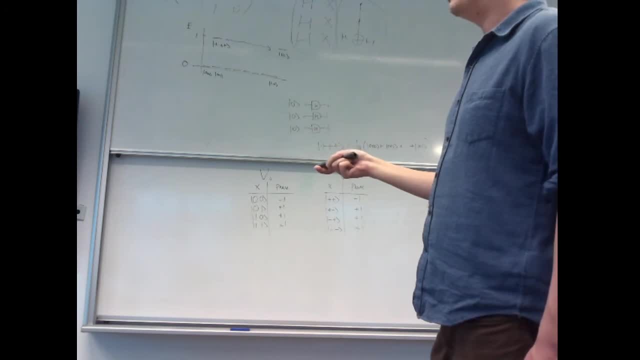 we would repeat this: square root of eight times Square root of eight. is what? square root of eight? Two point, something Closer to three than two, right? How many times did you do your? how many repetitions did you do Two or three? 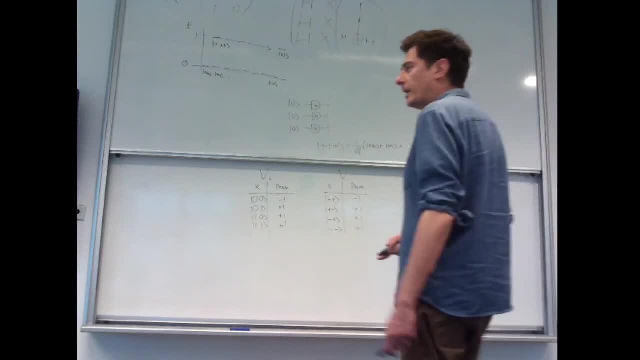 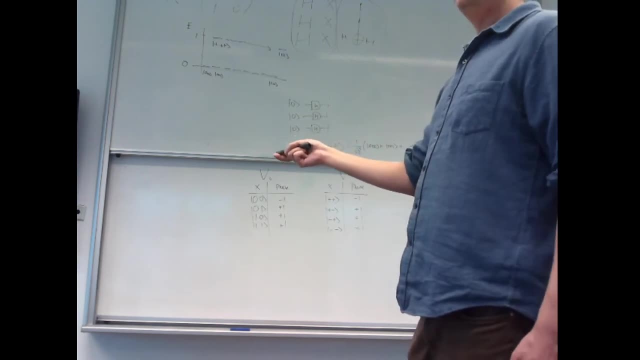 I think it was three, Three, okay, Okay. so there you go, It makes sense, So, but it's not exactly three, as we can see already from this formula, because it's square root of eight, right? So it's actually slightly less than. 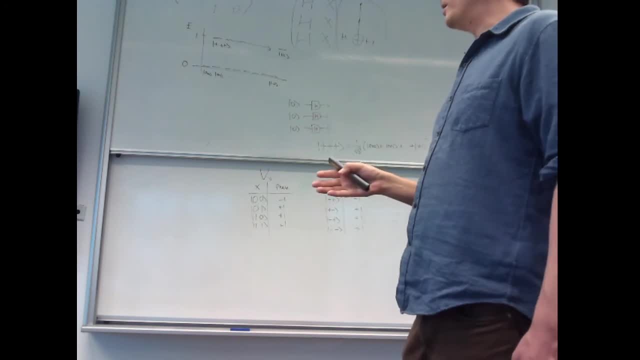 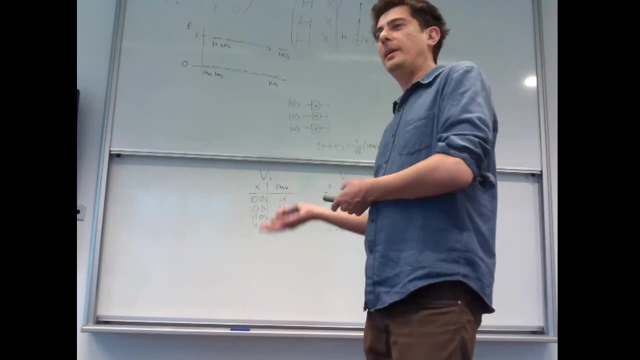 2.8.. Yeah, so, yes, exactly, Yeah, 2.8, that's right. Of course you can't do it 2.8 times. You have to either do it two times or three times, and three is the best. 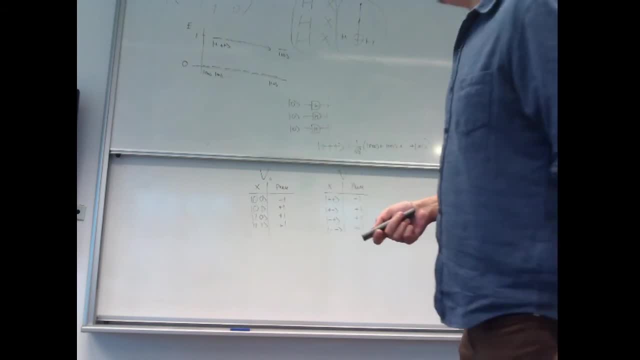 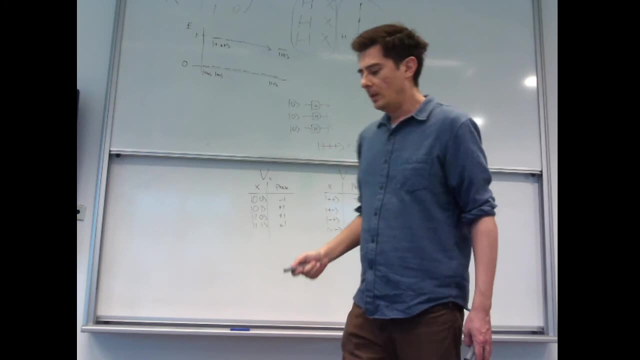 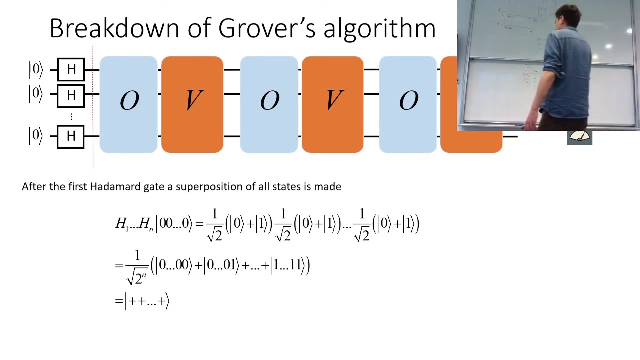 number of times to do it. Okay, All right, so that's the algorithm. and then, eventually, you measure it at the end. right, Okay, that's the algorithm, but how does that work and why does that work? So, oh, yeah, I think so. 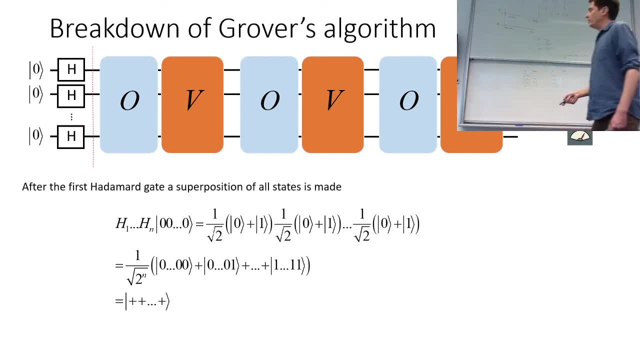 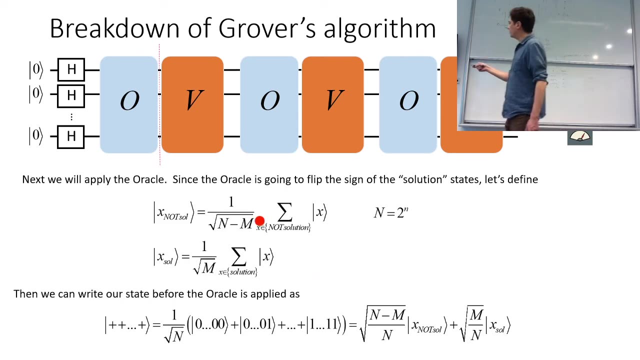 I already wrote that. but let's go through the algorithm step by step. So after the first set of gates, you just create the superposition state. Okay, I've already said that And this. I've drawn a red line here. 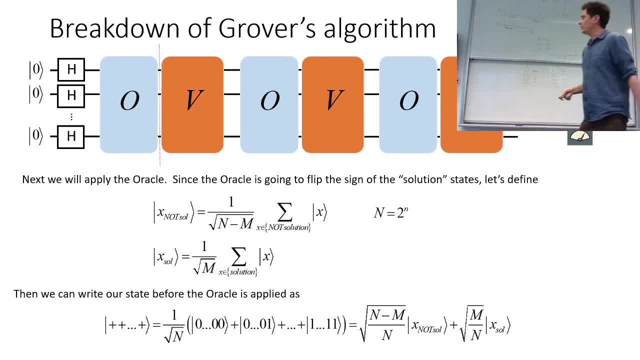 so you might be able to see. that's where we're up to in the circuit. So next we apply the oracle, and the oracle is going to flip. the sign of the solution states, And so what I've got here is something a little bit more general. 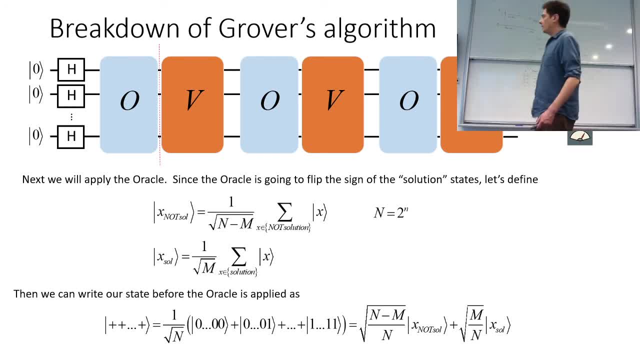 than what I was saying just here, Because you know there might be more than one solution, So it might be that. so remember n this. n here is the size of the space, but m is the number of solutions. Okay, 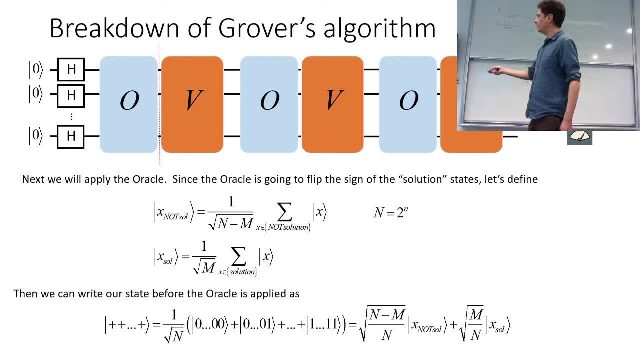 So if there's more than one solution, then this algorithm actually finds sort of all of them as well. Well, you know in a sense, Okay, so we're going to define these two things. So, basically, these are just all the states. 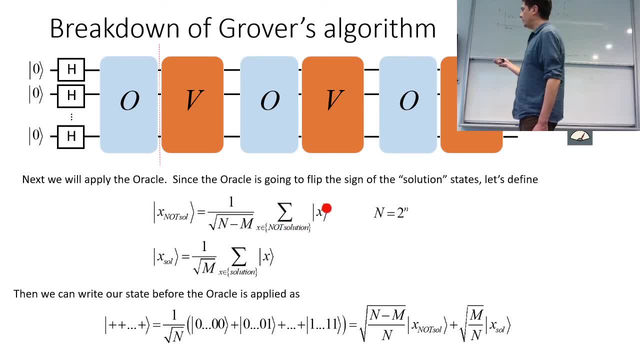 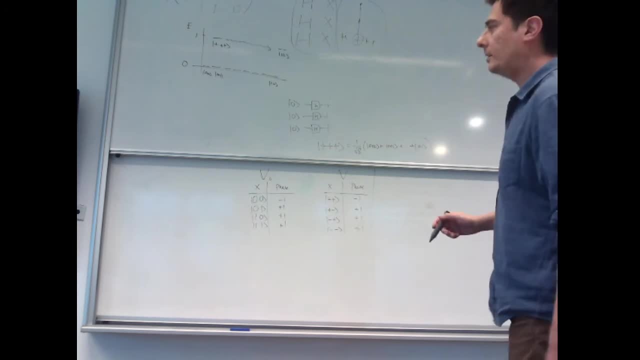 that are not the solution. Some of all of the states are not the solution. These are all the states that are the solution. So just to give you an explicit example, so if, basically, if, we're doing Danny's case, then x, x, naught solution. 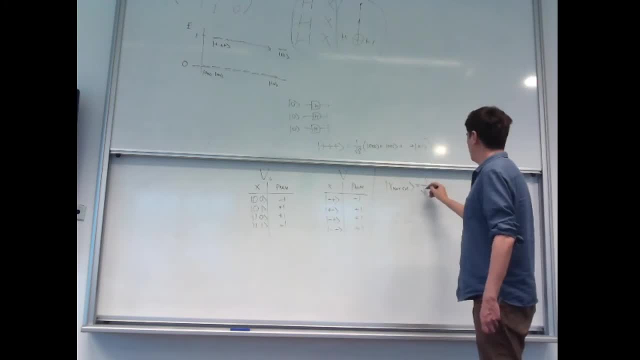 would be equal to square root of seven, zero, zero, zero, all the way up to one one zero and x solution. that would be just one, one one. Okay, There's more than one solution, like, say, if there's two solutions. 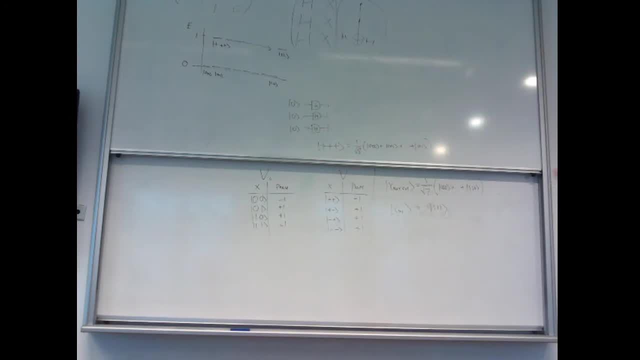 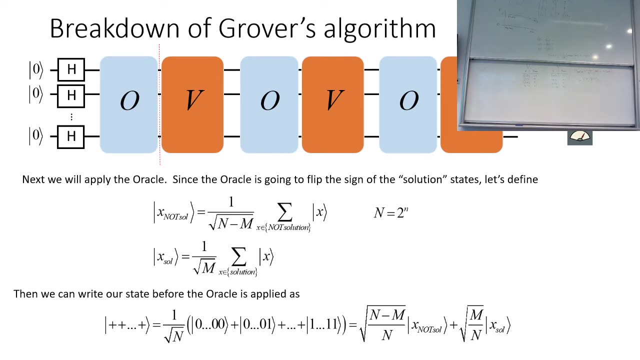 here, then we need to normalize it. So it's one over square root of two And this is seven, because obviously there's seven states and we need to normalize it. Okay, So then we can write this initial state actually in terms of these two things. 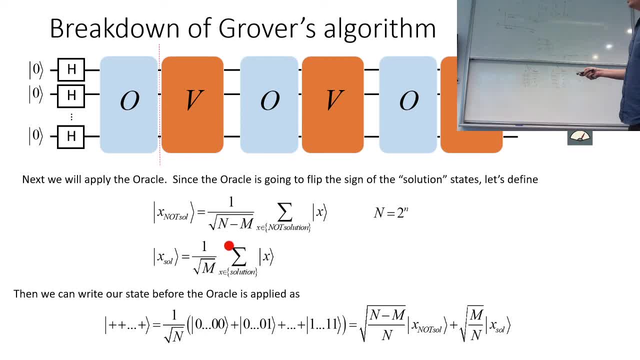 And it turns out that this will be the best way to write it. So, even though it looks a little bit more complicated, we can write it like this, And so, in this case, the initial plus state, and because we've got this: 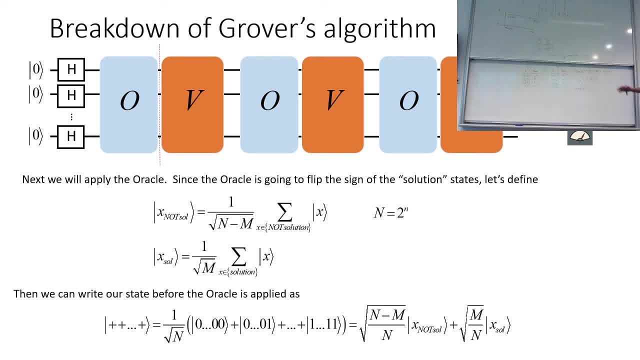 you know square root of seven thing. here we need to multiply by the original, like appropriate factors, in order to have just this equal superposition. So the initial state in terms of these two vectors, you would write that as square root of seven. 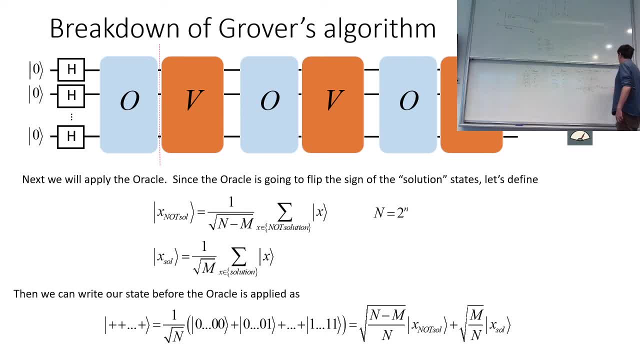 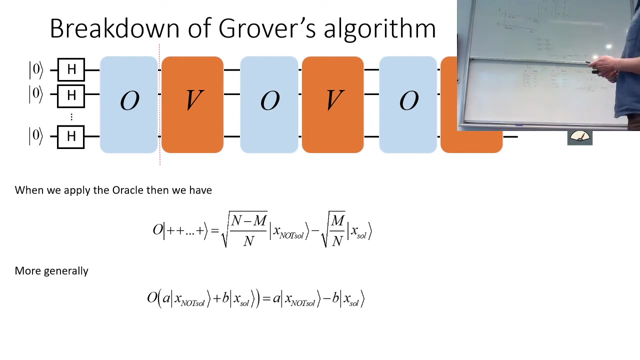 x, not sol, and then this is x- sol, And then, after we've multiplied by the right coefficients, we need to divide by the overall normalization. So that's just that thing there. Okay, Then we're going to apply the oracle. And so, now that we've written it in this way, 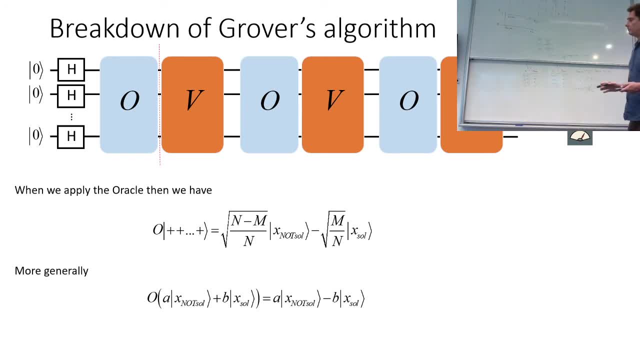 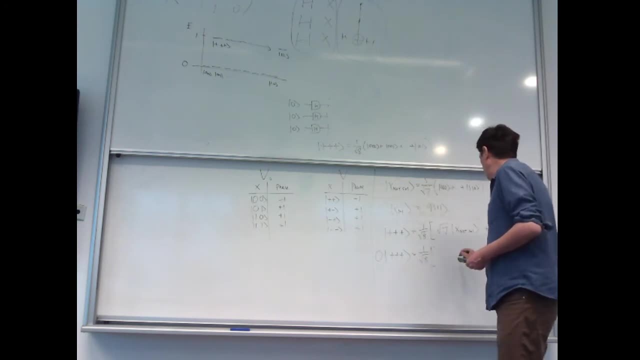 it's actually easy because, well, particularly this step is easy because we know that the oracle just flips the sign of this one. So oracle times plus plus plus is going to be just same thing, not sol minus x. Okay, So we just flip the sign of the solution part. 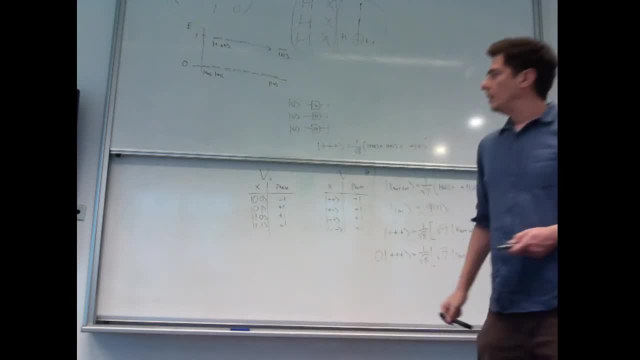 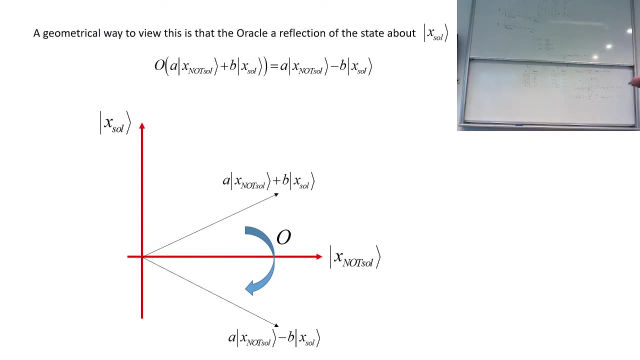 Slightly better thing, Okay, Okay, All right. And then now let's do the. oh yes, that's right. So there's a great way of understanding what this operation does geometrically. Okay, So let's. and it turns out that in Grove's algorithm, 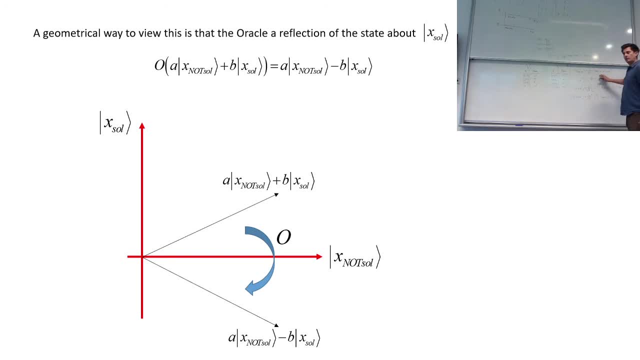 you can write everything in terms of these two states that we just defined. So the whole thing evolves actually in this two-dimensional kind of subspace. Obviously, the larger Hilbert space or the larger space is much bigger, right? So it's three qubits. 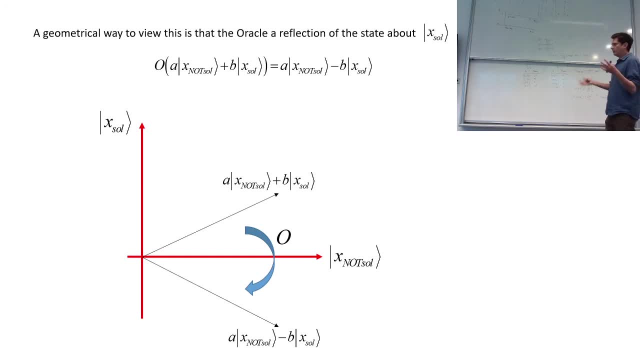 It's eight dimensional. Normally, you know, the algorithm wouldn't be moving in this eight-dimensional space, but actually for Grover it turns out that it's entirely in this two-dimensional subspace, So we can actually just draw it quite easily. 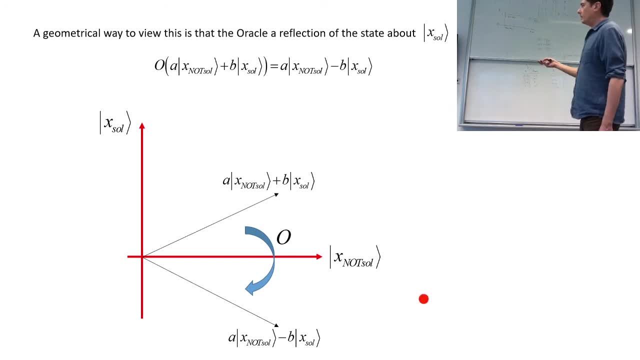 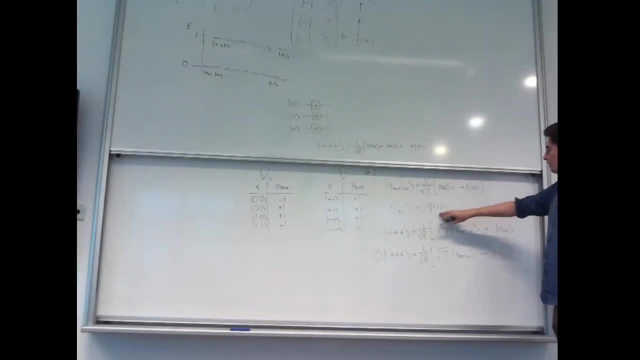 on the plot here. So these things are orthogonal, and you can tell they're orthogonal because there's no common states, right? So this is the solution one and this is the not solution one. So obviously one one one does not appear here. 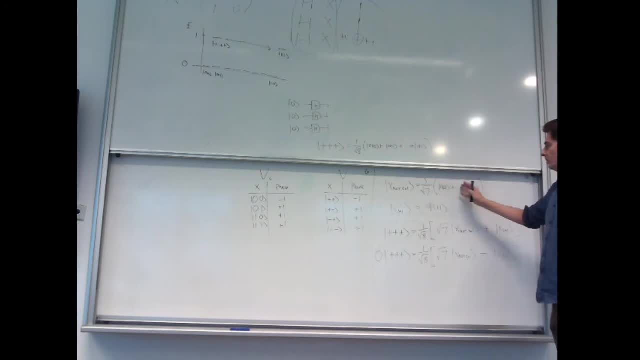 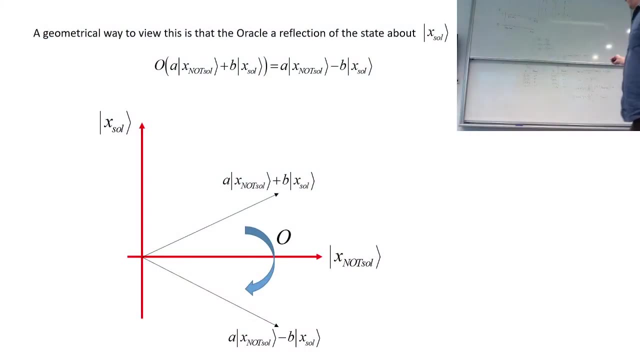 and all these states do not appear here. So if you take the inner product of these two, it'll be zero. So they're orthogonal and we've normalized them properly. So those are our axes that we're going to work with And let's just talk generally. 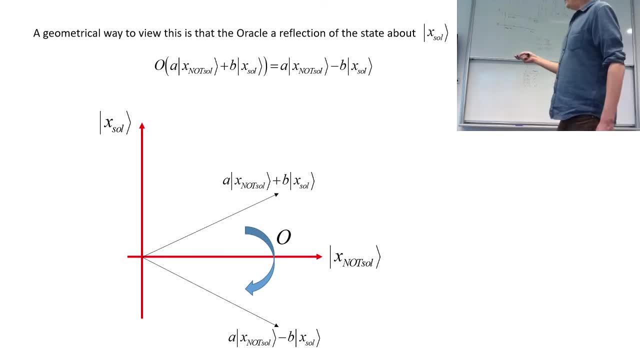 of what this oracle does. So if we take some state which is some superposition of these two basis states and we apply this oracle, so if we start with the state AB- it's pointing that way- then this flips this sign right. 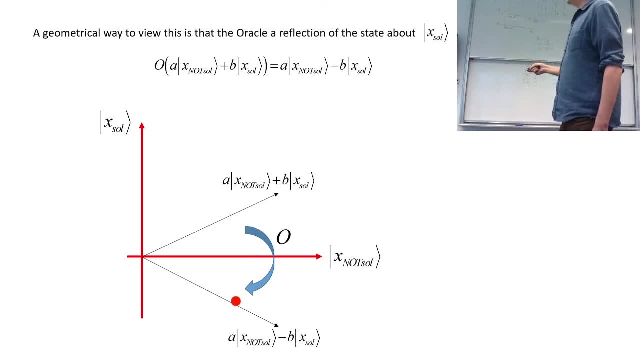 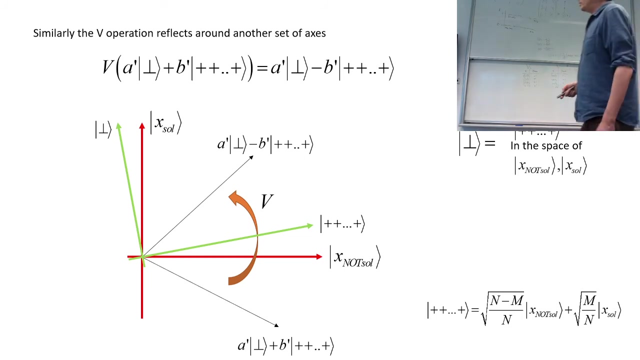 So obviously what that does is to reflect it, along with the axis being this not-sol, So we can use that to kind of visualize what is happening to our state. So, Oh, okay, Sorry, that's not what I'm explaining here. 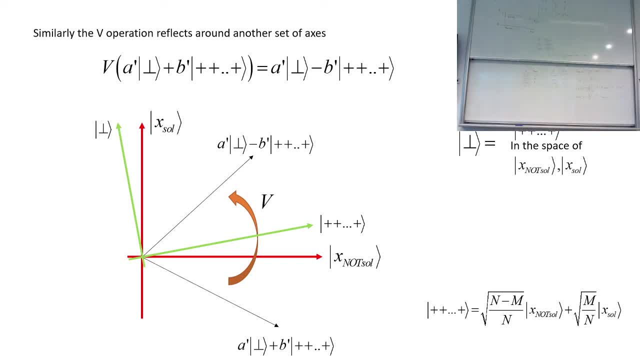 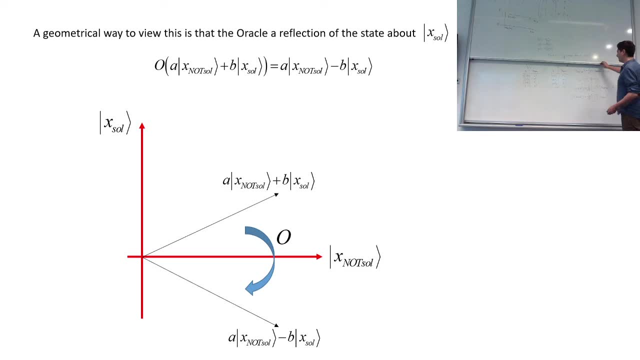 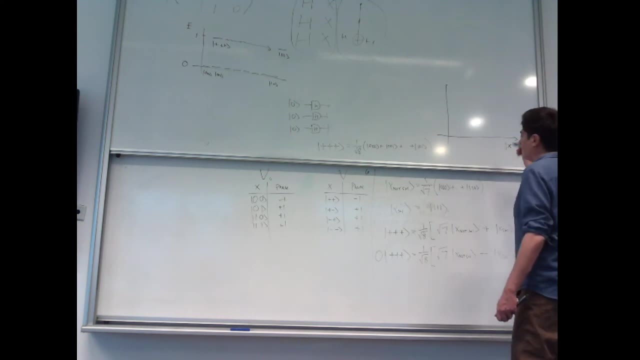 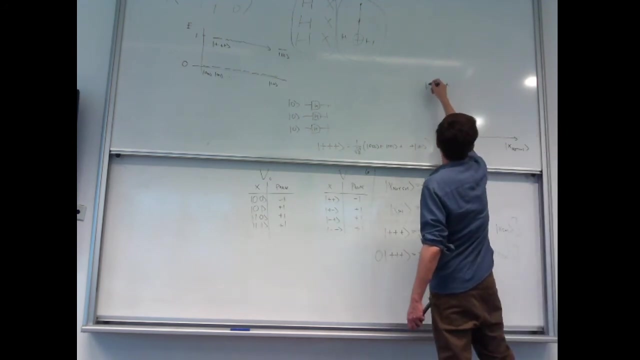 What? Okay so, So let's just sort of sketch what's happening to our state here first. Okay so, So let's sketch this. So this is not-sol, This is not-sol And this one is the solution. yeah, 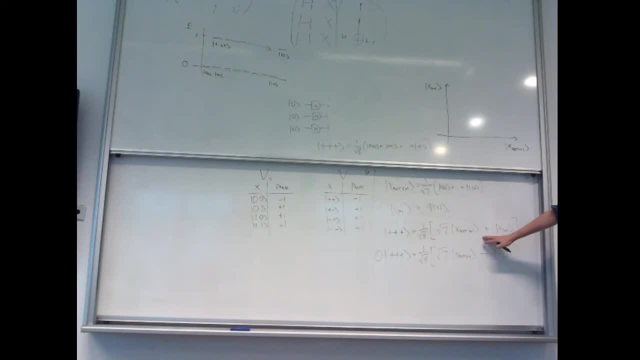 Okay, and our initial state looks like this. And keep in mind, there's no complex numbers or anything, so it's just all real numbers. so we can just literally kind of plot it on this graph. So for example here: 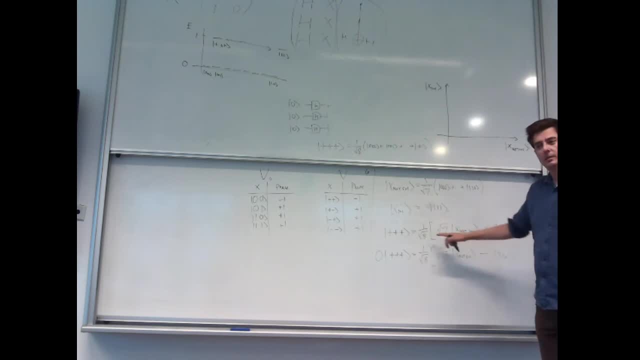 this coefficient here is root 7 on 8.. You know it's quite close to 1.. This coefficient here is 1 over root 8, so it's kind of much smaller than this one, But it's not 0.. 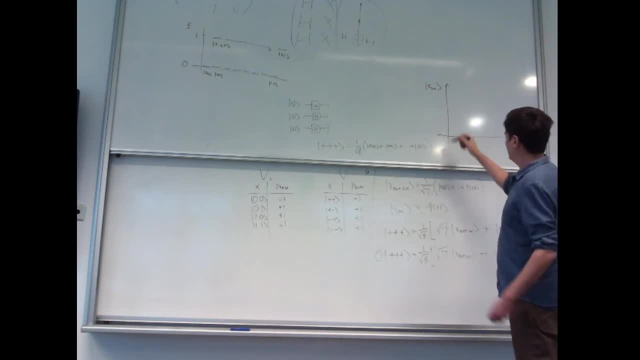 Okay, so if we plot it along on this graph, then roughly speaking, this will look like this: So this is actually what the Grover's algorithm initially starts with, And then one application of the oracle. what it does is: And so this in this triangle: 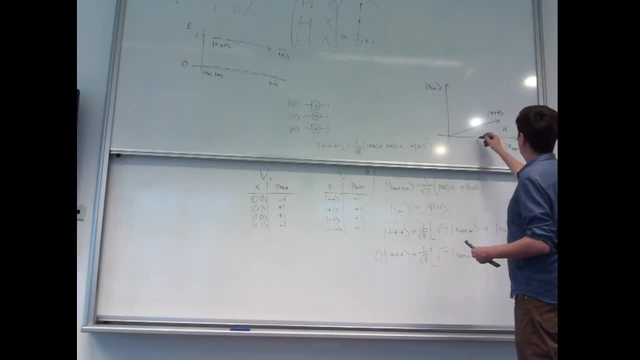 just to sort of got everything clear. this is root 7, okay, And then one application of the oracle will bring it down below this axis here. Okay, so that's that's where we're up to at the moment. We've applied the oracle once. 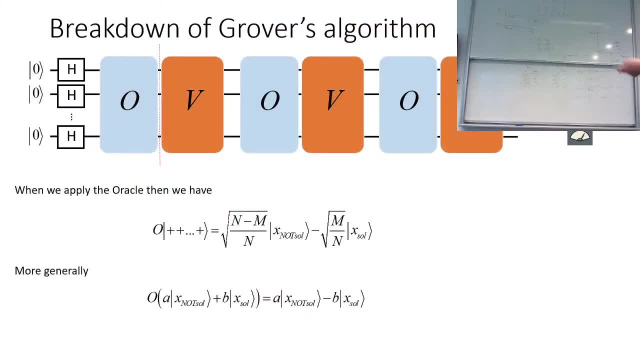 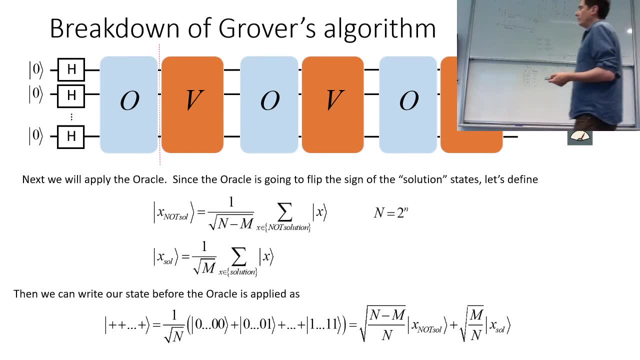 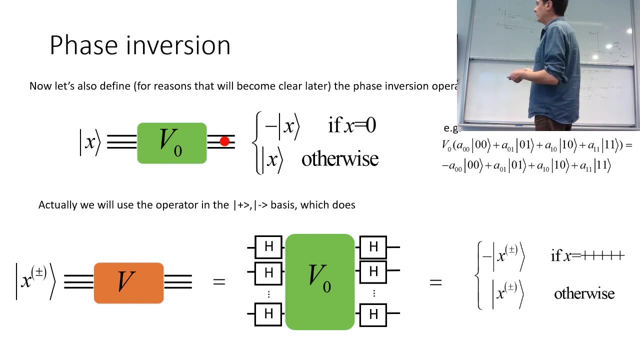 Okay, now let's think of what this V is going to do. Right, And if you remember, V V is actually, you know, kind of something very similar to, very similar to the oracle, except what it does is to apply. 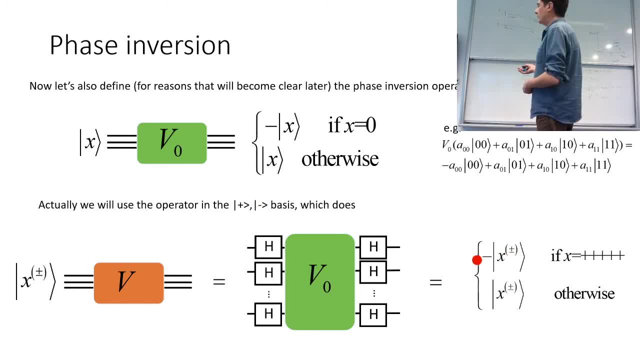 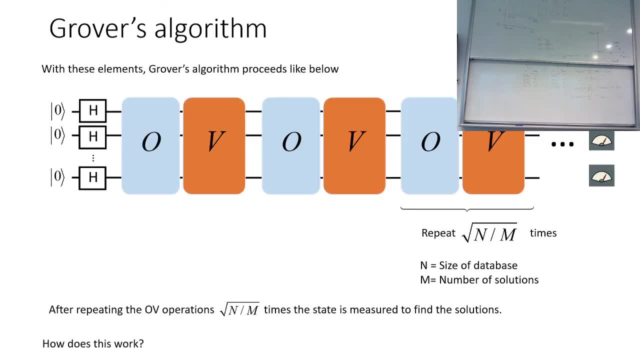 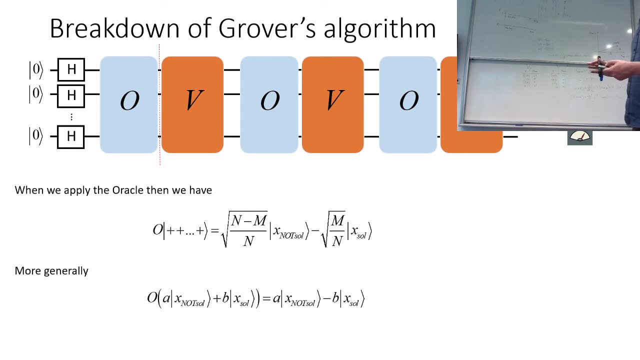 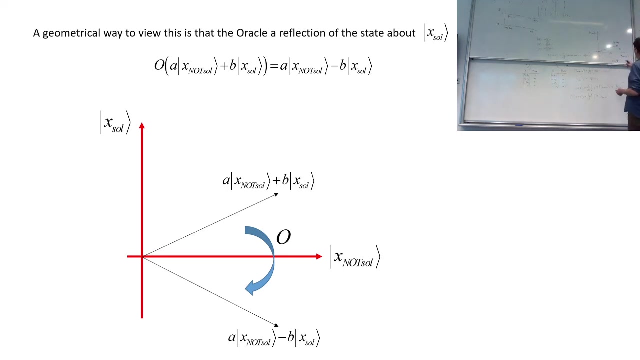 a minus sign on this plus state, And I don't want to show you the calculation because it's just sort of tedious, It's not so, It's not very interesting And it's kind of obvious from this result that So the oracle is something that 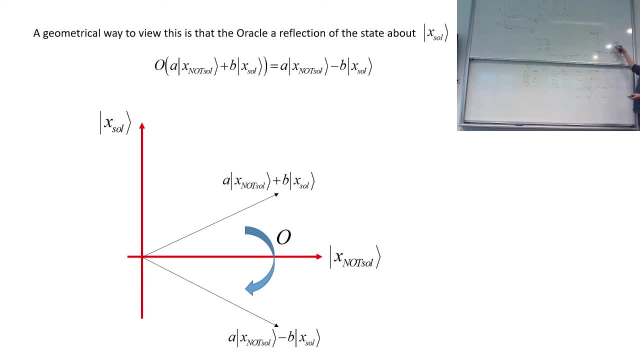 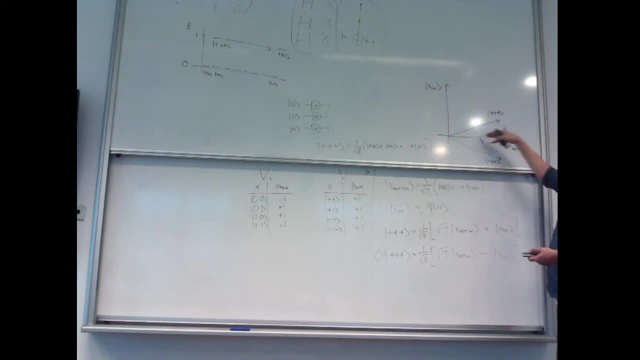 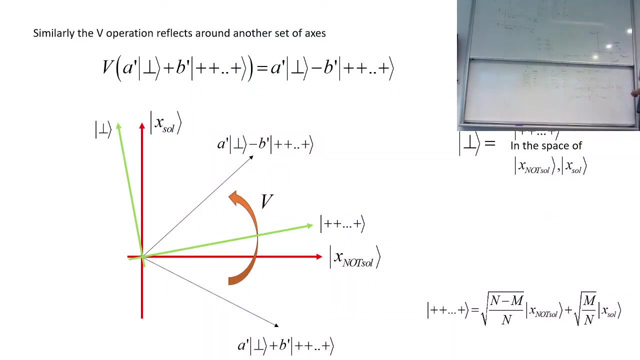 flips the sign on the on the solutions, right, And basically what that does is to reflect it around this axis. that was the not solution. What the V operator should do is actually to again reflect it around actually this axis, which is this plus. 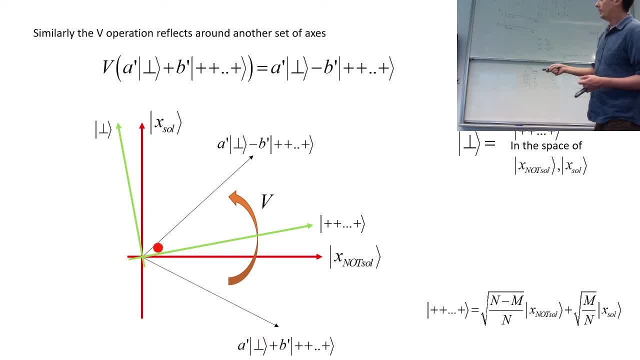 So it will For any state over here. it will then reflect it and make it another state, which is on this positive side, because, Well, okay, so here Maybe I should have said minus V dash here and plus V dash to be. 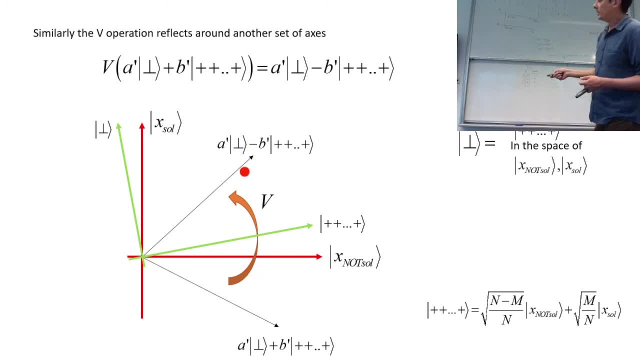 a little bit clearer. but But basically what this does is to reflect the state around this plus state, instead of the not solved state. And this is basically because the V and the oracle are kind of very similar operators. They're both operators that just. 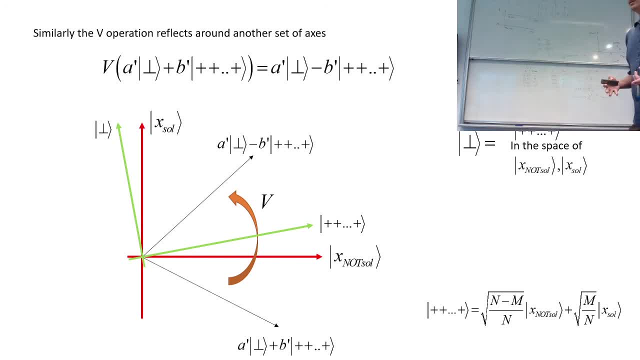 change the sign of one particular state. In the case of the oracle, it changes the state of this solution state. In the case of this V operator, it changes the sign of this plus state. So So you know, that's. 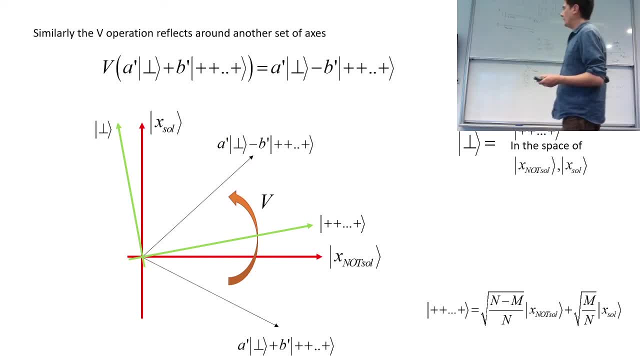 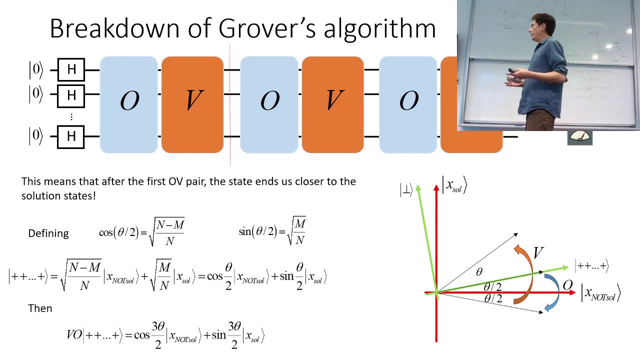 That's the action of this V. So, essentially, what you can then do is to purely from the geometry in this sort of two-dimensional space. you can just think of the multiple reflections that this initial state is going to do. So our initial state: 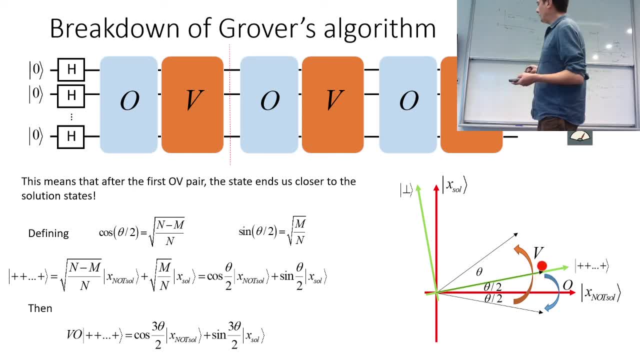 This was our initial state And firstly it gets reflected around this not solved axis And then- So that was the oracle operation- And then It will get reflected now around this plus state axis. So now this is going to go up here. 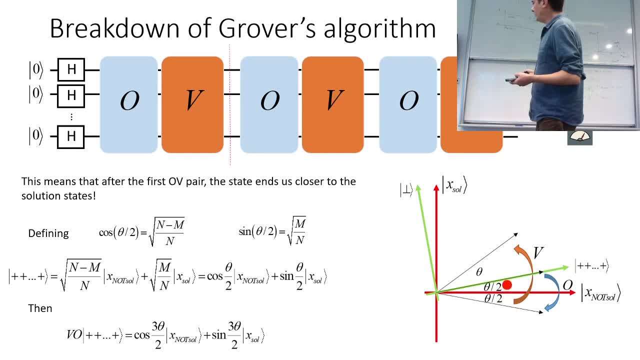 And now notice that the angle between this kind of green line and this other line going down is actually theta right, And when we do the reflection, this will end up pointing in this direction, With theta being this angle between the green axis and this arrow here. 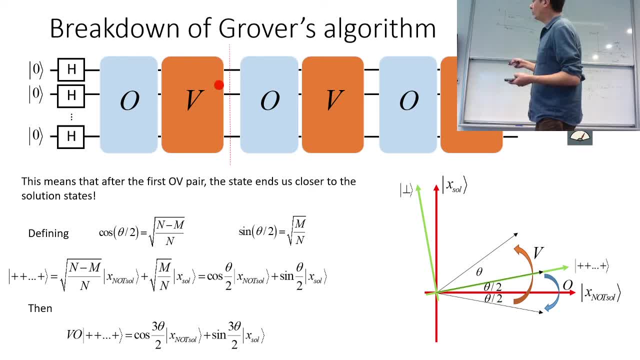 So if you think about what happens after one iteration of OV, it will sort of go down by a degree of theta- Theta is defined somewhere over here- And then it will go up by 2 theta. So if it goes sort of, if it's rotating- 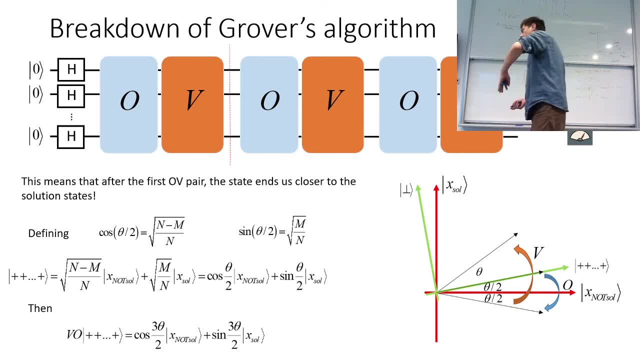 clockwise by theta, then anti-clockwise by 2 theta. of course, eventually it will end up closer to this red axis. So it's purely based on sort of geometry. But this is sort of the easiest way to kind of understand or kind of. 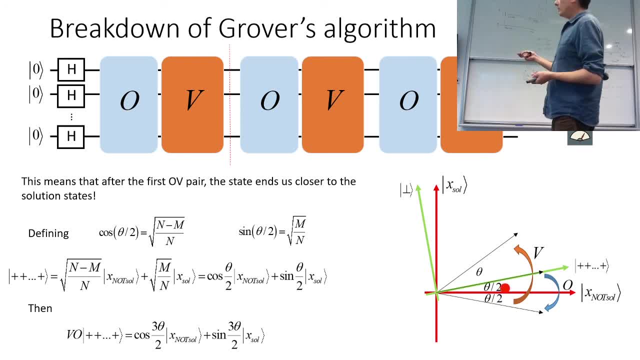 prove why this works. Okay, so, regarding these equations here, this is just the definition of what this angle here is. So in this particular example, the angle was- you know, just look at this triangle. So whatever that angle is is what theta is all. rather, this is theta over 2,. 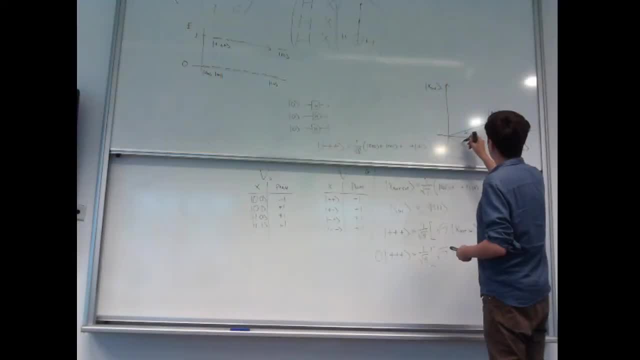 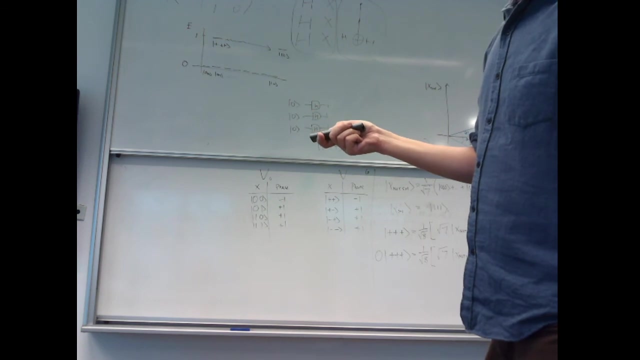 right theta over 2.. So that these factors just define that triangle according to just high school trigonometry. Um and then, uh, all I'm saying here this is like this initial state, plus just written in terms of cosine sine, because 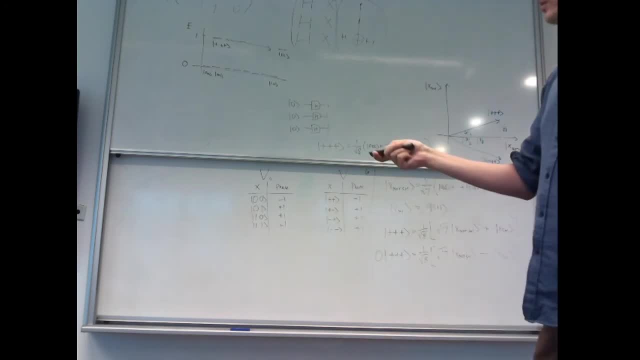 we just defined theta here, So that's just that. And we know that after one oracle then that sine flips, But then after application of the v it will go up by another 2 theta. So eventually the angle here is going to be: 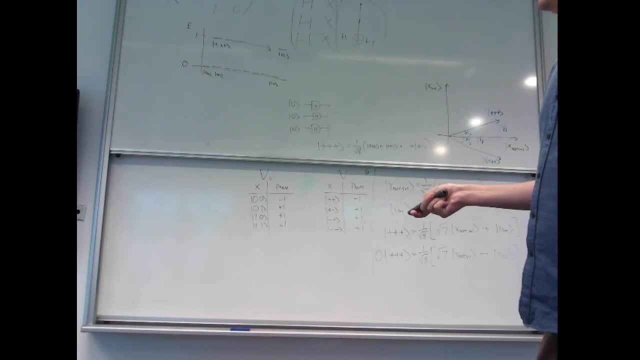 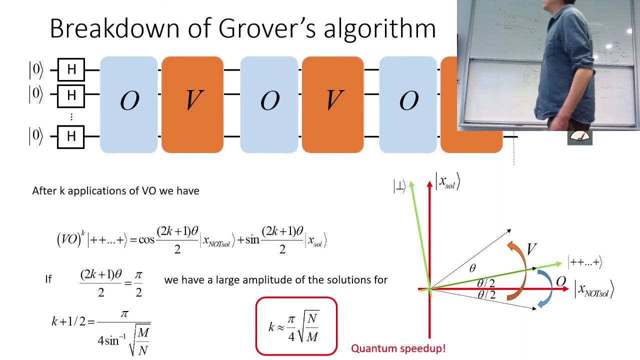 3 theta over 2.. So initially the angle is theta over 2. And then, after the v-o operation, will be 3 theta over 2.. Just looking at this diagram, Okay, and so basically the pattern then repeats itself, because 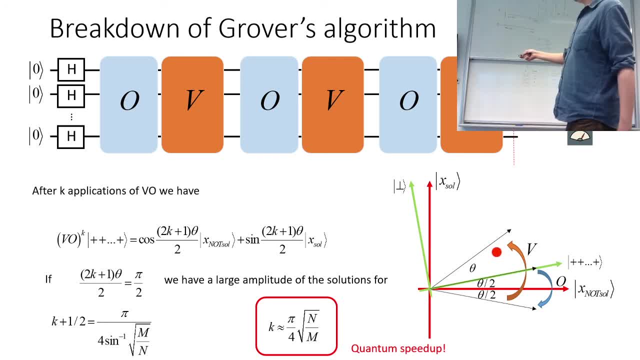 this is just. you can just work it out according to what the combination of these two reflections are, And so essentially, with every pair of this O-v, it basically moves closer to the solution state by an angle, theta. So by repeating this some appropriate number of times, 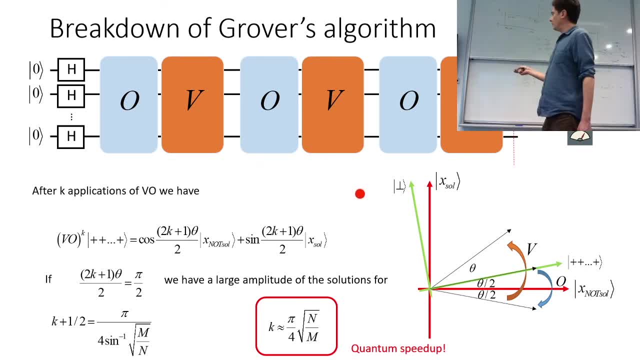 it will get quite close to this solution state, And so this is what I was saying at the end of Danny's talk- that maybe the reason why it doesn't get exactly to 100% is because these steps are kind of discrete. So this theta is: 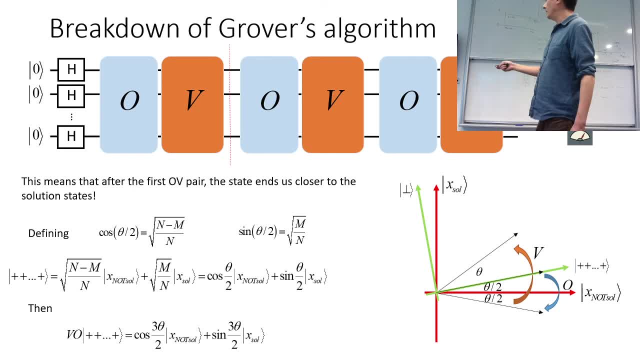 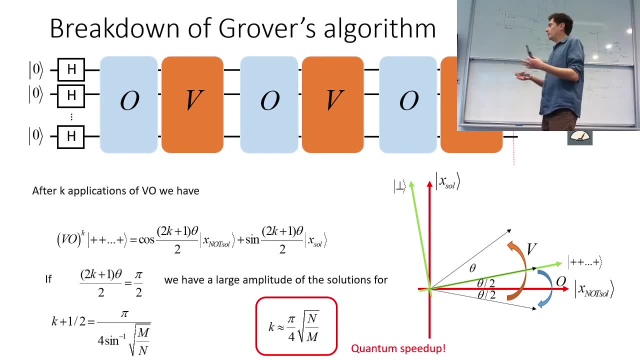 whatever you work out according to here, So you just work out that angle. So if that angle isn't a multiple, if you don't do a multiple, if it's an angle such that it's not like it doesn't get exactly, pointing along this solution. 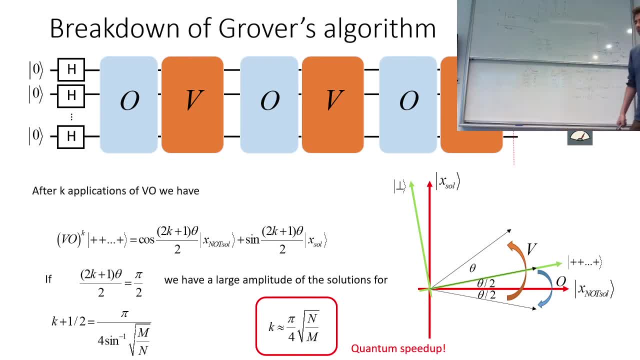 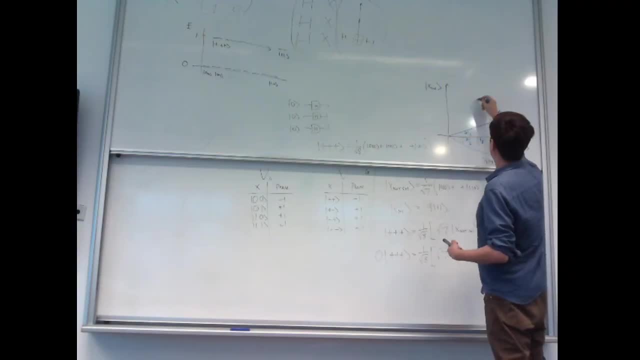 direction. then you won't get 100% probability or 100% in this solution state. You'll get it kind of closer like so maybe after one iteration it'll look like here: so this is theta, Two iterations. well, according to this, it might not point exactly. 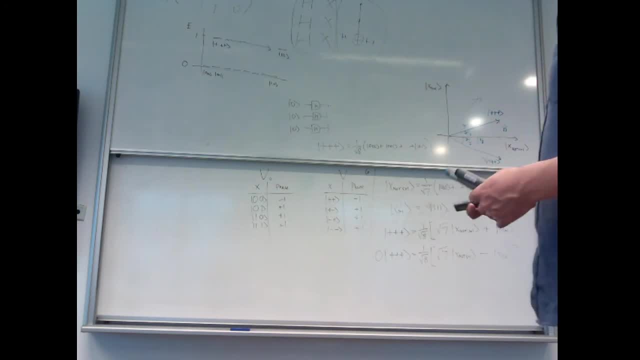 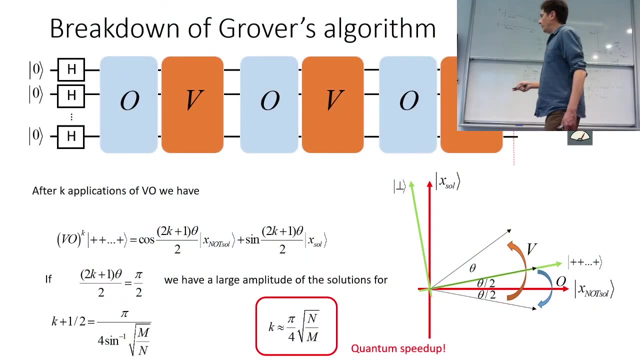 along the axis. Okay, and then now here comes the most important part, which is: so, how many times do you need to apply this? Okay, and because we know this angle, so basically, if after k applications of this v o, essentially we want this thing here to be 1 right, 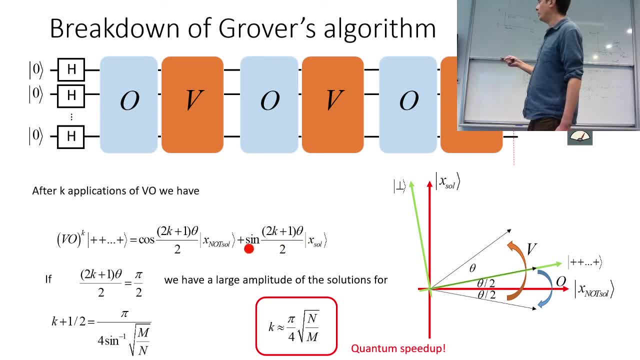 Well, we want that angle to be pi over 2. then sine is 1 and cosine is 0. We obviously want the state to be in the solution and not in the not solution. So okay, set that to pi over 2, simple calculation and work out. 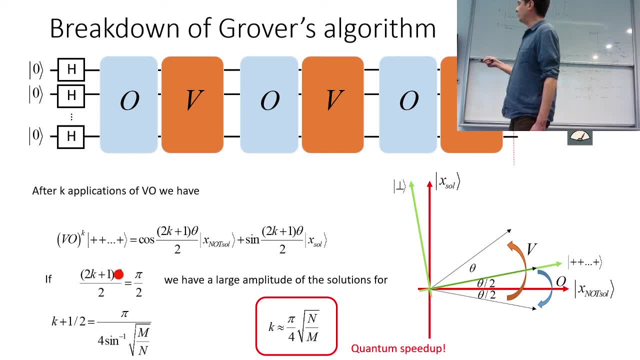 what k is. so if you just rearrange this thing according to the definitions, it's that. and just to make the formula a little bit nicer looking, let's assume that n is quite big and m is much smaller than n. then this inverse sine is approximately linear. 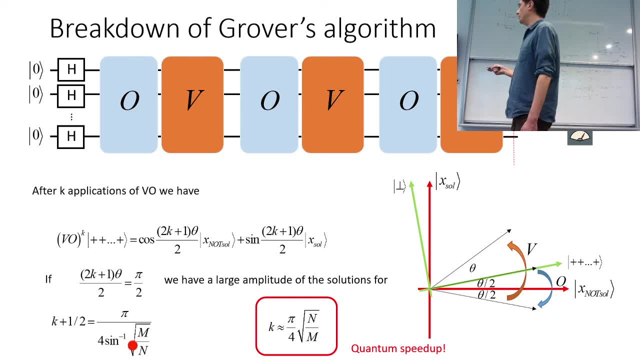 so this sine of square root of m over n is approximately square root of m over n, and then just forget about the factor of a half, because let's say that's small too, it's equal to that, and so the key thing here is that this scales. 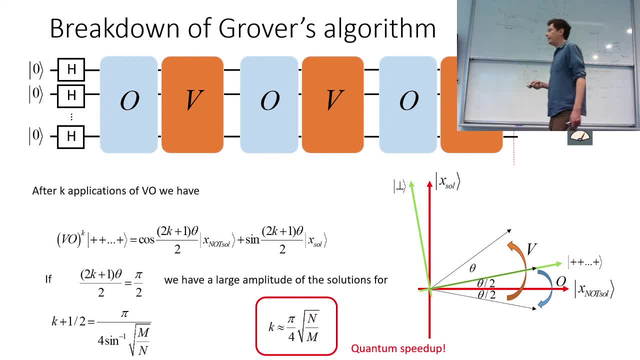 as the square root of n and classically you need to search through the database, like basically almost all the database elements. even if you're doing a random search, if there's a hundred elements, roughly speaking you need to look a hundred times before you get the answer. 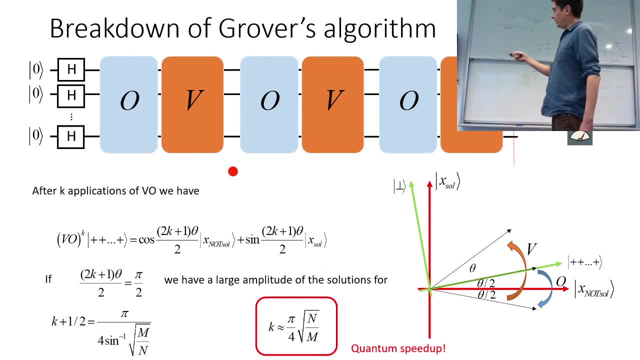 that you're looking for. but here, if we count how many times we are doing this ov combination, you only need a square root of n times. so if you had a hundred elements, classically take something like a hundred tries out with quantum you can do it with. 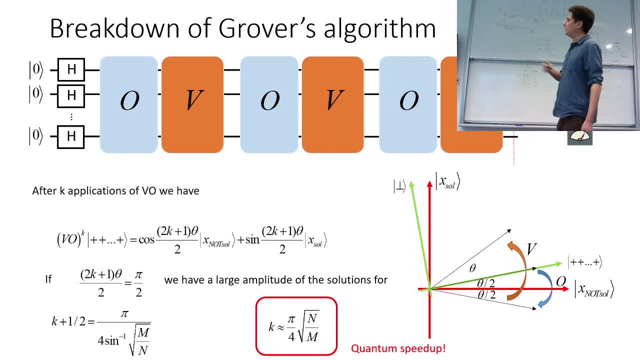 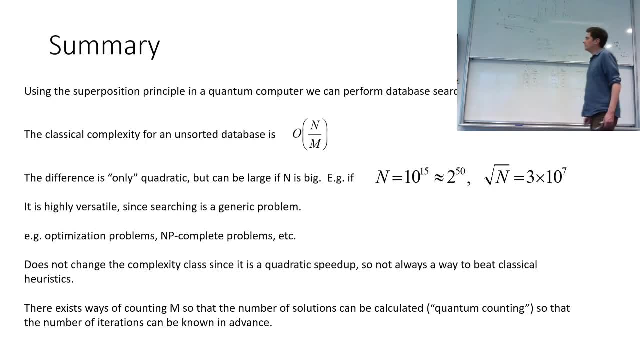 ten, ten iterations of Grover. if n is bigger then this gets even more kind of powerful. so even though this is, you know, inverted commas, only quadratic speedup compared to classical. but if n is big then this can make a big difference. so if we're talking like n is, 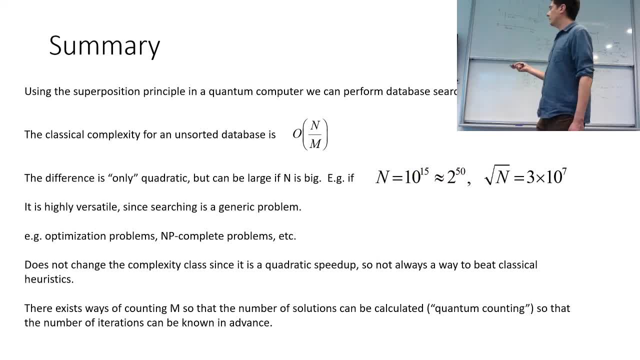 two to the fifty. why don't I choose two to the fifty? probably because maybe this is like the largest sized quantum computers that are available today, so that's just today's technology. so they're actually not quite good enough to do this algorithm with fifty qubits. 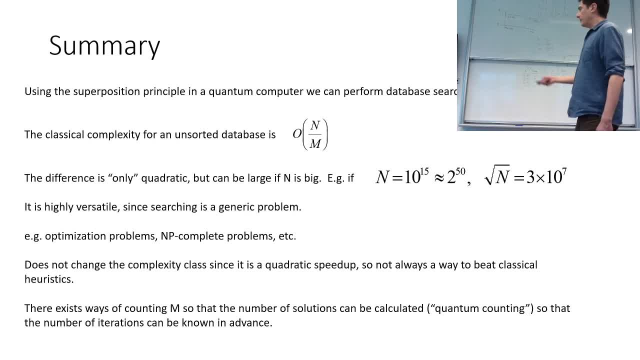 I think. but. but even if they were, there would be quite a big speedup, because two to the fifty is quite a big number, ten to the fifteen, but square root of n is only ten to the seven, and you know basically anything like you know like computers. 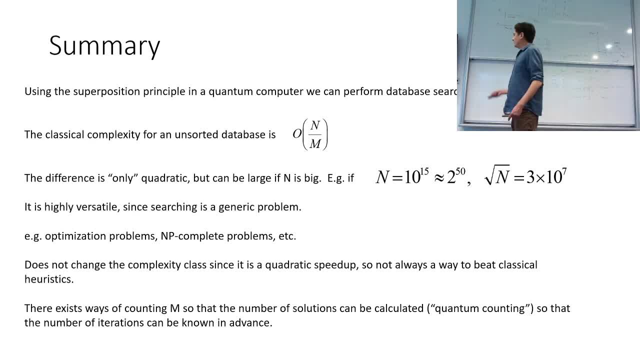 or like gigabytes, terabytes, this kind of thing. so ten to the seven is is actually nothing with in terms of today's sort of classical, quantum, classical computing technology, but ten to the fifteen. once you get to things like this, even the best super computers in the world. 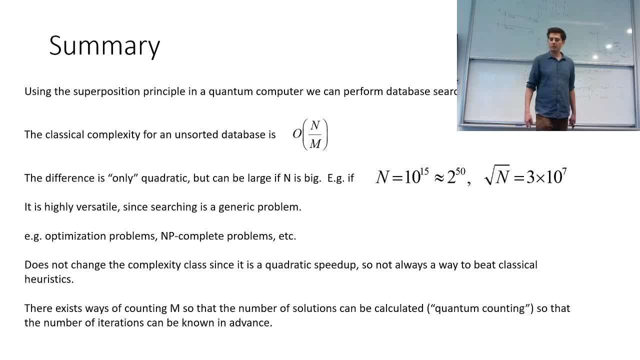 find it difficult to handle that, like just to store that amount of data or, you know, just have that in the memory of a program or anything like this. it's kind of very goes beyond typical capabilities. another factor is that this thing is it's very versatile. so 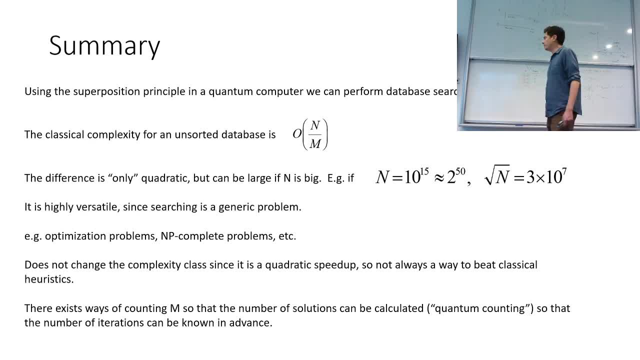 searching is a very generic kind of problem. it comes up all kinds of places, so it's very applicable actually. so you can apply it to optimization problems and so forth. um, now I don't know if you guys are um, do you know this? P equals NP. I've read it. 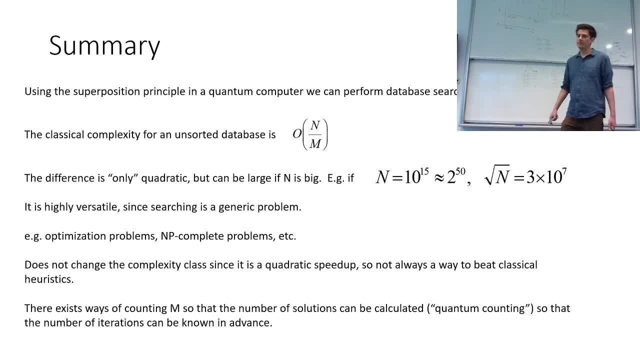 in the aspect, but I don't actually know how it works, right, yeah, so, yeah. so this is a famous kind of uh unproven well conjecture. in computer science there's um classes of algorithms, which are some types of algorithms are very efficient. they can be solved. 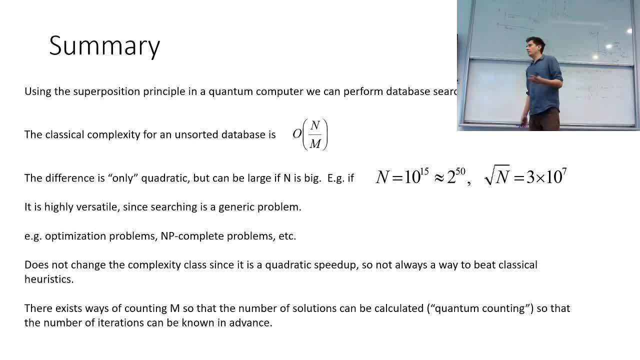 in polynomial time, and some types of algorithms are very difficult in the sense that the time to do the algorithm scales exponentially and so, um, it appears that there are kind of two different classes of algorithms. so there are these ones which just scale much more, you know like exponentially. 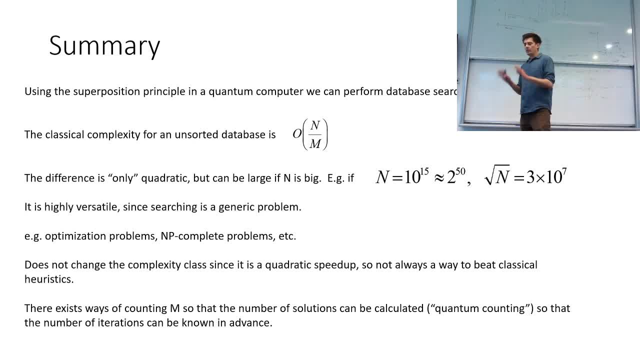 and there are those which are somehow easy. so the polynomial ones are called P and then exponential ones generally are in this NP class and um. this P equals NP problem is um. well, it's widely believed that these are different classes, like basically this: um, these are not the same, but 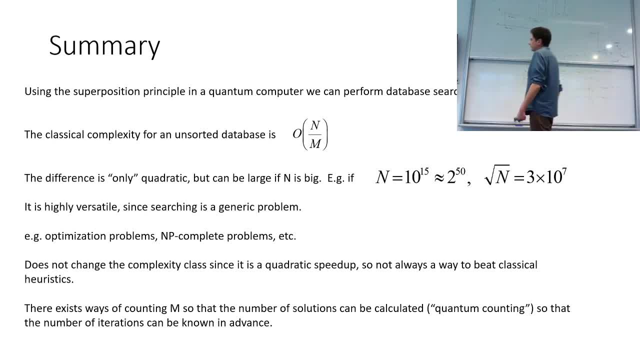 um, um, but yeah. so basically it's a kind of conjecture to say that, um, that basically, you know, NP class is a larger set of problems than P, so P should be kind of a subset of NP. this is sort of the conjecture, but um, but there's no real. 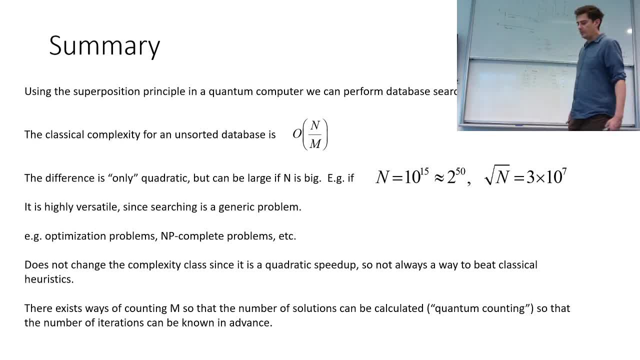 proof for it, right? so, um, nobody can prove it, but that's what is sort of observed. so, um, um, one point is: you know, could this be used to help solve such exponentially scaling problems? so the answer is basically still no, because you know if you have some problem. 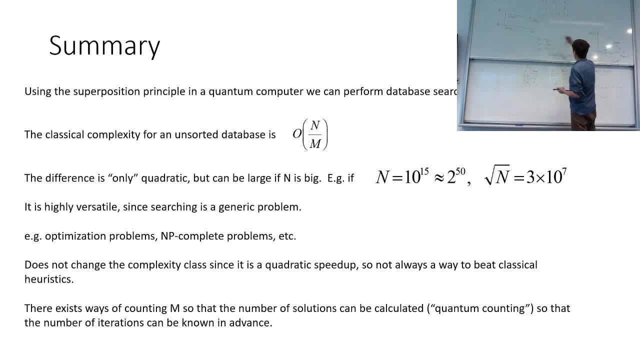 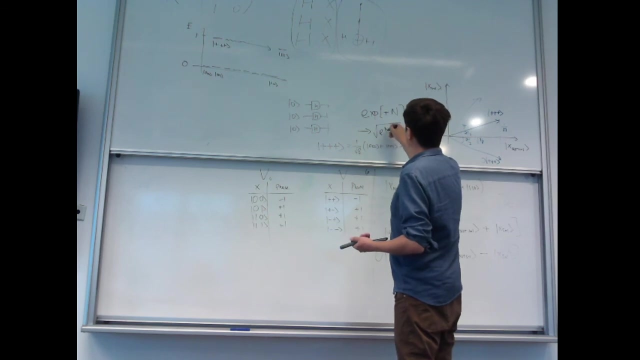 that sort of. you know scales as exponential, so say you know the the time, say complexity of an algorithm. you know scales, suppose, like exponential n, right and uh. if you apply Grover's algorithm then essentially what happens is that it becomes square root of the exponential of n. 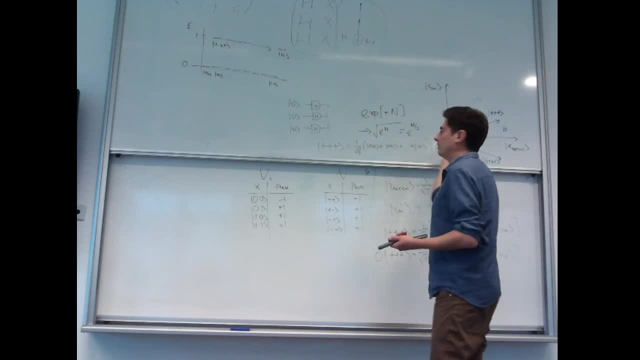 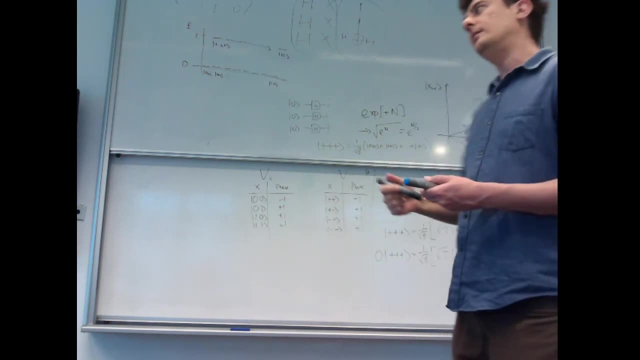 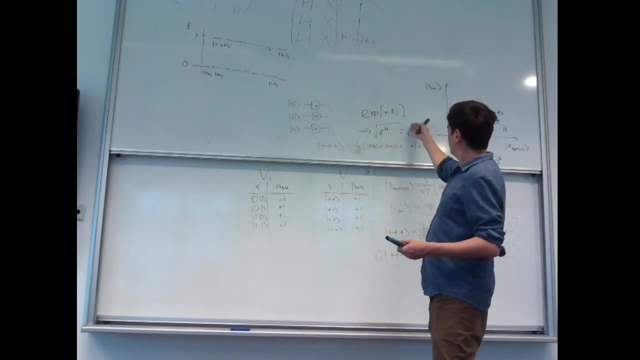 but actually that's still exponential. so because square root of n is still exponential, so it doesn't really change the complexity of the algorithm. um, of course that helps quite a lot because it makes it n over 2, not n, right, but the thing is, is that, uh, there's lots of 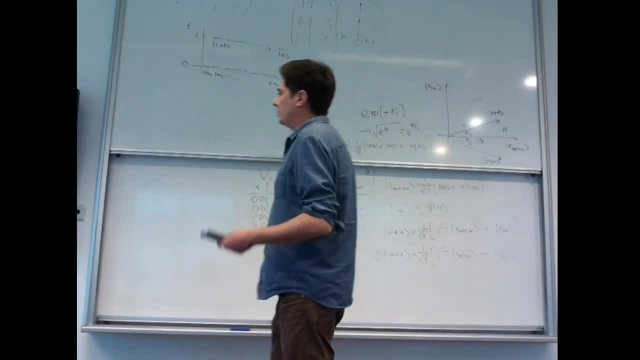 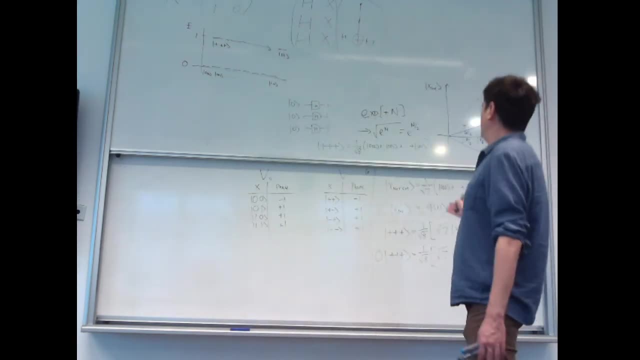 different algorithms that people have come up with to sort of um, you know so, even if a problem is exponential to to you know to have exponentials that scale like relatively well, right. so essentially, even if you applied Grover, this would have to beat whatever you know some other. 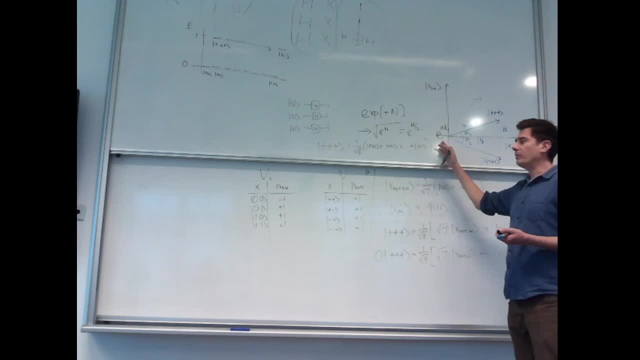 you know potentially exponentially scaling algorithm, and essentially what we're competing here is this sort of factor in front of the n, so you know. so here we might get a factor of you know a half, but maybe with classical, you know, with a clever algorithm you can still get you know some. 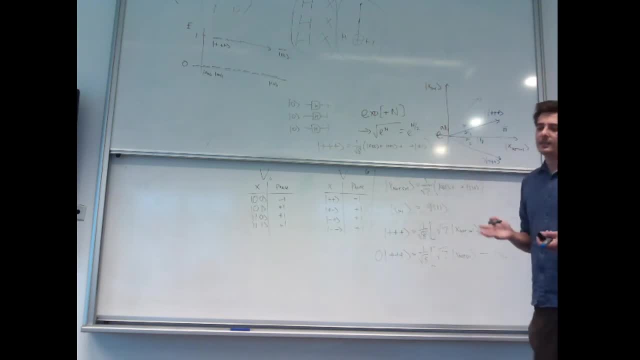 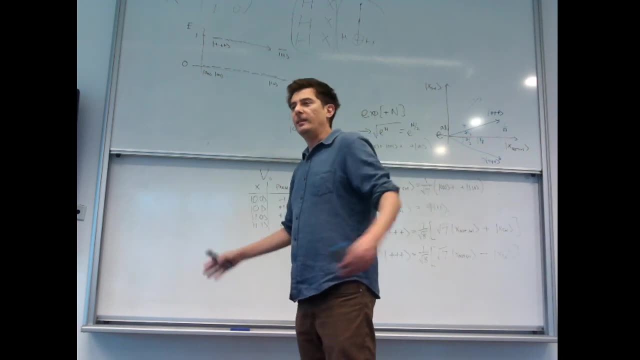 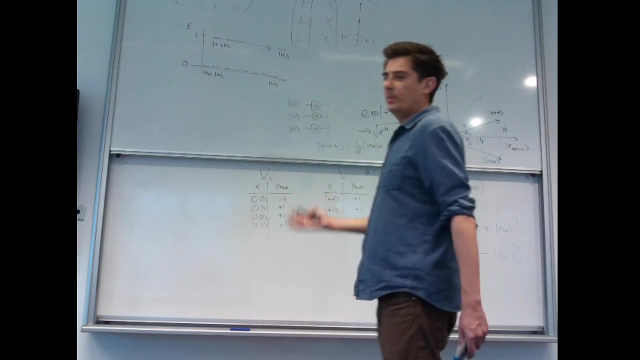 similar factor, which is also maybe like a half. so it doesn't. this doesn't necessarily beat any classical. you know this is not a recipe to beat any classical algorithm, uh, but it could be used. so it really depends upon the particular algorithm and maybe this could be used. 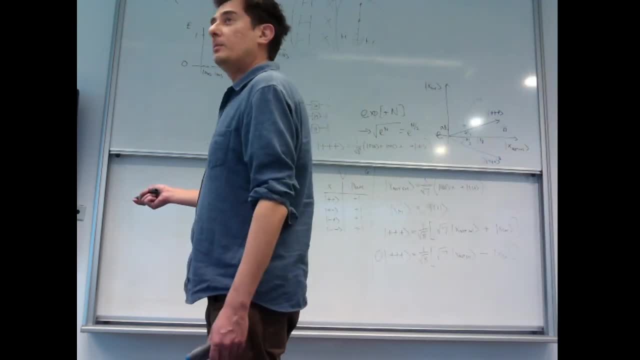 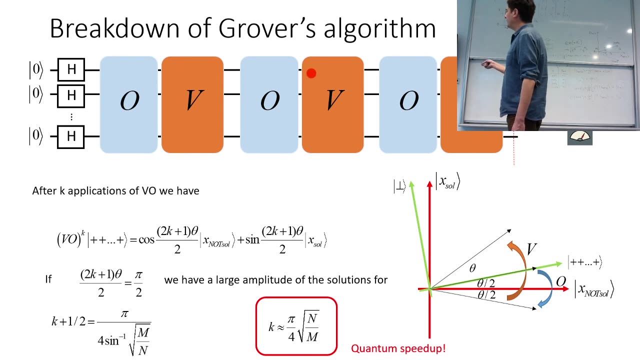 um, yes, and I won't go into sort of time, but uh, you might be wondering: uh, okay, that's you know. so we have to apply this some number of times. how do we know what number of times to apply it to without doing it many times? actually, there are. 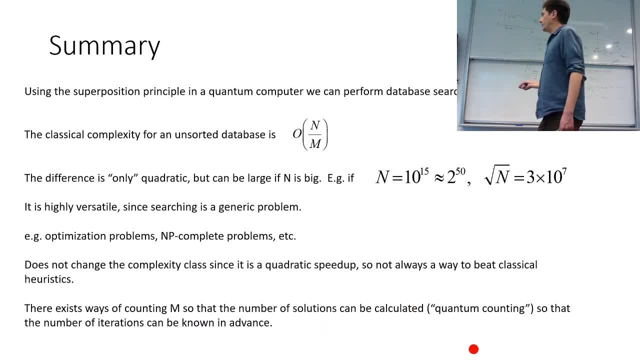 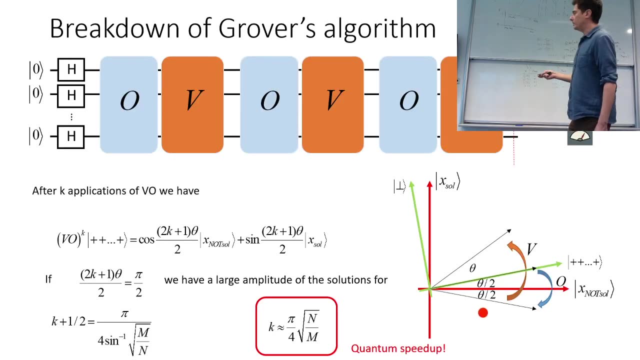 some algorithms out there that are known to figure this out. so there's this so called quantum counting algorithm, which, well, you can look up in the textbook Nielsen and Chuang. so they do exist, so that even that is could be calculated with another algorithm, or you could do it.